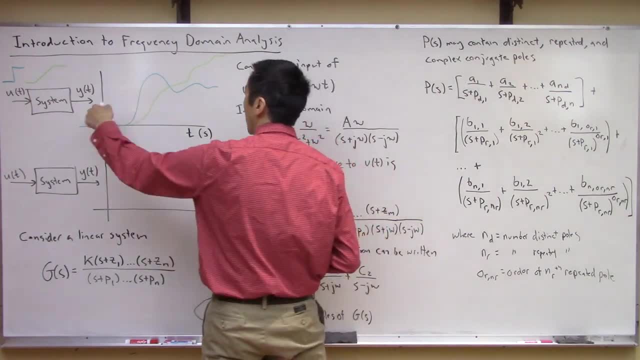 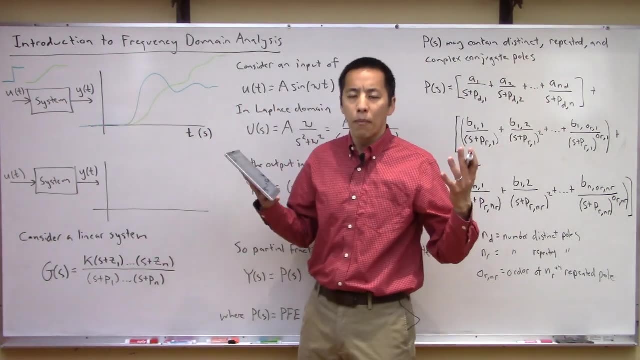 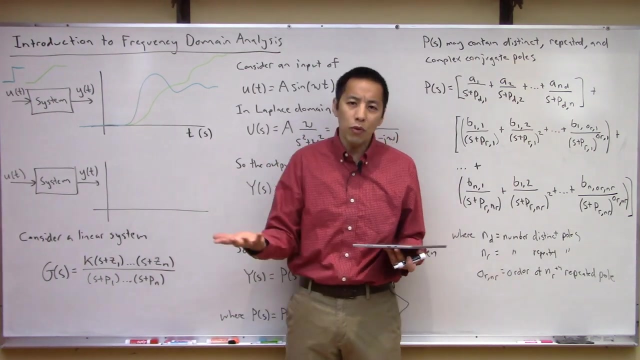 seconds or something like that is the sort of independent variable. and the dependent variable is whatever It's the actual response, it's the some internal signal, it's some part of the system that responds to this input, right? So that's the idea with time domain analysis. What is frequency? domain analysis, Frequency. 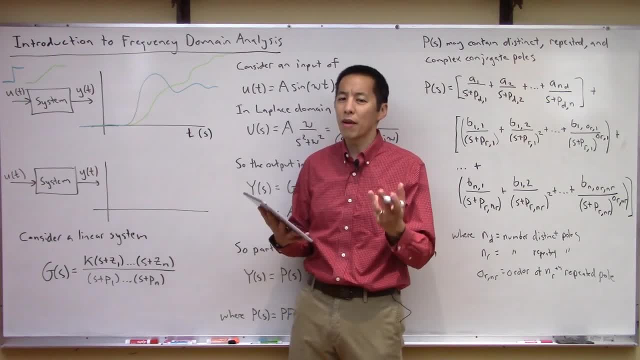 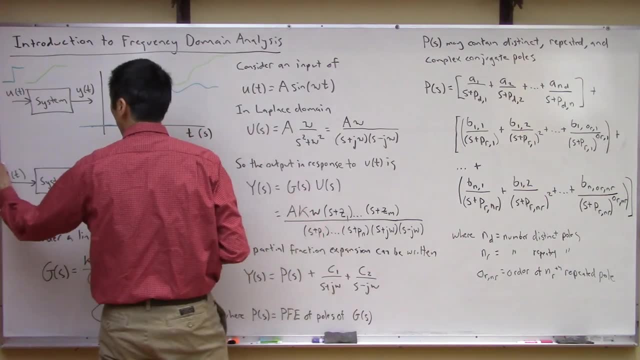 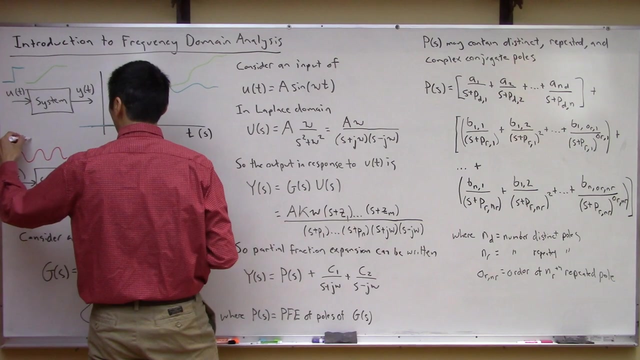 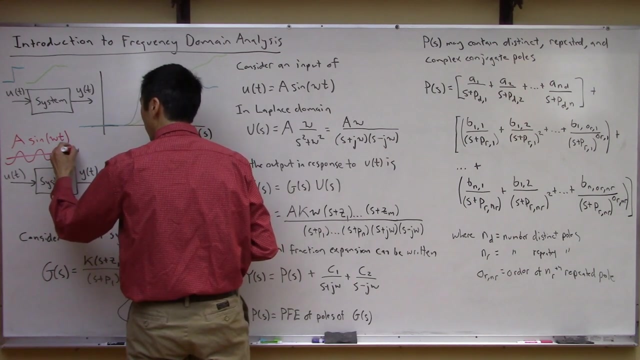 domain analysis is like time domain analysis, except what we're interested in now is using an input of a sinusoidal input to this system. So what I want to consider is a sine wave input, something of the form maybe like a times sine omega t right. So this is a sine wave right With an amplitude of a. 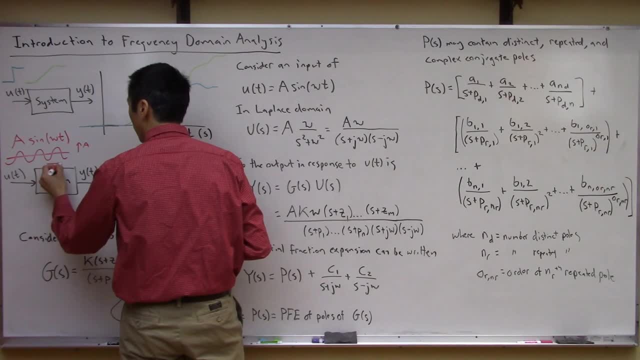 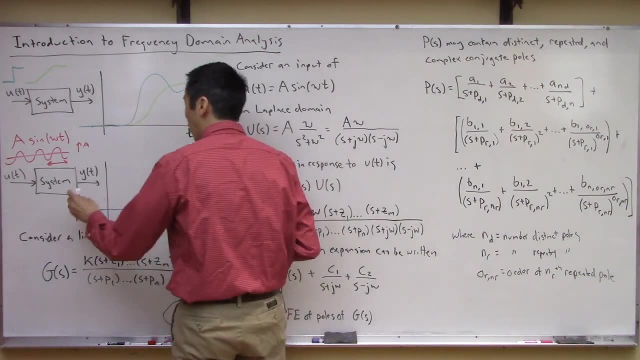 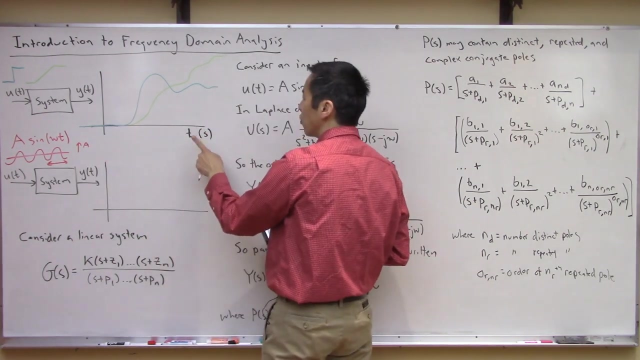 right And it has some angular frequency denoted by omega right. So all we're talking about with frequency domain analysis is: now I would like to understand how does the system respond to this sinusoidal input input? but instead of looking at time as being the independent variable, I want to now look 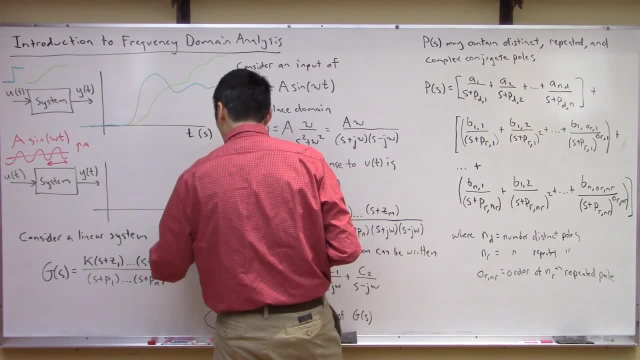 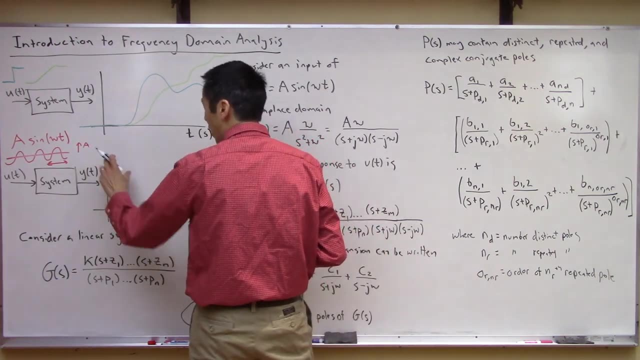 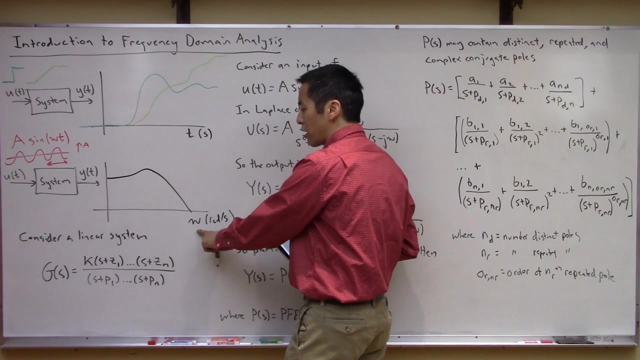 at the frequency of this input omega in, say, rads per second right. And then what I would like to understand is something about the system, and how does that something vary as a function of this input frequency, omega? okay, So again you can almost think about frequency domain analysis. it's almost like a subset of 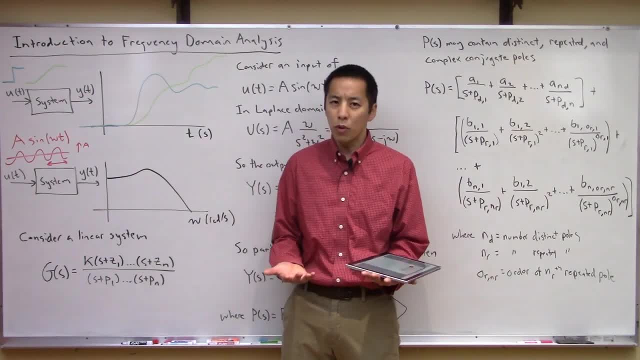 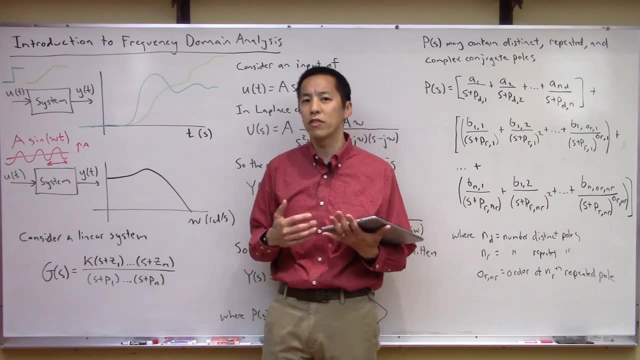 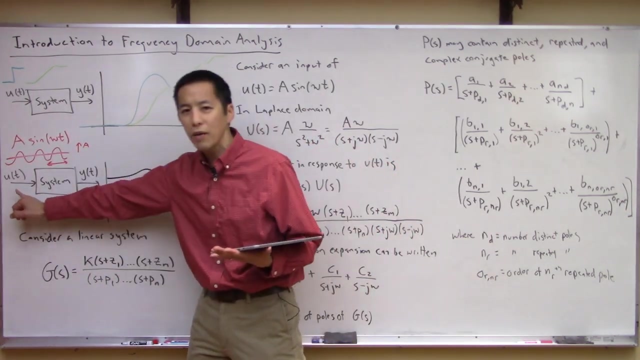 time domain analysis. the only types of inputs we're considering are sinusoidal inputs, and now the independent variable, or the thing that we would like to understand how it affects the system, is now the angular frequency of this sine wave. so we're going to put in some slow sine waves, some medium. 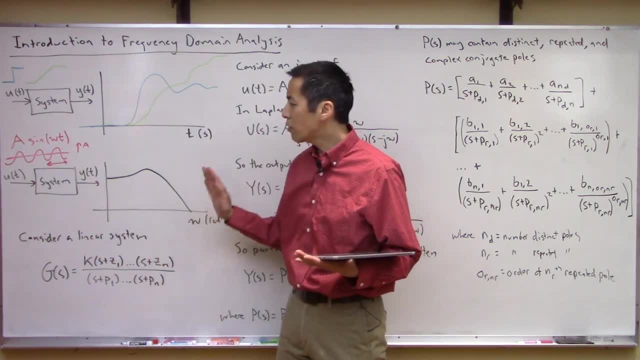 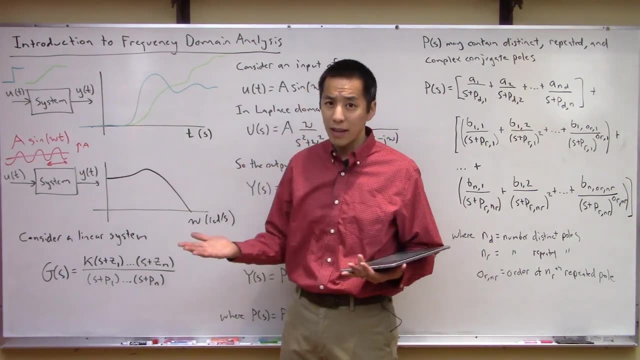 sine waves, some fast sine waves, and we want to understand how does the system respond to those varying frequency sine waves? okay, and we're going to talk a lot about that down the road, but i just want to set the stage, for this is what we mean by frequency. domain analysis is just understanding. 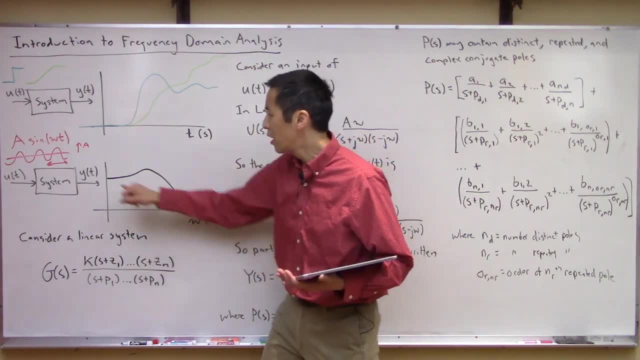 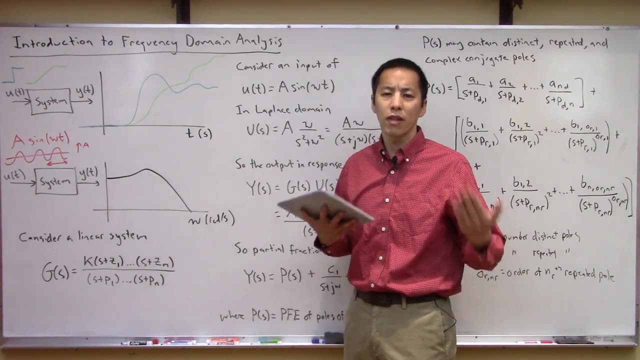 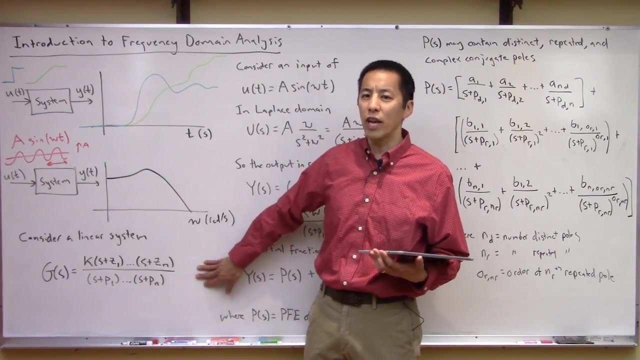 how the system responds as a function of the frequency of the input, sine wave. okay, so that's the setting, and now let's go ahead and jump into it and look at some of the math behind it. so let's go ahead and just consider now a linear system. okay, a lot of the magic and a lot of the 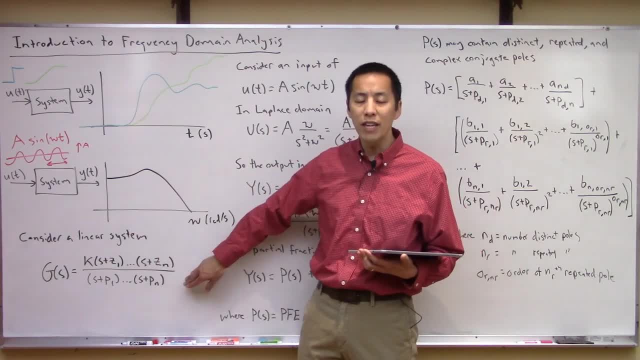 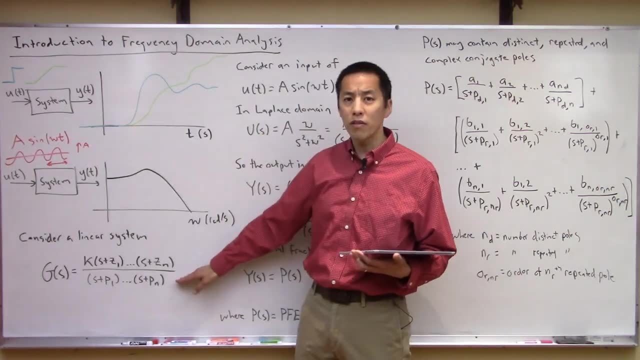 results that we're going to derive now hinge on the fact that we have a linear ordinary differential equation system which represents this box here. okay, so for convenience, we're going to write this in transfer function format. so again, we've got a lot of videos discussing transfer functions. i'm going to assume that, if you're 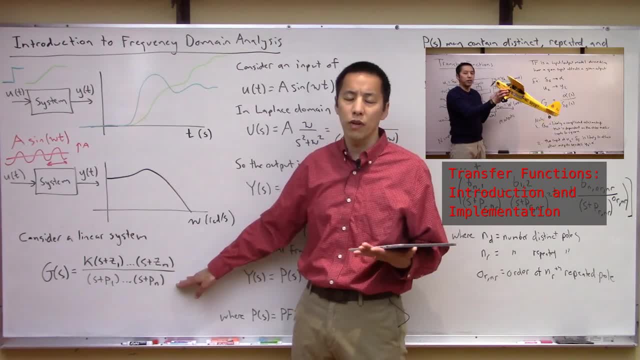 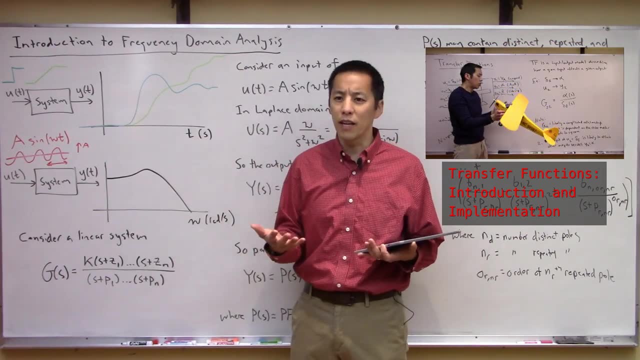 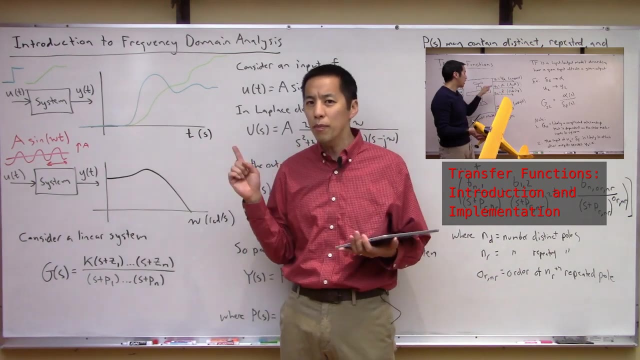 this far in the video series. you've watched some of these future videos on things like transfer functions or time domain analysis, or you're at least somewhat familiar of it. um, with ordinary differential equations and, uh, basic control theory. this is probably not a topic you want to jump into cold turkey, so i would recommend, if you are unfamiliar with any of these terms, 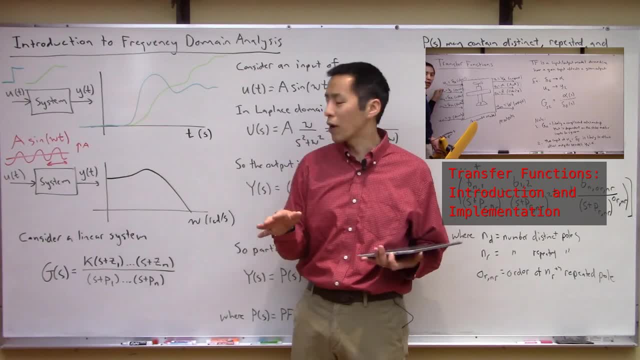 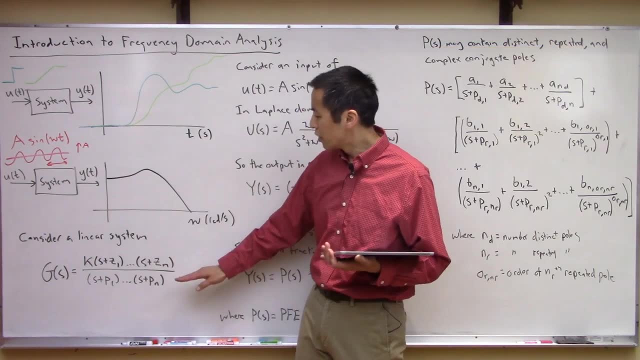 that i'm going to mention here, check out the playlist, watch a couple of these prerequisite videos and then come back to this, because we're going to move a little bit quickly. uh, assuming that you've got a little bit of this background already. so again, let's assume. 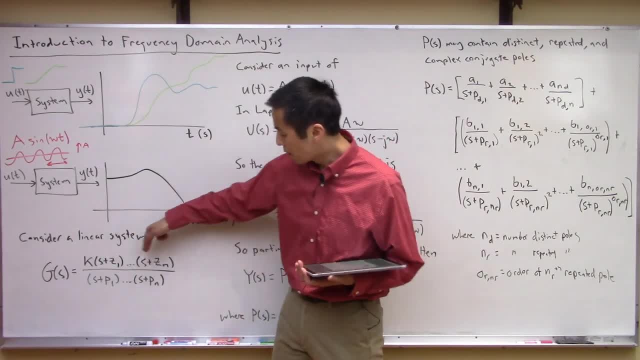 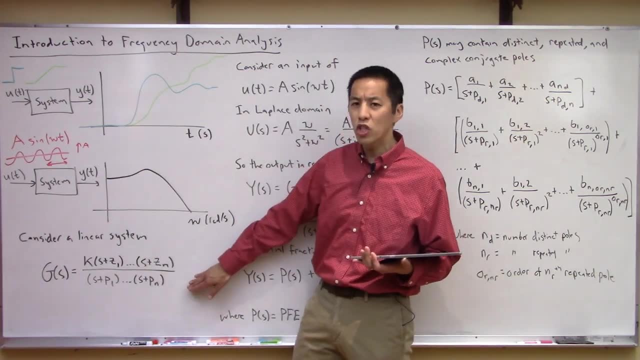 that you've got some linear transfer function system like this, where you have maybe m zeros and n poles, and for now we're not making any assumptions. this is a very generic form of a transfer function. you could have repeated zeros. you can have repeated poles, you can. 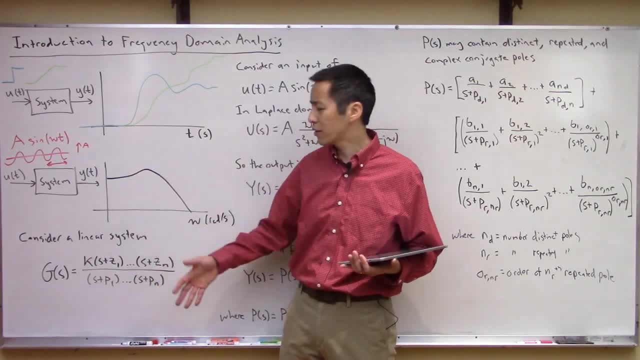 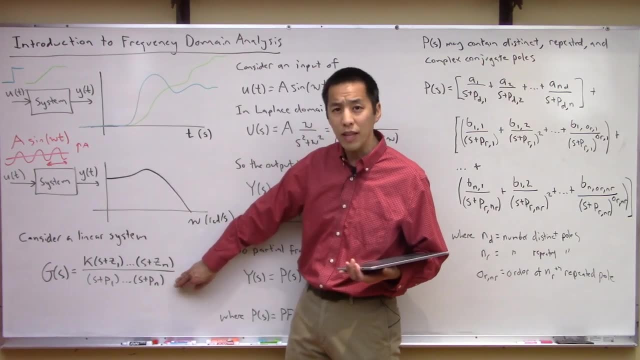 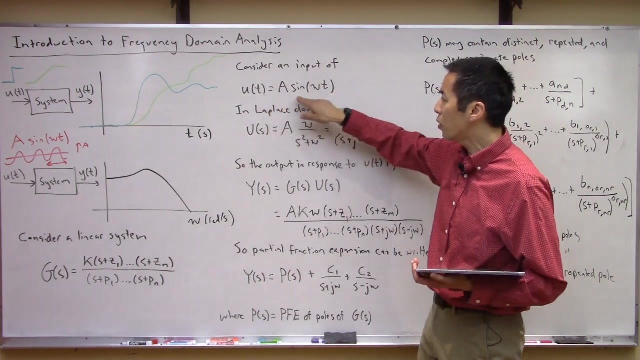 have complex conjugate poles, distinct poles, you know, et cetera, et cetera. this formulation is going is completely generic in terms of a linear system, right? So let's assume you've got something like this, okay, Now, what we said here is frequency domain analysis considers an input of this form. 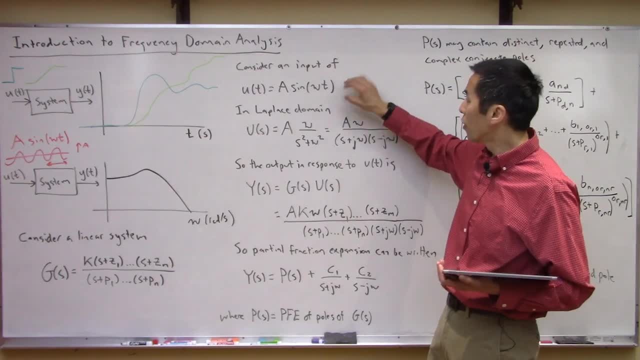 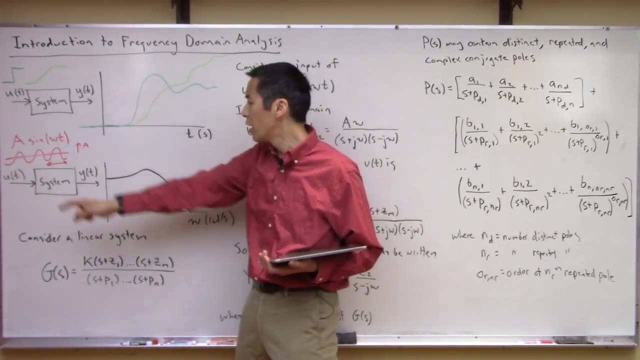 It's a sine omega t, right? So this is what it looks like in the time domain, right? This is that signal. You can just plot this right. It looks really simple. It's just a sine wave. Let's go. 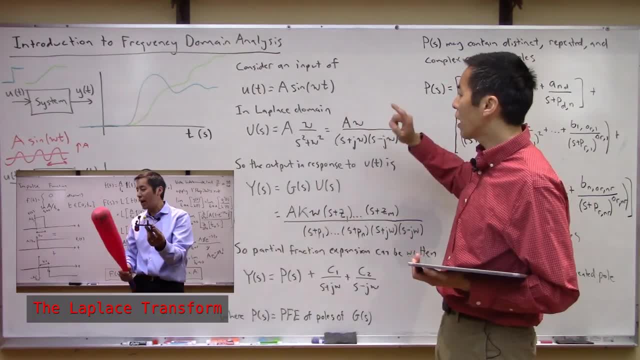 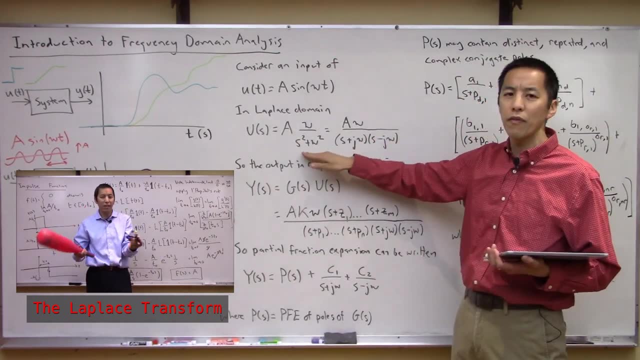 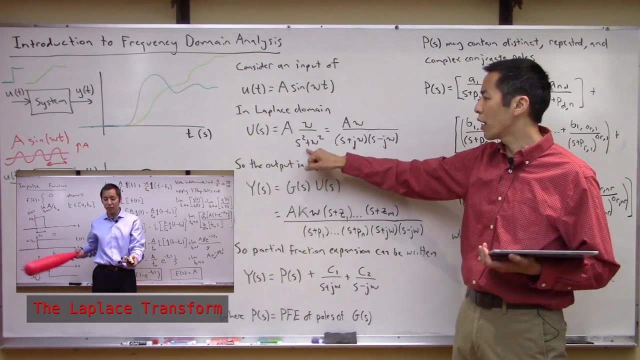 ahead and take the Laplace transform of this. okay, If you take the Laplace transform of this, you basically get this here right? So this is what a sine wave of the form, a sine omega t, looks like in the frequency domain or the Laplace domain. It's just a omega over s squared plus. 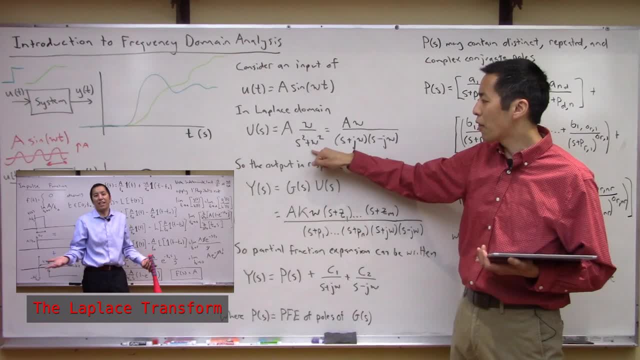 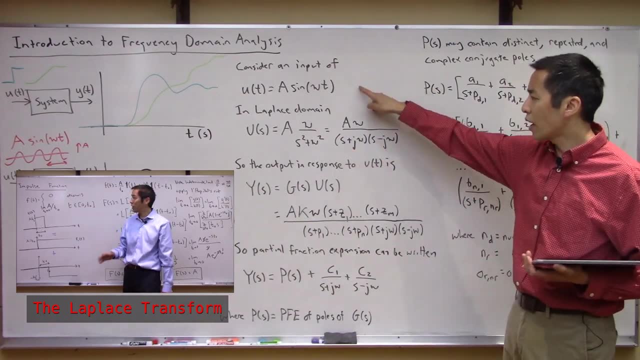 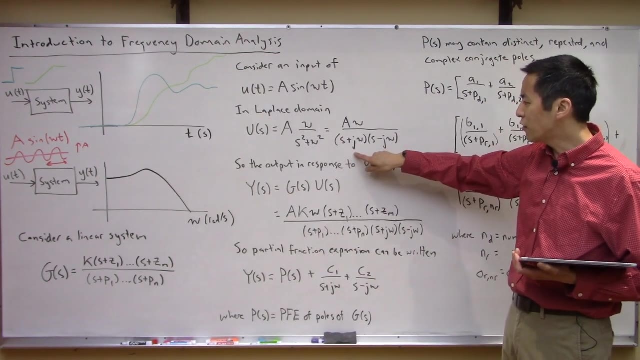 omega squared, or I can basically break up this polynomial into two distinct poles. right Like this, right, This is the same thing. So we see that this sine wave input looks in the frequency domain of aw over a pole at s equals negative j omega and a pole at s equals. 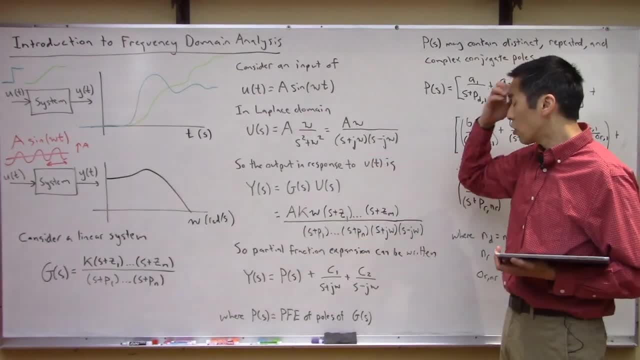 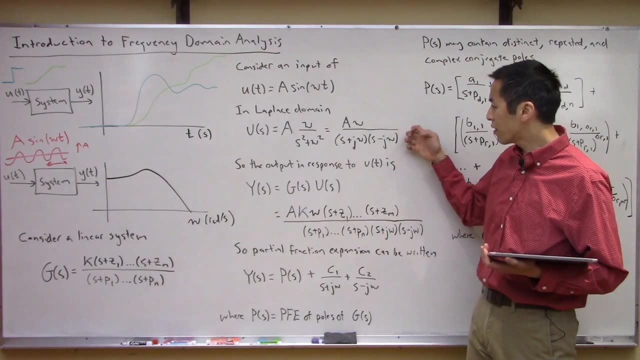 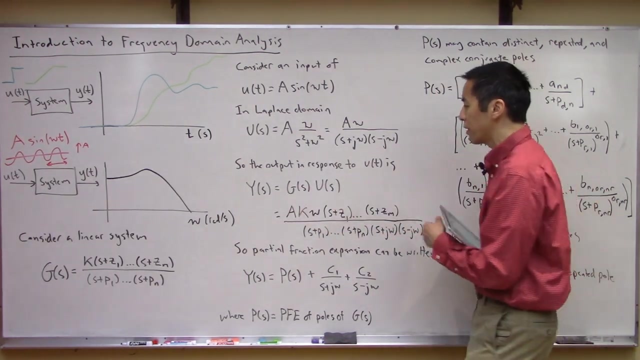 positive j, omega, right, Two poles. okay, So this is the input, So the output in the frequency domain in response to this input, it's just the transfer function times, the input. right, So the output is transfer function times, input. So it's basically this transfer function times. 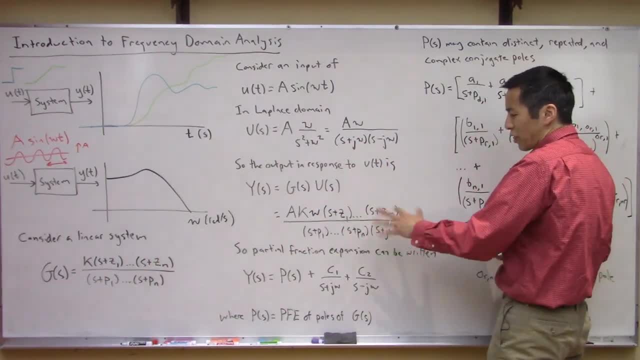 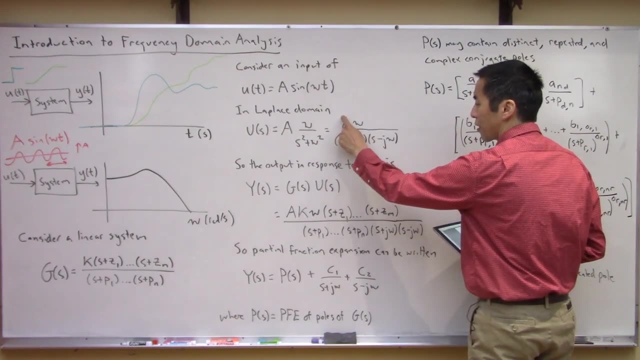 this here And I've just written and you can kind of see I've jumbled a couple of terms or rearranged them, but you can clearly see there's nothing fancy about this. right, You still get the a from the sine wave. You get this k. 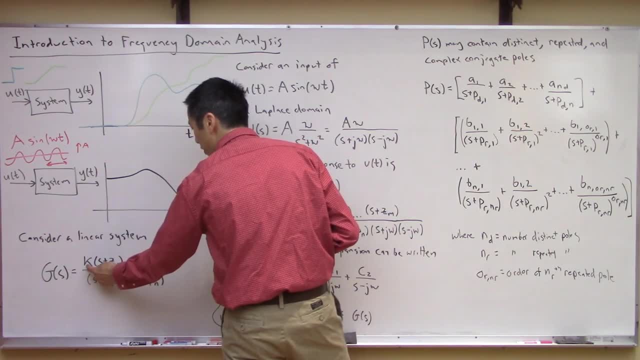 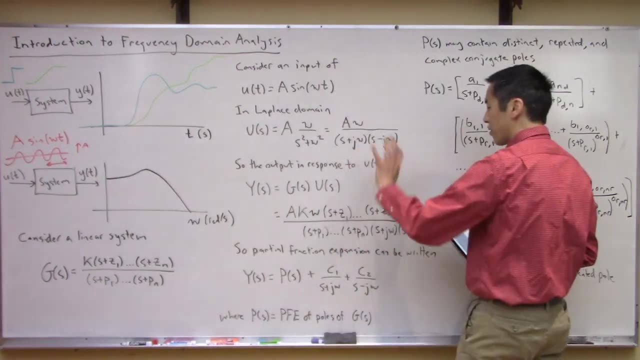 which was just sort of your gain associated with your transfer function. here You get the omega from here. Anyway, again, all this, this is just algebra. I literally just multiplied this by this and rearranged some things, okay, So again, the thing I do want to point out is: let's look at: 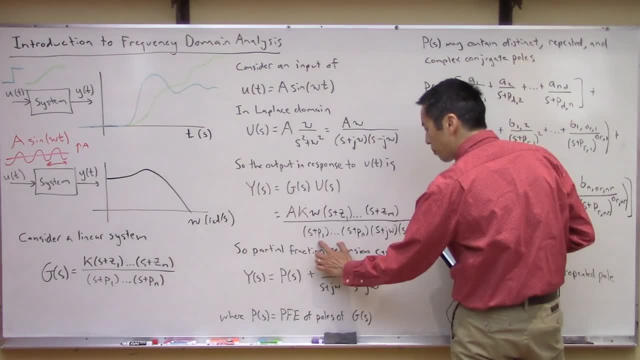 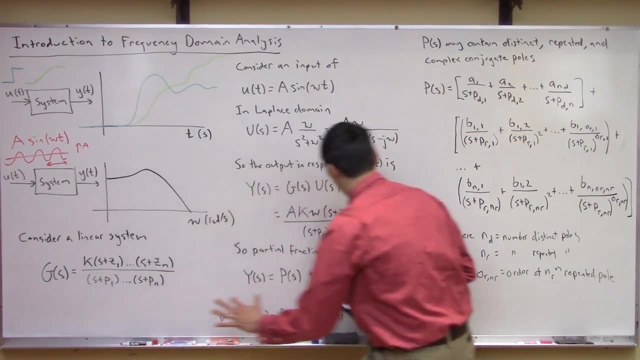 the characteristic equation of this right. You see that these poles, p1 to pn, these are the poles that came from the system right The open loop transfer function here right. Then these two poles of the response here came from the sinusoidal input, right. So 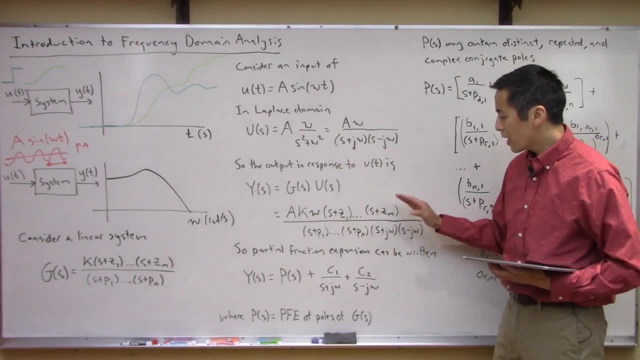 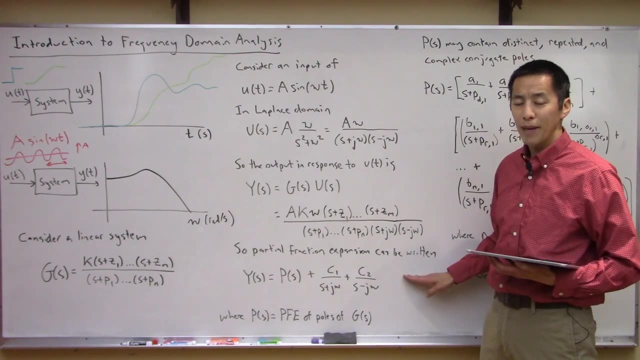 this is what we've got, okay? So what you can do with this is, again, you see that this is nothing more than a ratio of polynomials, right? So you can perform a partial fraction expansion And again, I'm going to assume you've watched our videos on partial fraction expansion. 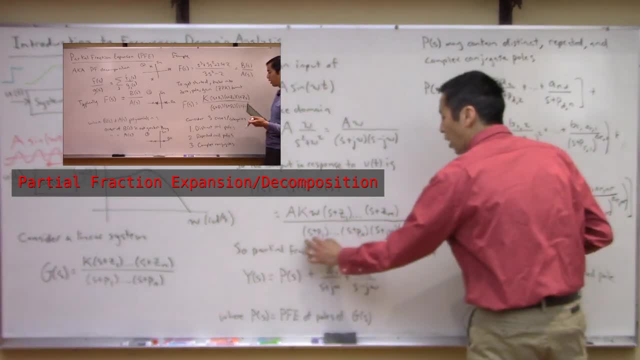 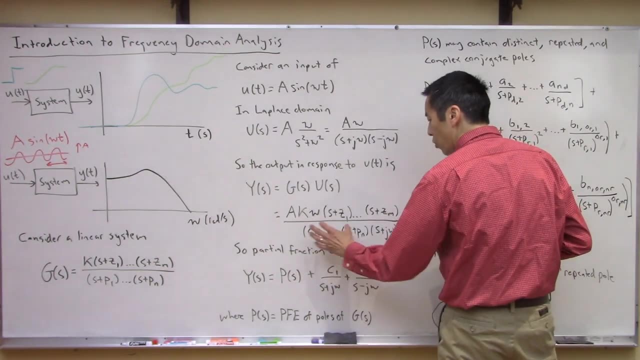 and you know how to do this, And what we can basically do is isolate each one of these poles into their own terms. okay, So what I'm going to do here is we are going to capture all of these poles here associated with the open loop transfer. 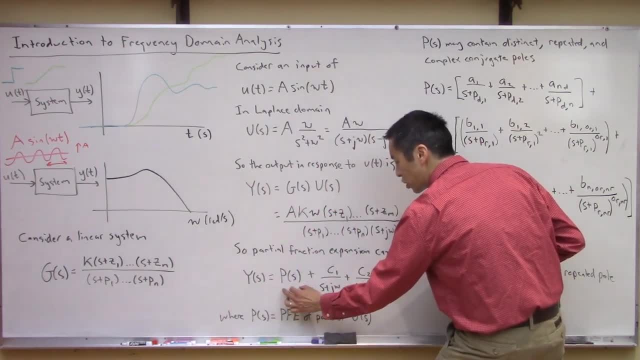 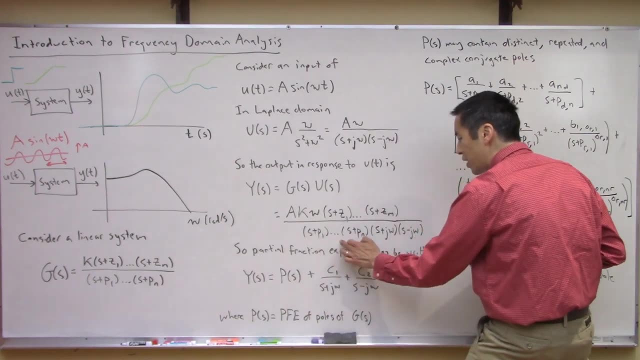 function. I'm going to call its partial fraction expansion, just p of s. So this is the partial fraction expansion component that comes from these poles here right. Then there's these two poles that come from the sinusoidal input. So they are going to have to do a partial fraction expansion. 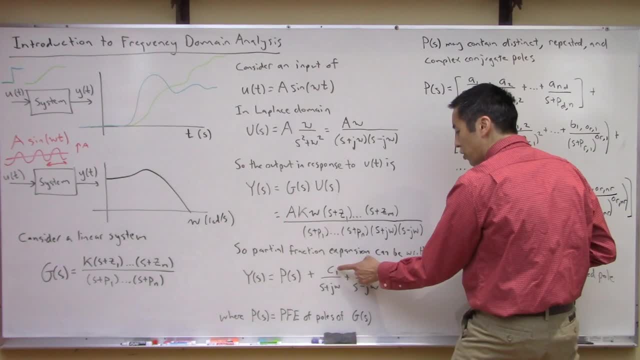 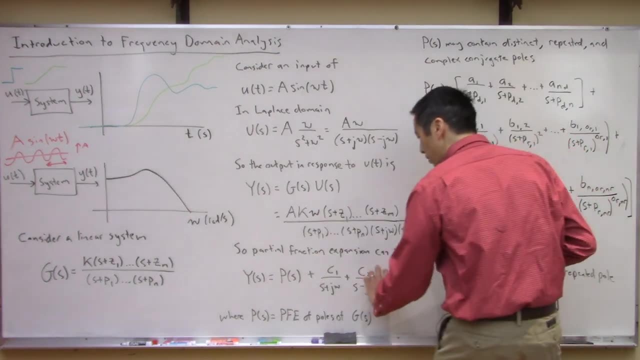 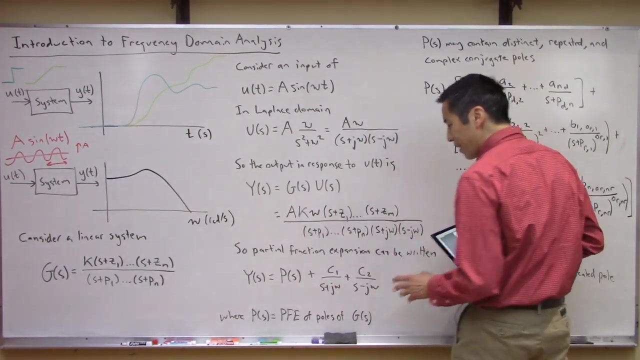 here And again. the numerator coefficients of c1 and c2 at this point are unknown. We are going to solve for those in just a second right. But all I'm saying is you can write the response using the partial fraction expansion as this right. Now where this gets interesting is this: 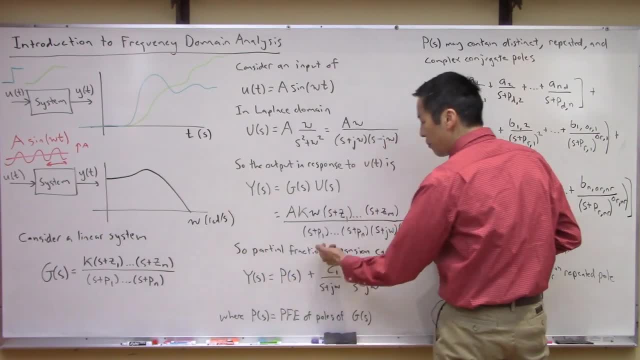 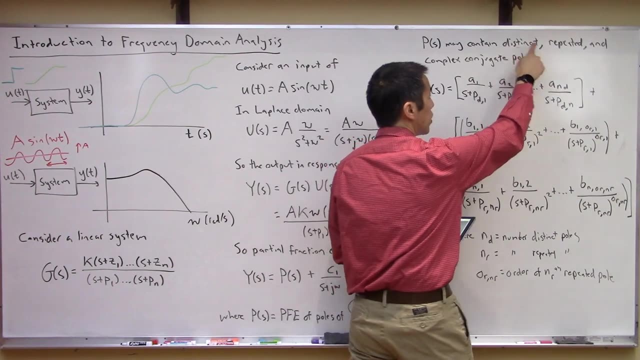 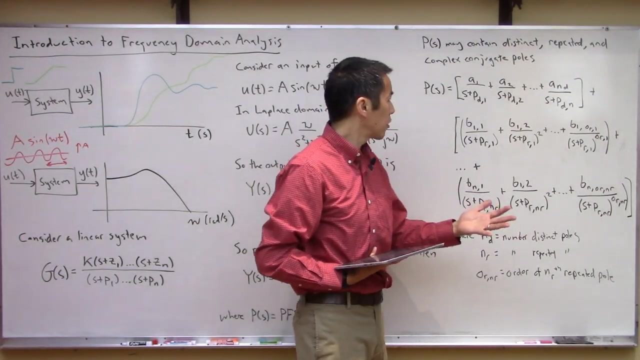 p of s right. As you can imagine, this could be ugly because these n poles, it could be distinct, right. You could have repeated right. So, at the end of the day, a generic form of this p of s, it's going to look something like: 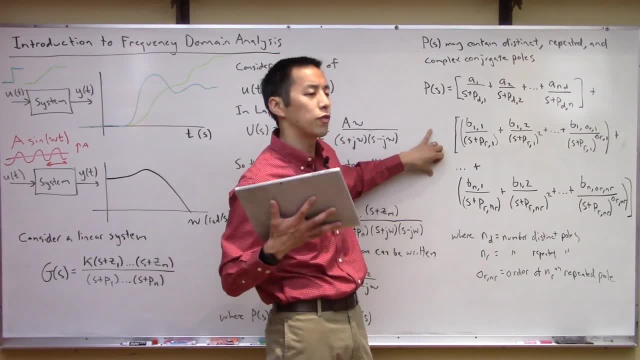 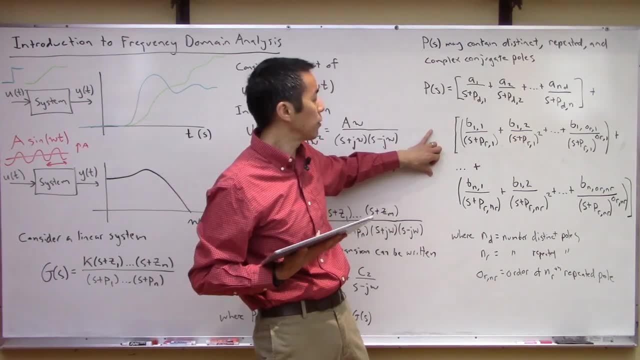 this And it might be ugly. I do want to just write all this down just for the sake of completeness. Luckily, this is going to here. spoiler alert: this is all going to go away in a second once we make a couple of assumptions, But in general, right that partial fraction, expansion of all. 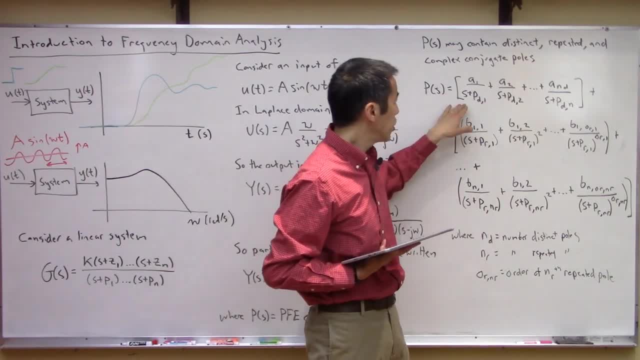 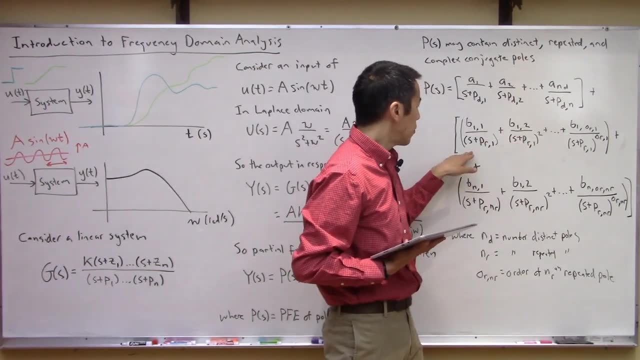 of these kind of poles associated with the open loop transfer function is going to look something like this: You could get you know. here's the partial fraction expansion component related to all of your distinct poles, right, And then you might have, you know, a repeated pole like maybe. 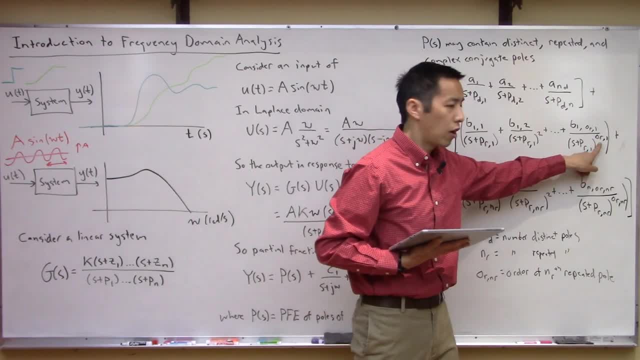 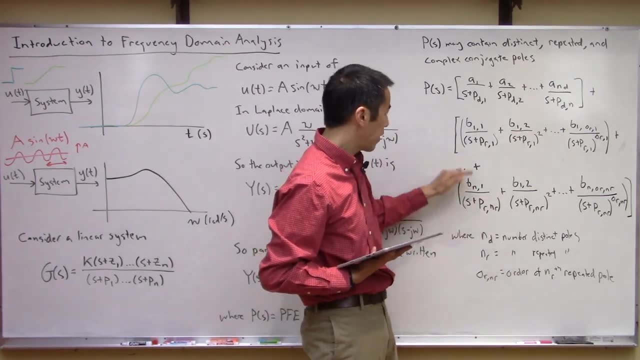 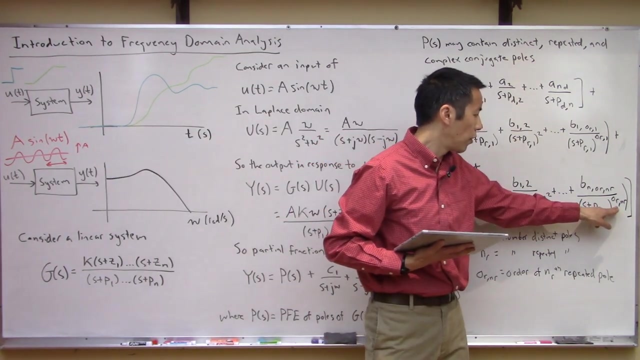 pole repeated number one, has a multiplicity of order or1.. Then you could have another pole that's repeated of or2, etc. etc. You could have it all the way down to you know the nrth pole which is repeated at an order of ornr. 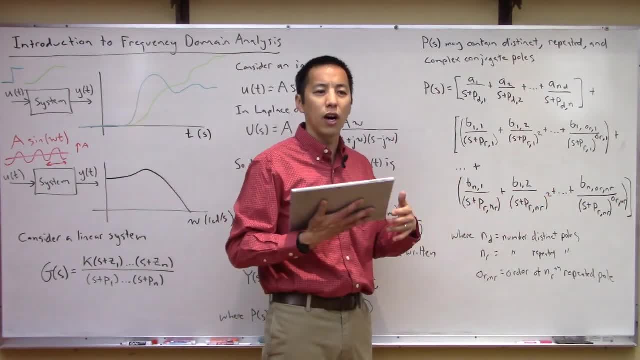 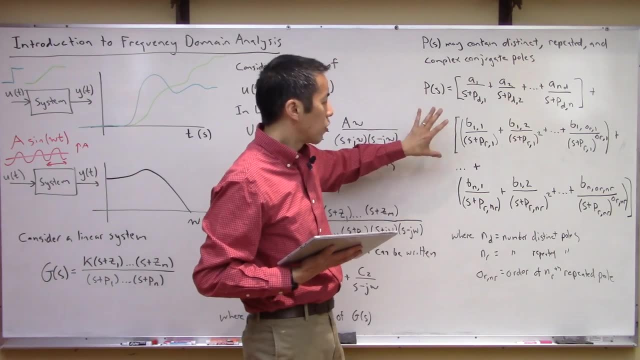 So, again, this is ugly. It's very generic, but it has to be in order to capture all the possibilities, But this is what it could possibly look like right. So now, as we see, this is ugly. 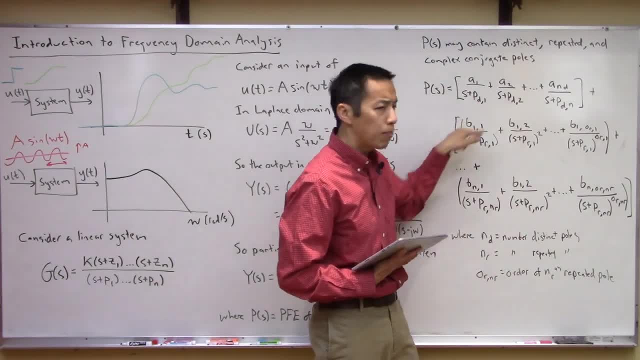 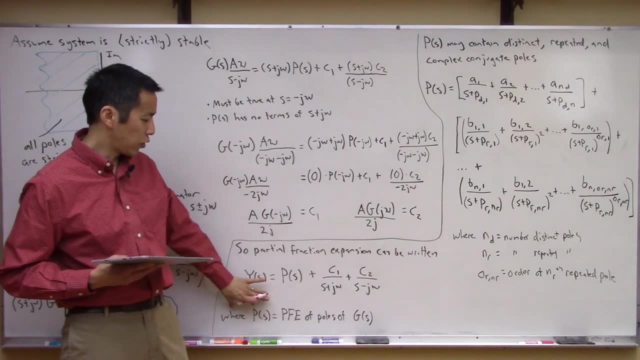 Let's go ahead and make an assumption on where these poles might actually lie. All right, So I actually left some of the board the way it was earlier and I erased others, So this part over here is just like it was. 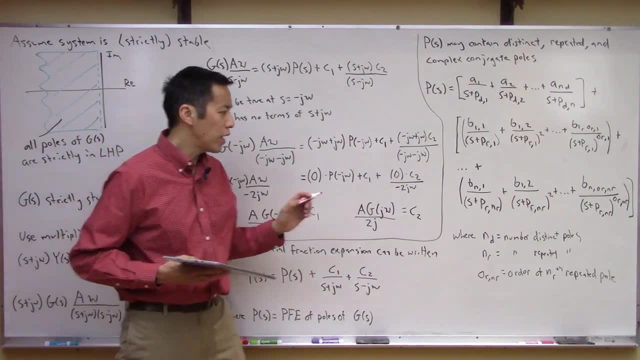 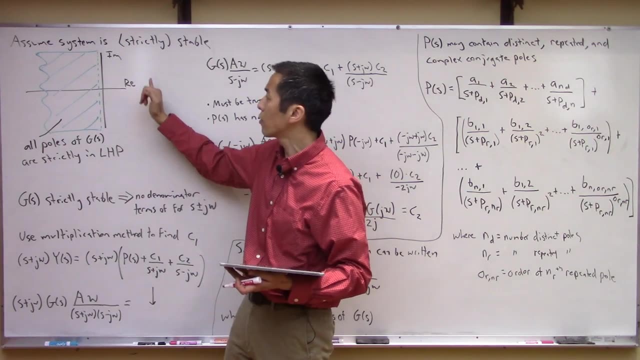 So now again, what we want to look at is what if we had some restrictions on where all these poles of the open loop transfer function are? So that restriction I'd like to now consider is: let's assume that the original transfer function G of S is strictly stable. 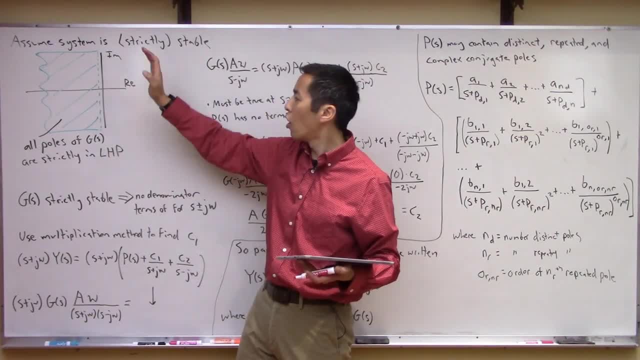 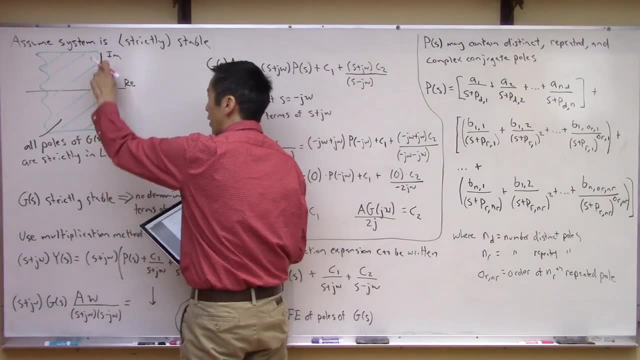 And again this strictly adjective. what this means is that all of the poles of G of S are strictly in the left half plane, meaning they cannot be on the imaginary axis right. Sometimes people refer to that as kind of like neutrally stable. 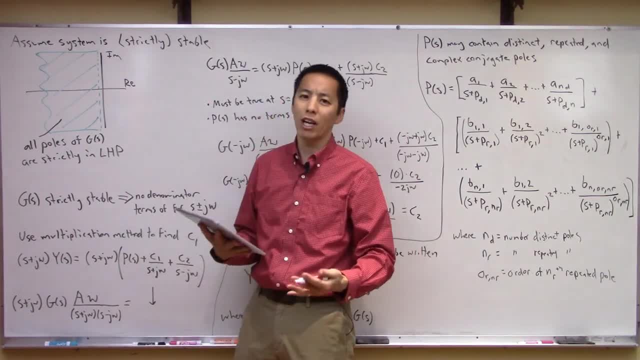 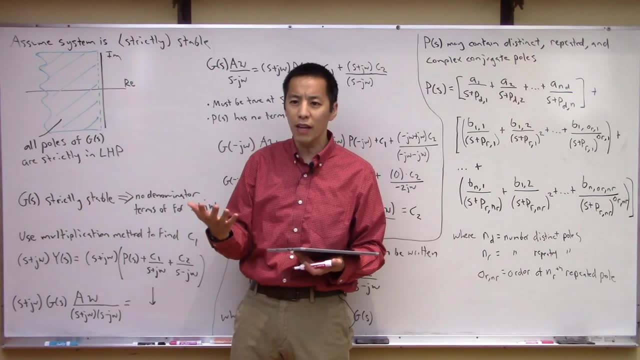 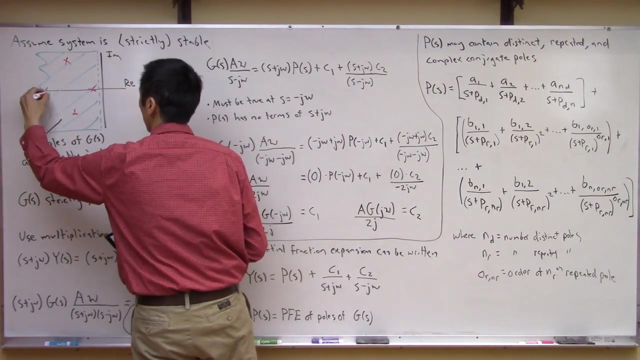 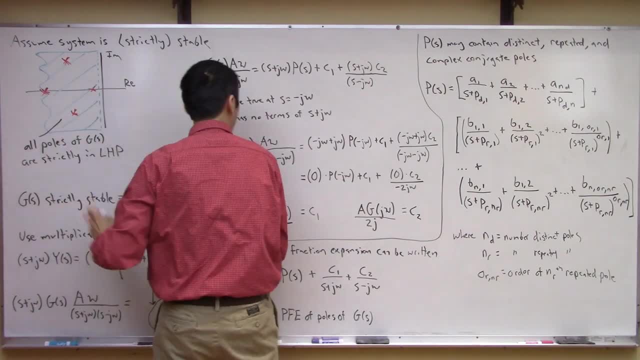 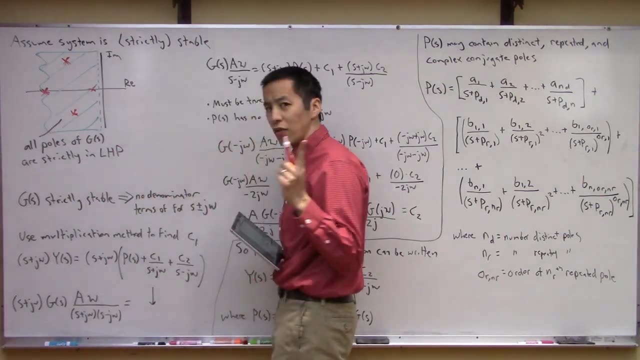 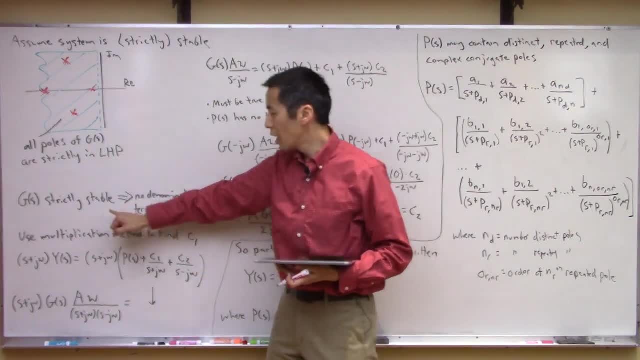 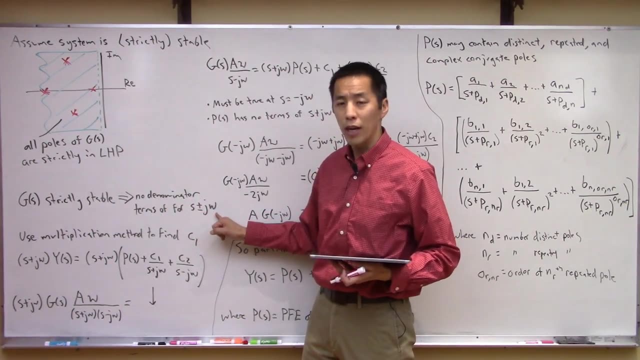 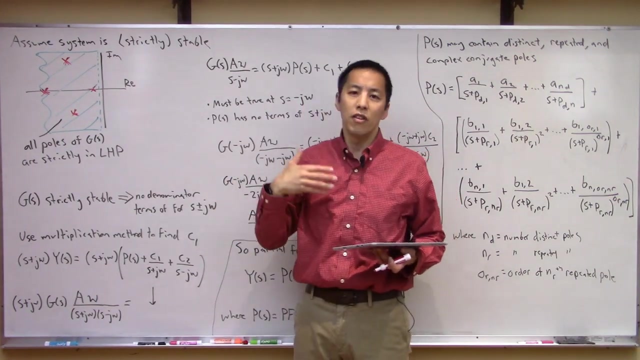 think about that long enough- is if g of s is strictly stable, that implies that g of s there are no denominator terms of the form s plus or minus, j, omega, right, because this is poles exactly on the imaginary axis, which we said is now not allowed. so again, this is one assumption we're 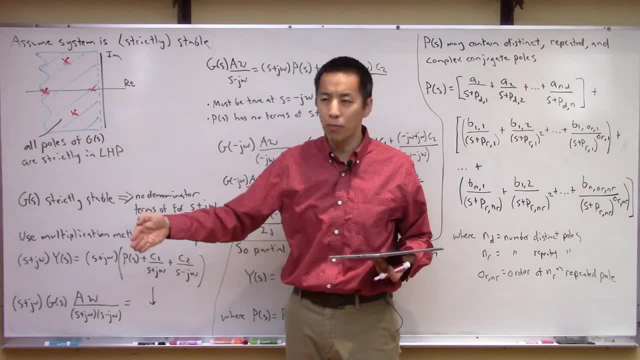 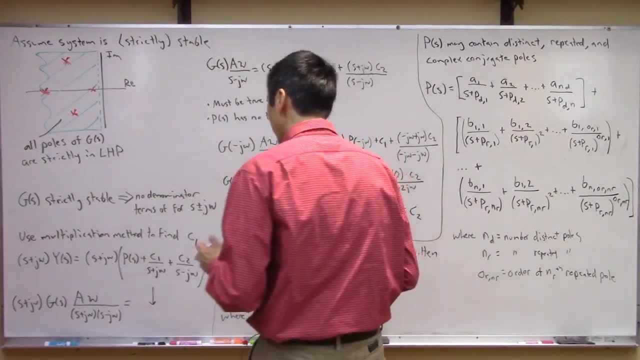 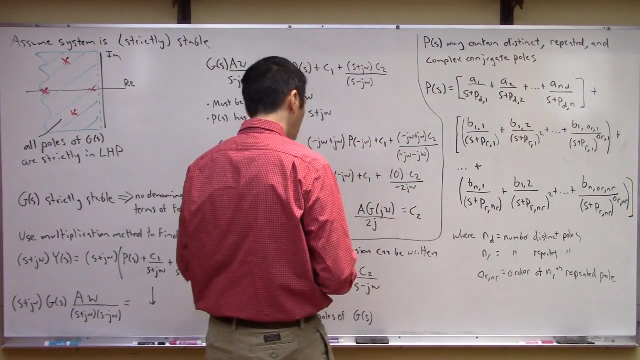 going to have to make going forward in order to move past this point. okay, so let's assume this is true. okay, and now, if that is true, what we can now do is we can start asking ourselves: how can i go ahead and, um, find, uh, basically, what are these coefficients c1 and c2? right, we said 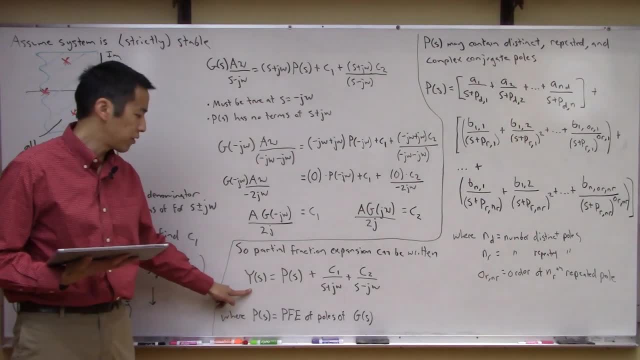 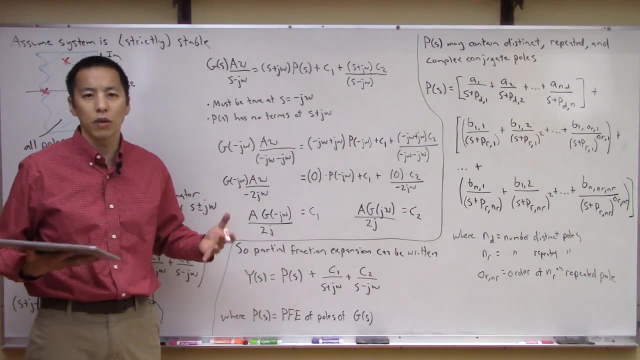 here. this is y of s right. we found what the output of the system is in the laplace domain. i need to find these coefficients c1 and c2 via partial fraction expansion so i can understand what this might look like in the time domain. okay, so the way we're going to do this, 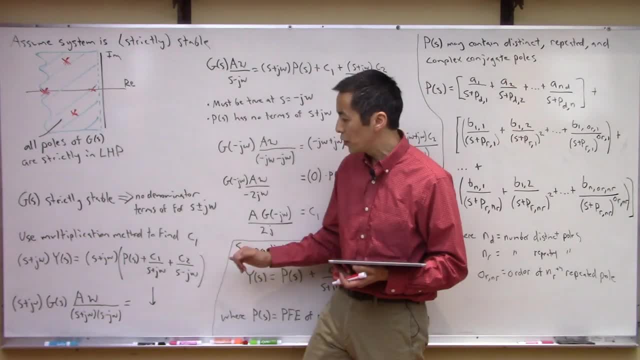 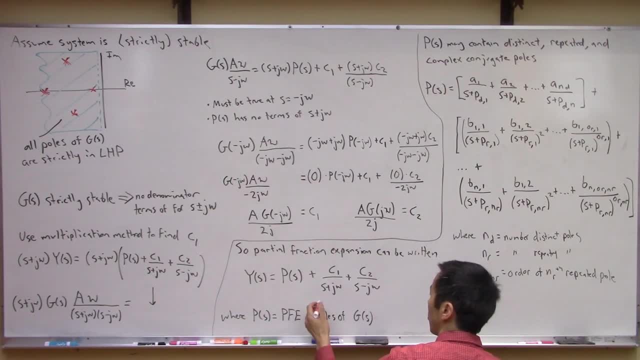 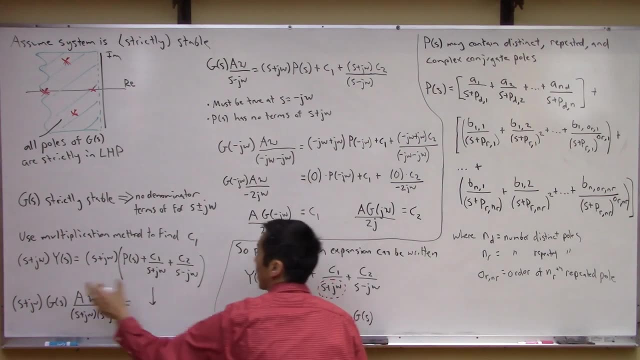 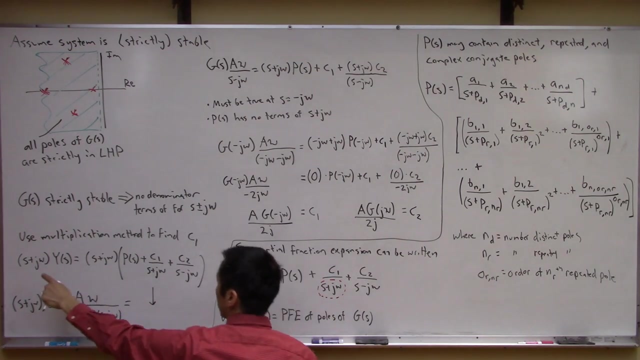 is, we're going to take this output and we are going to multiply it by the pole associated with C1.. So you can see, all I'm doing is multiplying the left-hand side and the right-hand side by S plus J omega, right? So multiply the right side by S plus J omega. okay? So now let's go ahead and 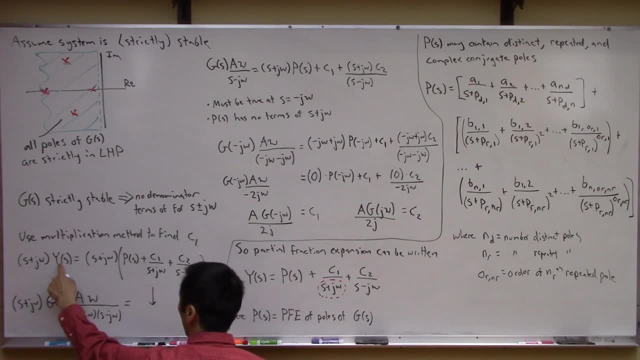 go down one step. Let's see The output: Y. Y is just G times the input. right, And the input was this sine wave, right, So Y here. this is basically this term here. right, This is G times the input. 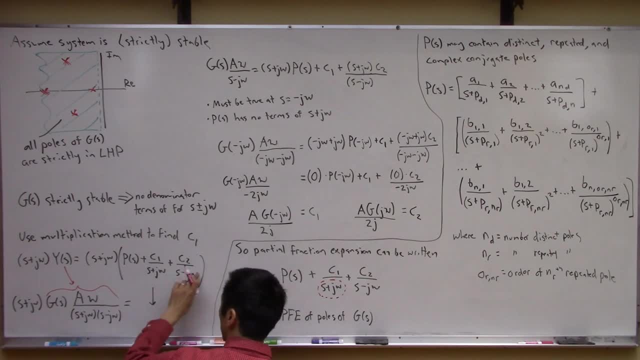 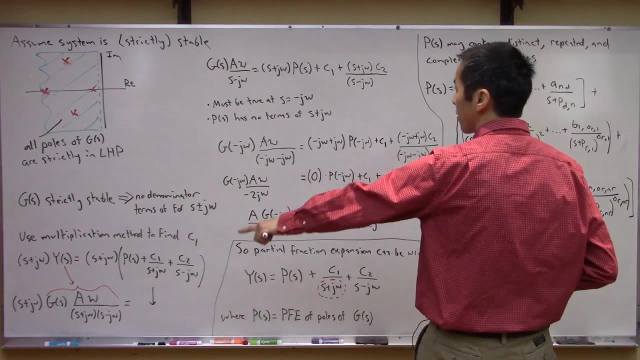 right, Okay. And then the right-hand side is just this gobbledygook, right Same thing, okay, Let's simplify even further, okay? So now what I can do is let's see here, Well, a couple of. 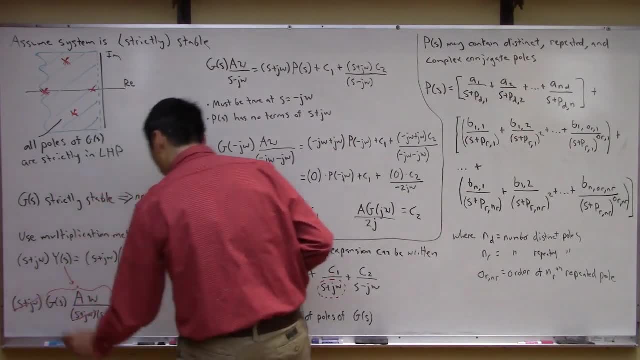 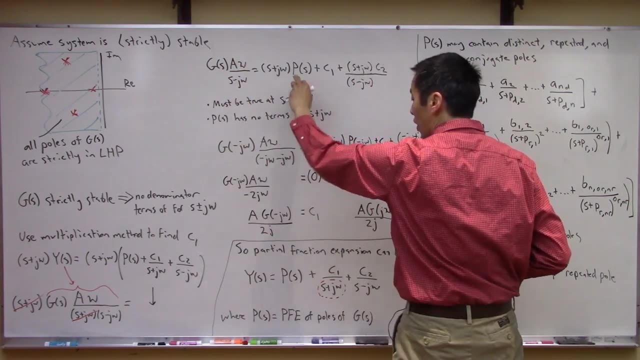 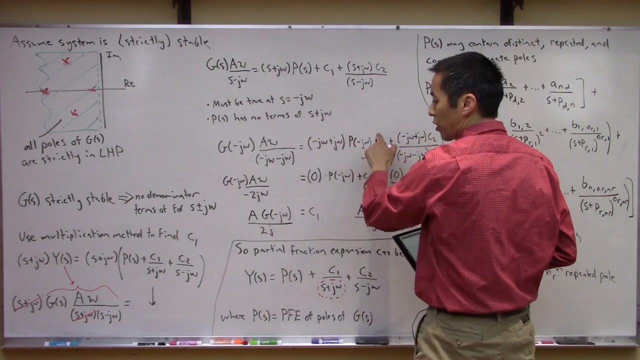 things happen, right? So this cancels with this, right. So the left-hand side becomes just G A omega over S minus J omega, right, Okay? And now on the right-hand side, let's distribute this S plus J omega into this term, this term and this term, right? So that's what you end up with here. 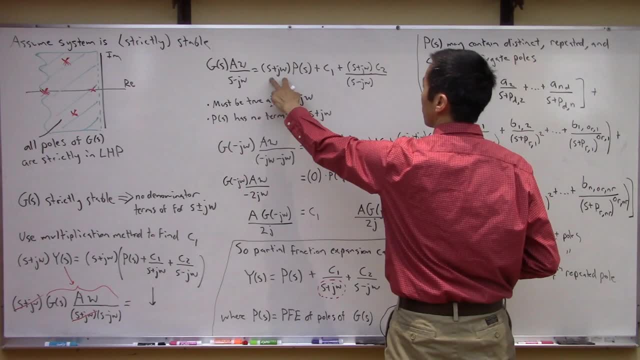 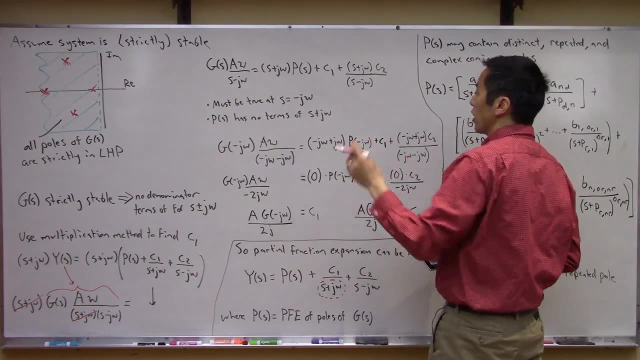 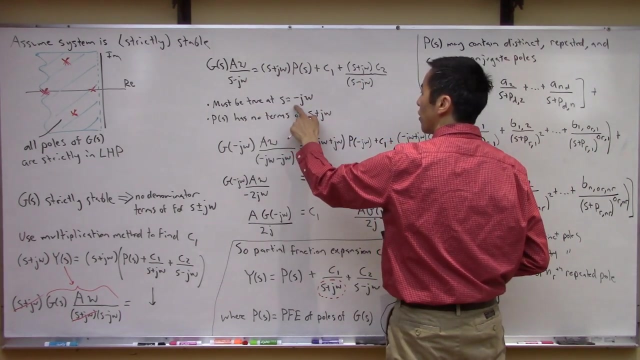 As you can see, this S plus J omega will cancel with this S plus J omega, So we basically isolate C1 by itself. right, Okay, great. So this is our equation we have now- This has to be true at all- values of S. so let's choose an S value of. 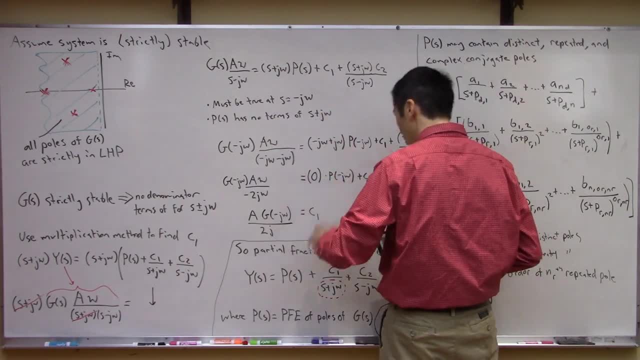 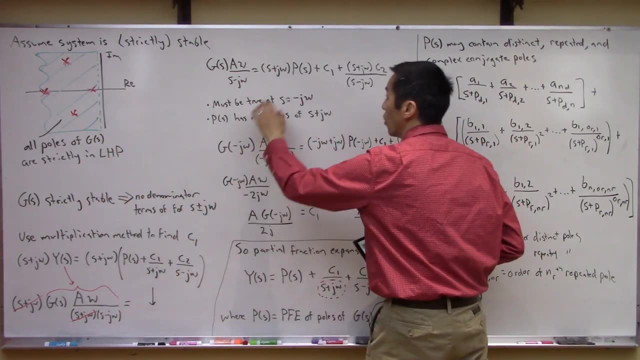 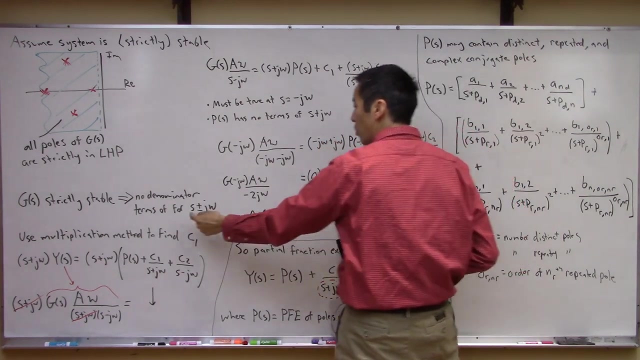 negative, J, omega, right. Okay. Now the other thing that we can notice now at this point also is: remember: we said we assumed all the poles were strictly in the left half plane. So this term P of S- right, There are no terms that look like S plus J, omega in it, right, This is exactly what. 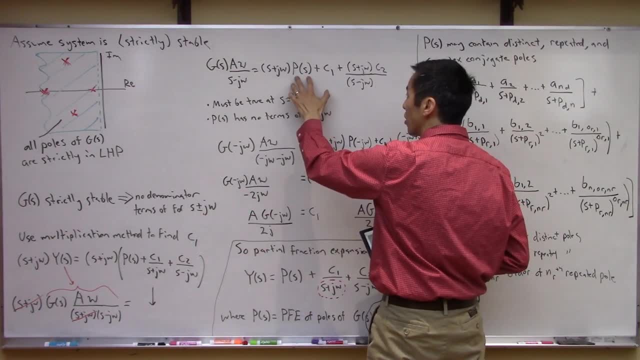 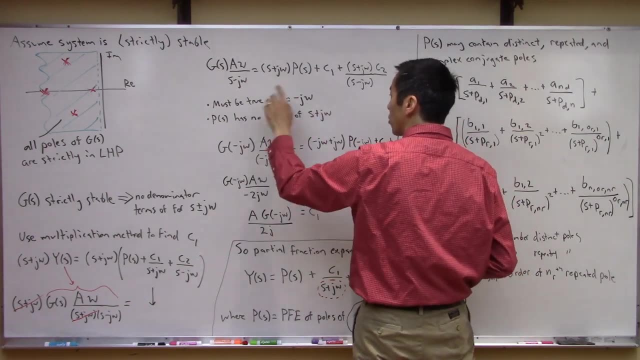 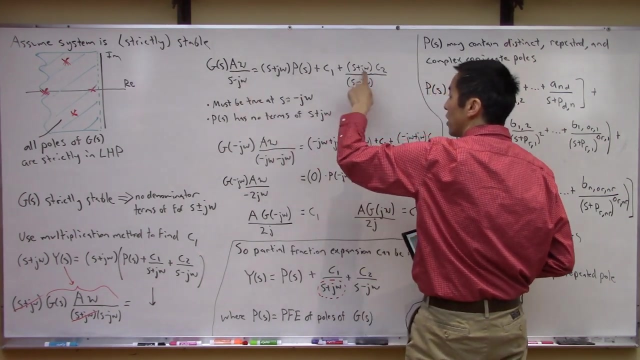 we talked about right here. So, in other words, nothing in this denominator will be able to cancel this term here, So this is going to stick around, okay. So with that in mind, let's go ahead and evaluate this function here at. S is equal to negative J omega. So in other words, everywhere you see an S in here. 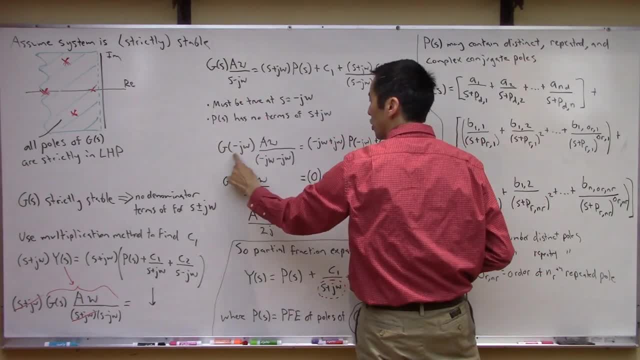 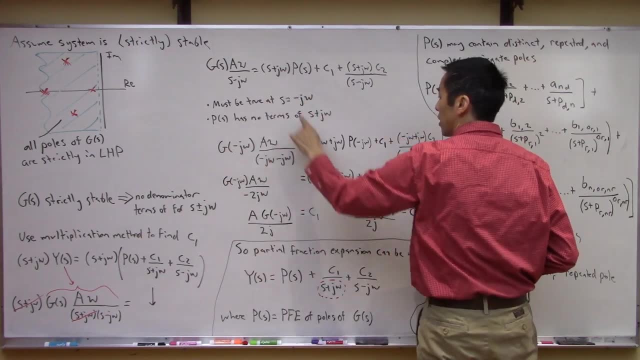 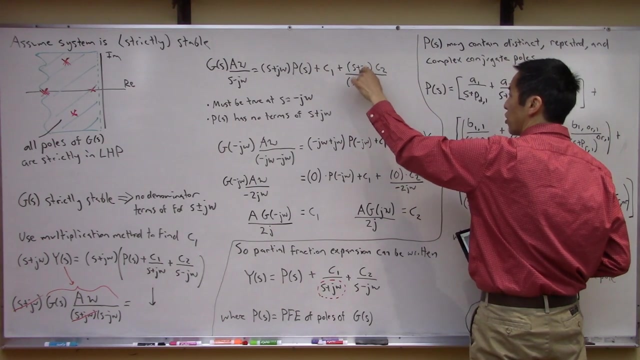 just jam in negative J omega. So this G of S becomes G of negative J omega. This S down here becomes negative J omega. Same thing over here. This S becomes negative J omega. This S here becomes negative J omega. C does nothing by itself. And then same thing over here. You can plug in J. 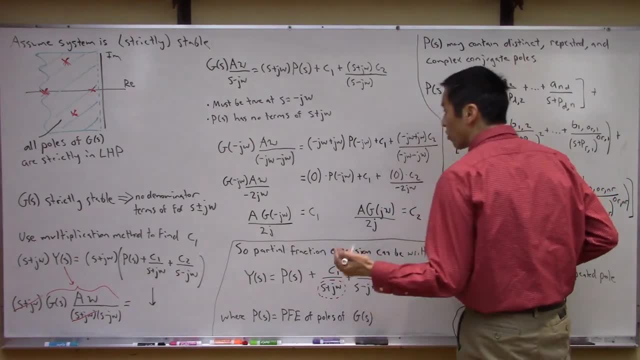 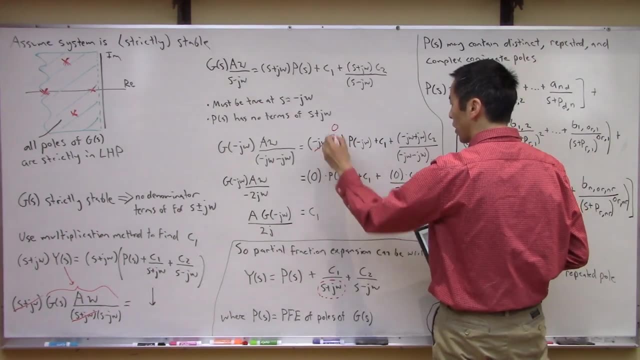 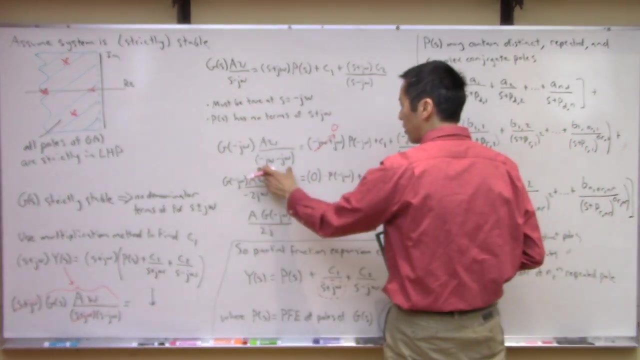 to S's and this is what you end up with, right, Okay. And now this is where this is beautiful, because now we see, okay, what is this right here? This is just zero right. And same thing right here: This term is also just zero right. And what else is nice? This bottom is just negative. 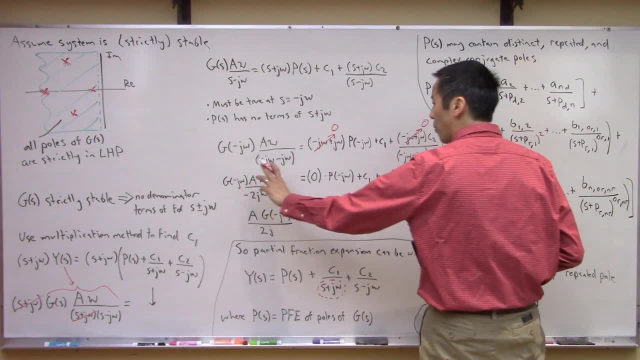 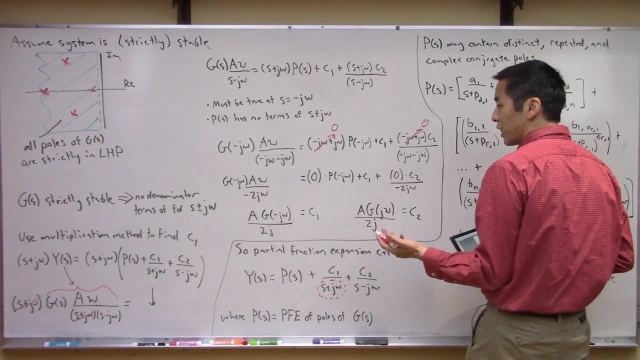 two J omega, right, Okay. So basically what we end up with is this: down here, right, Here's the zero, the zero. So this is starting to get cleaned up quite nicely. right And again, we can also probably notice that this omega will cancel with that omega. So the left. 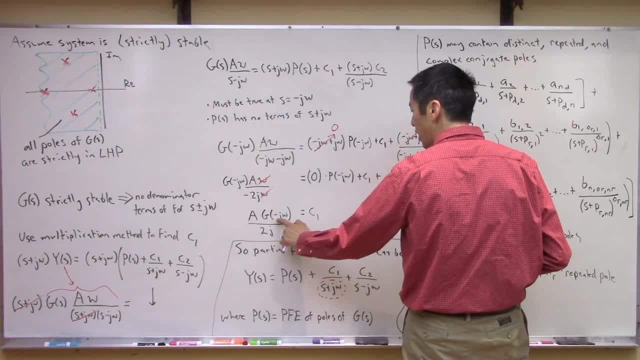 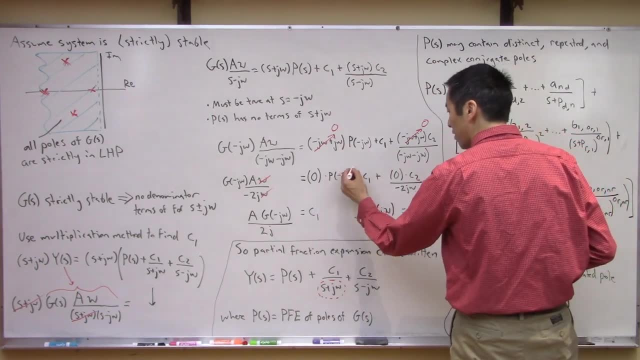 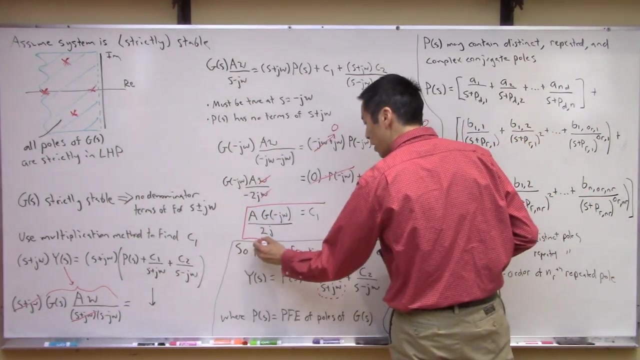 side boils down to this really nice form. We get A times G of negative J, omega, all over two J And the entire right-hand side. you know, this gets knocked out right, Because there's a zero there. This gets knocked out. We end up with just C1.. So this is actually the C1 coefficient. 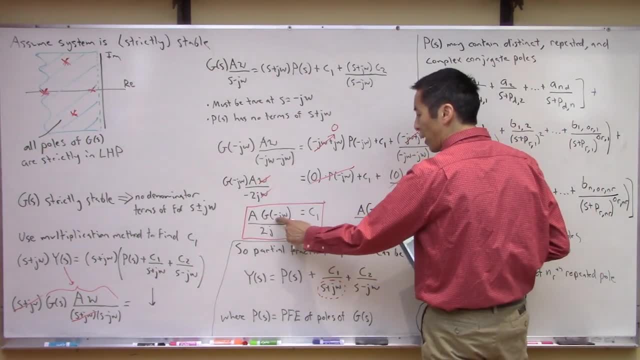 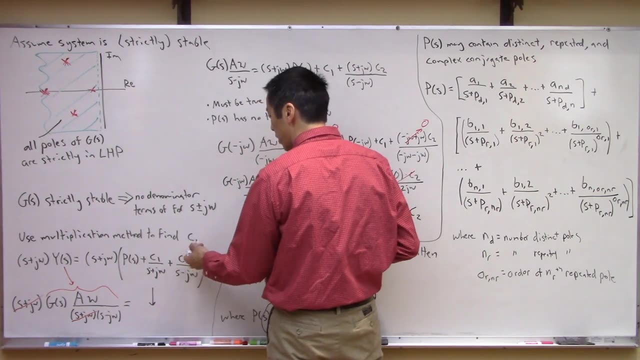 right, It's just A times. the transfer function evaluated at S equals negative J, omega all over two J. And you can do the exact same thing by going back and using the multiplication method to find C2. now right, You just have to do a very small modification. Now we're going to multiply. 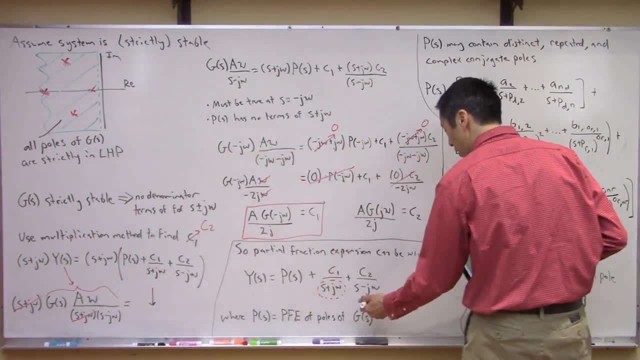 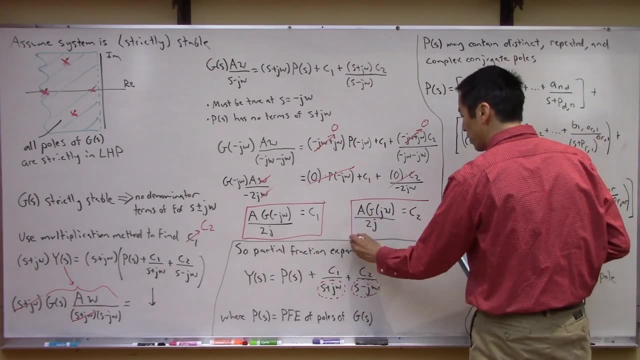 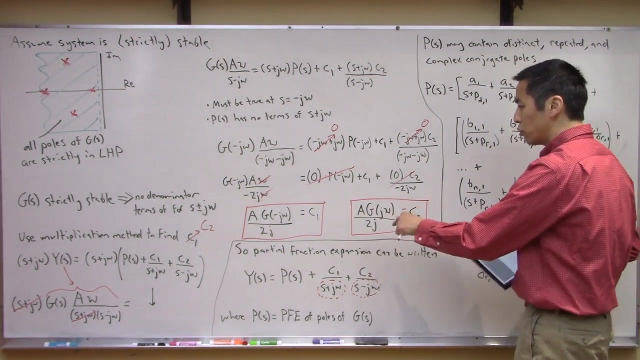 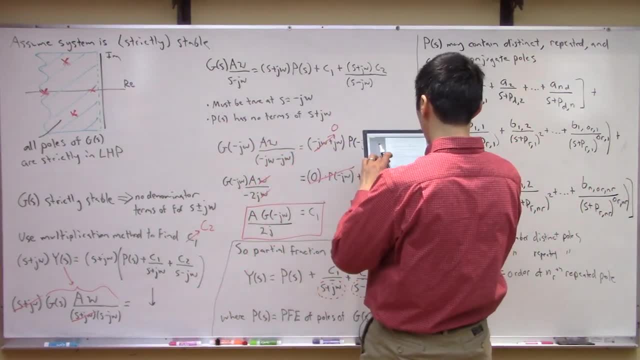 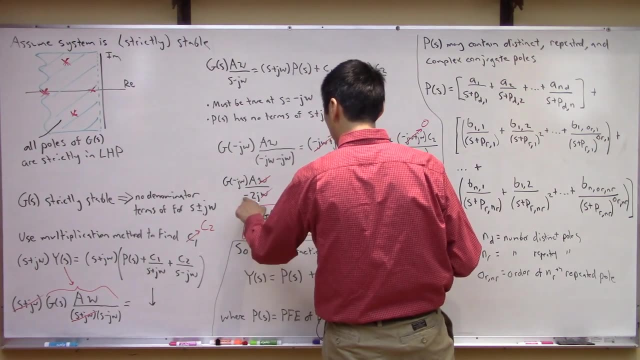 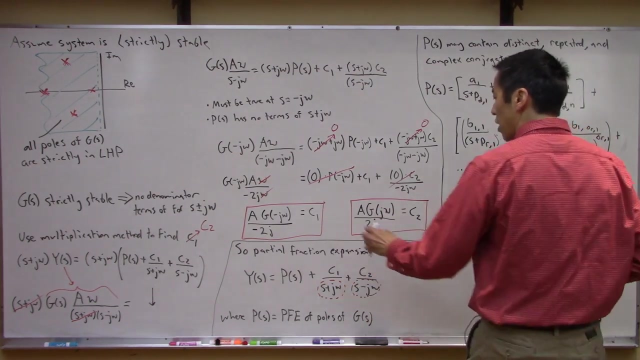 sign. hold on, hold on, hold on. i think my c1 here needs to have a negative hold on. yeah, sorry, this should be. this should be a negative. uh, down here, right, yeah, because it's negative. 2g, right, okay. yep, that's correct. there we go. okay, great, save these, we are going to need this. so um tell you. 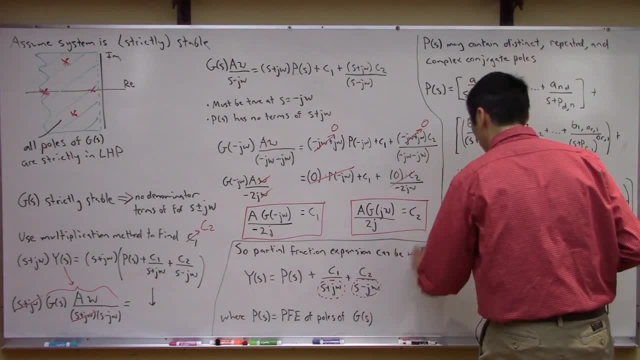 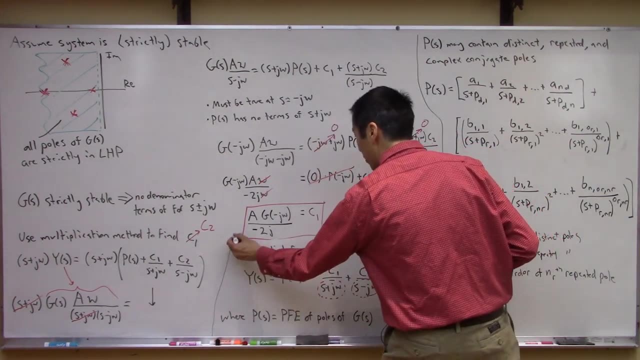 what? um, let's go ahead and move our little line of saving, right, this is where i want to save all of my stuff, so we're not going to erase it. let's move this line up to encapsulate these two bits as well, because we now need to put all this together. okay, give me a second to erase. 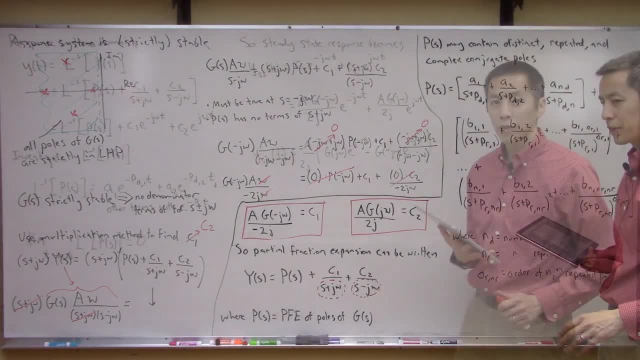 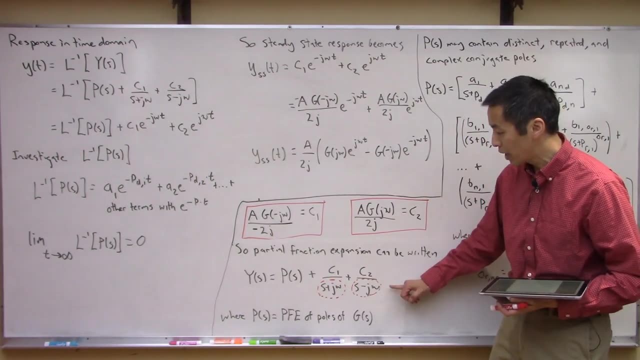 all this other stuff. we'll keep this and then we're going to keep trucking, all right. so now this is getting exciting because again now we have the response of the system in the laplace domain. is this right? so to get the response in the time domain, let's just take the. 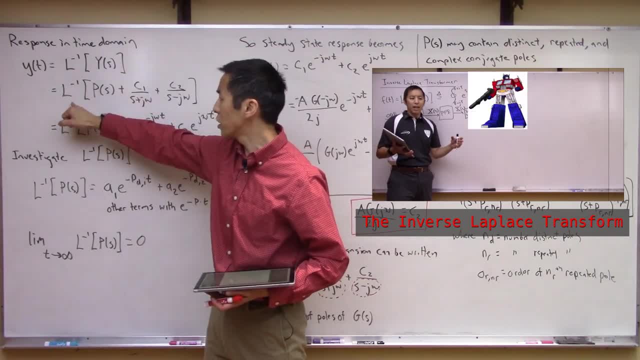 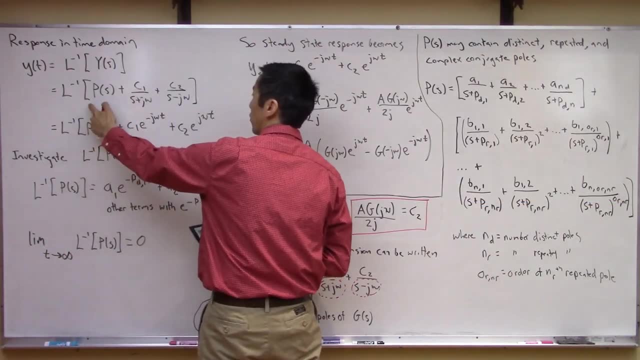 inverse laplace transform of it. right? so, in other words, i'm just going to take the inverse laplace transform of this term right here, right. so here it is. and, as we know, this inverse Laplace transform operator, I can just distribute it in: right, it's? uh, it's a linear operator, so it's the Laplace transform. 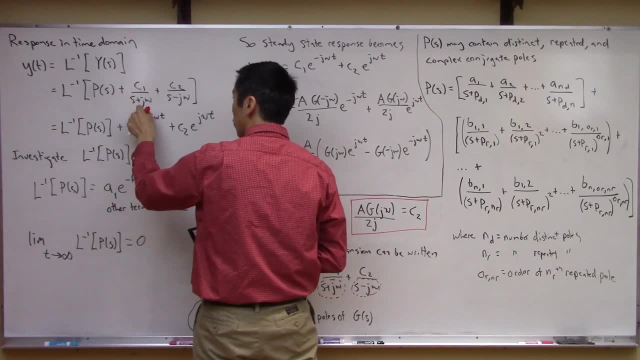 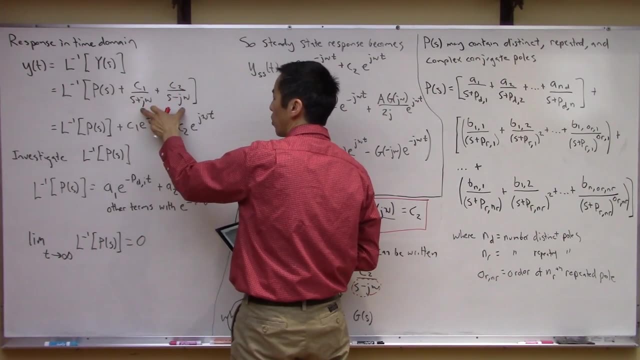 or the inverse Laplace transform of p of s plus the inverse Laplace transform of this plus the inverse Laplace transform of this. well, these two terms are fine, they're. they're basically distinct poles. so we know the inverse Laplace transform of c1 over s plus j1, that's just c1. 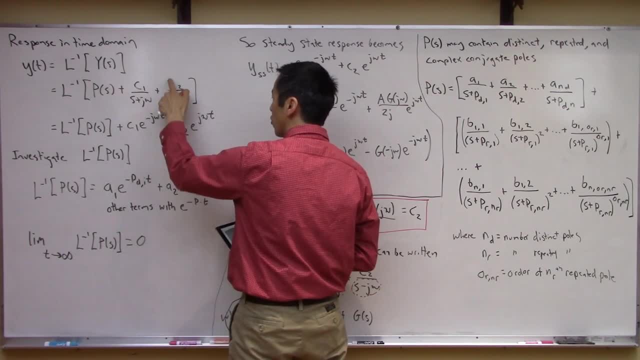 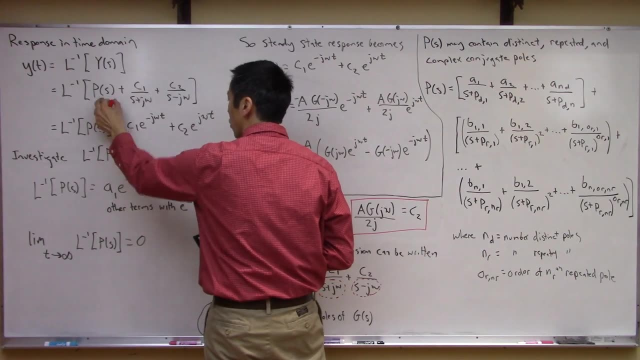 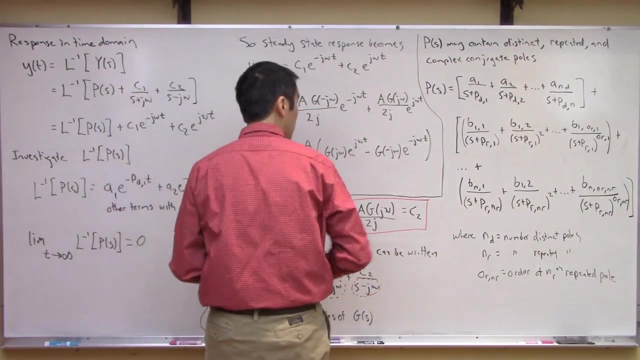 e to the minus j omega t right and same thing. this term here, the inverse Laplace transform is just c2 times e to the j omega t right. so we got these two terms. now this one is a little bit cumbersome- is maybe the right way to describe it, right, because we know p of s it's this. it's this. 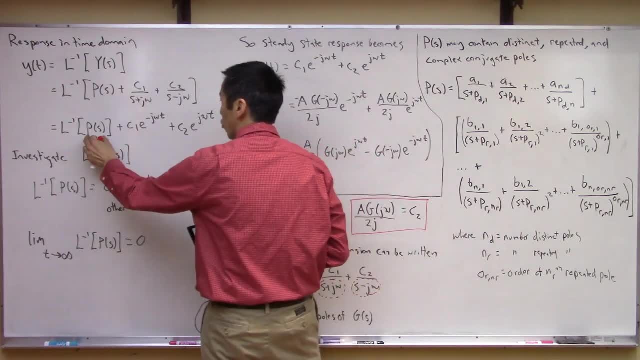 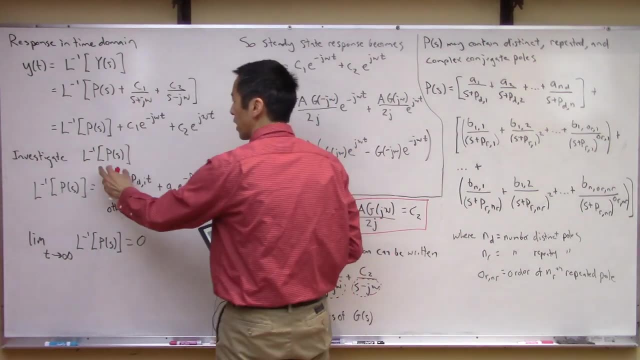 ugly thing over here. right, it could be very, very complicated, so we're just going to leave this as Laplace, the inverse, Laplace transform of that ugly thing. right, let's take a closer look at that. right, let's take a look at the look at the. 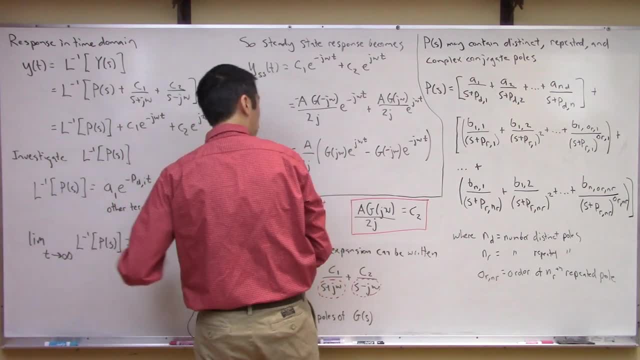 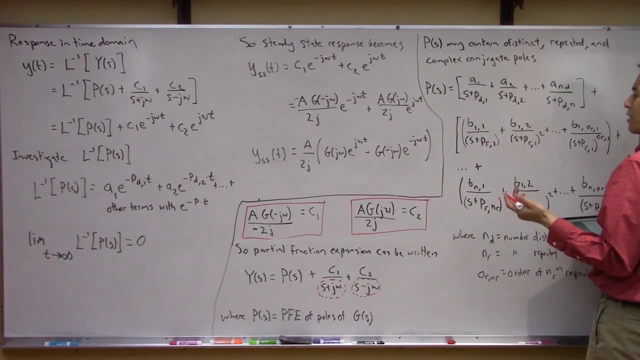 ugly thing, right? so it's just the inverse Laplace transform of this gobbledygook, right? so, in other words, i got to take the inverse Laplace transform of each one of these terms, kind of one at a time, right? so tell you what? let's look at this one right here. right? this is nothing more than a1. 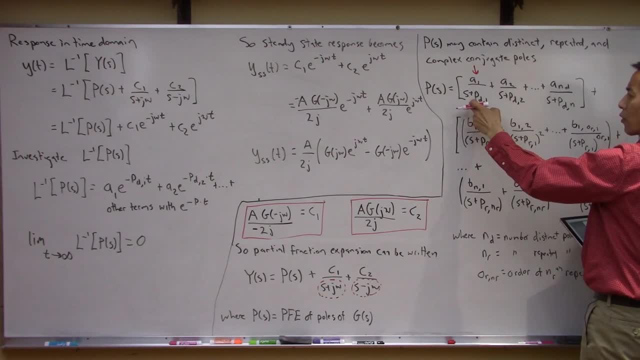 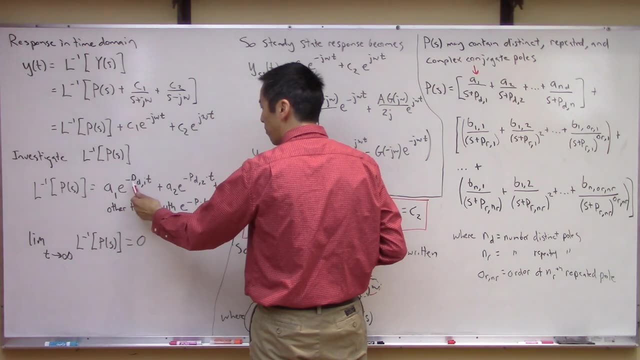 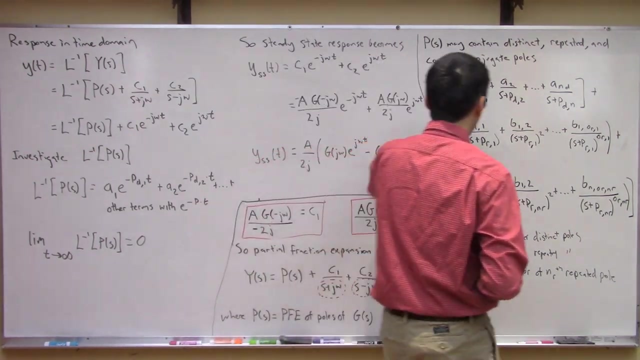 over distinct pole, right, it's a1 over s plus pd1, right, so the inverse Laplace transform of this term. it's just going to be this: right, it's a1 e to the minus pd1, i guess. right, that should be a sorry, one times t, right, and then, okay, do this term right, same thing. you get this a2 times e to the. 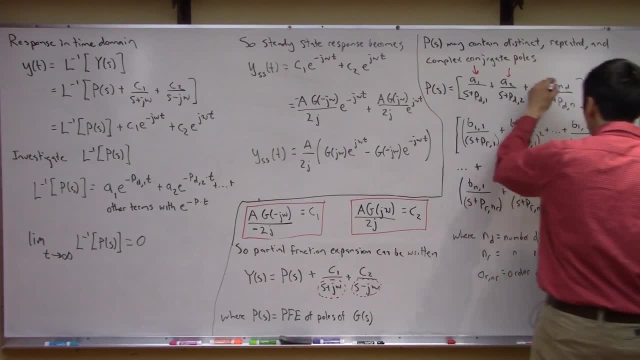 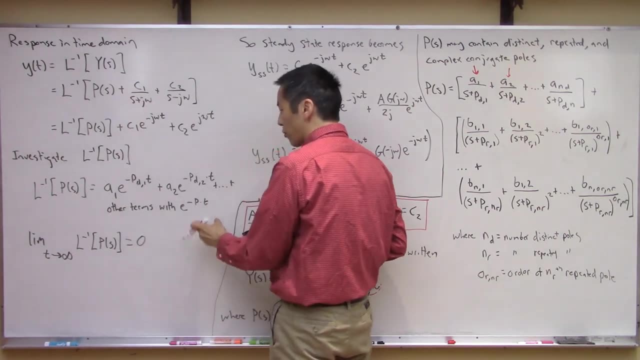 negative pd2 times t, etc, etc. right, you can do each one of these terms right, take their inverse, Laplace, transform, so you're going to have all this. but basically all these terms are going to be exponential decaying terms. right, because we had that restriction that the system is strictly. 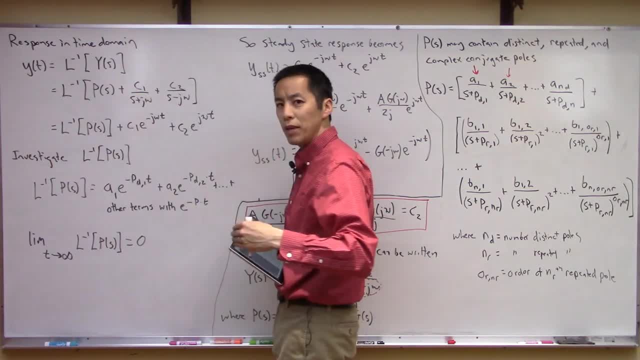 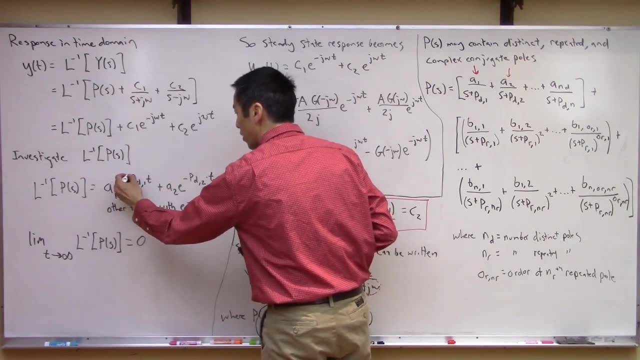 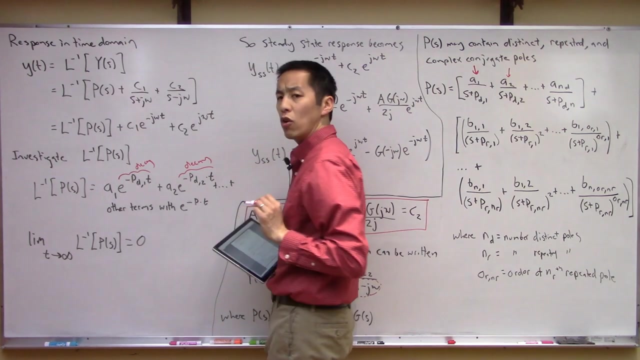 positive. we know all these p numbers are going to be strictly positive numbers, so that you have an e to the negative positive number times t. this term is going to be decaying right? so will this term. this will decay right. in fact, every single one of these terms are going to. 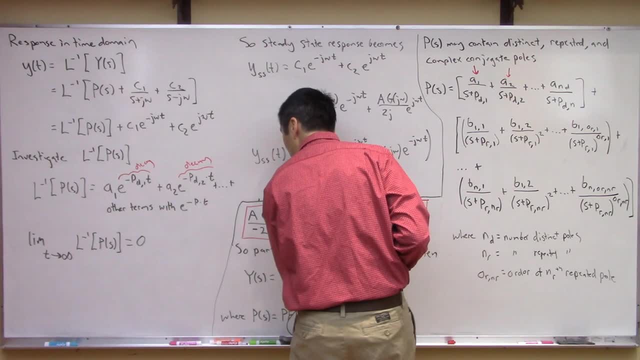 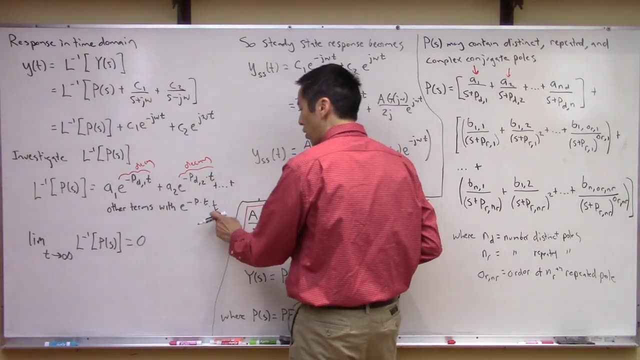 decay. sure, some of these terms might have a t in front of it, right, it might be this: exponential times t, right, for if you have a multiplicity of of order one, right, you'll have a t term. if it's a multiplicity of order two, you might have t squared or t cubed, right, everyone gets what i'm. 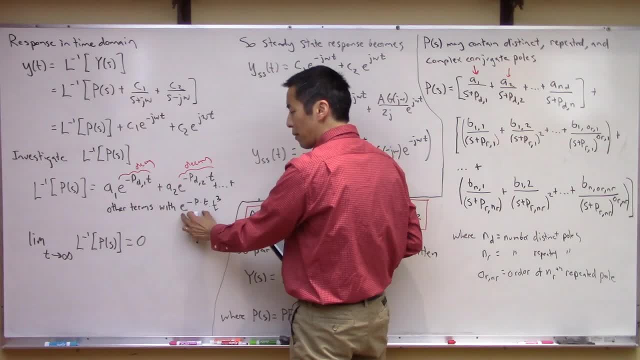 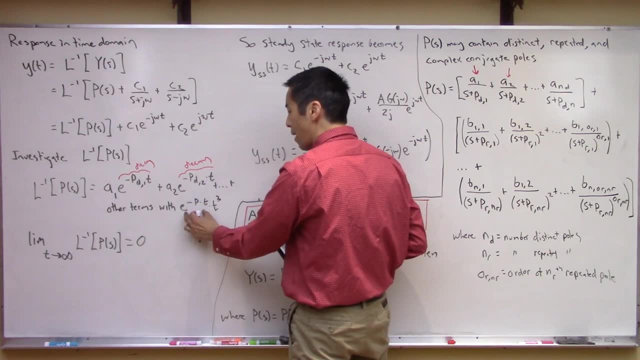 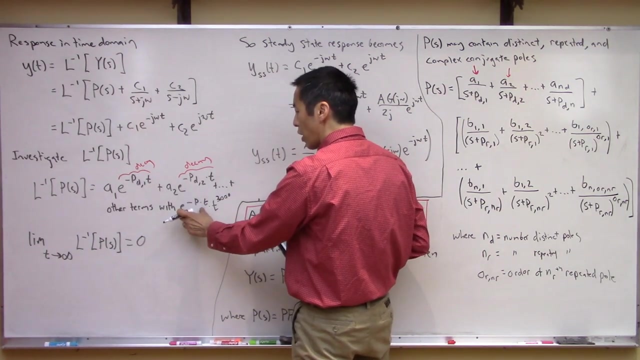 saying: right, you might have this, but you're going to have it multiplied with an exponent. uh, that's decaying. and since this is of exponential order, we know that, no matter what, i don't care if this is like t to the 300 or 3000, right, this exponential, no matter how slow it is, it will eventually squash this. 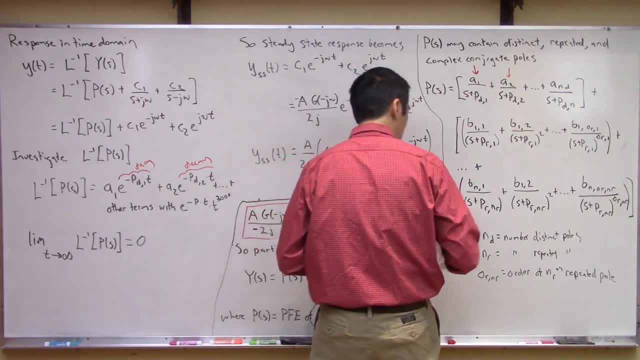 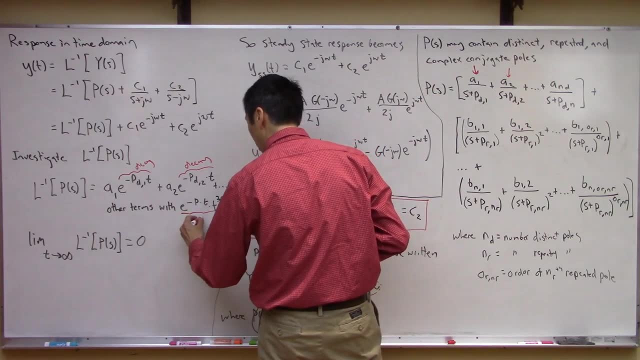 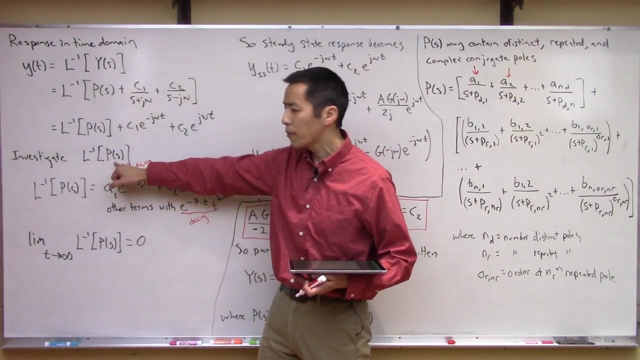 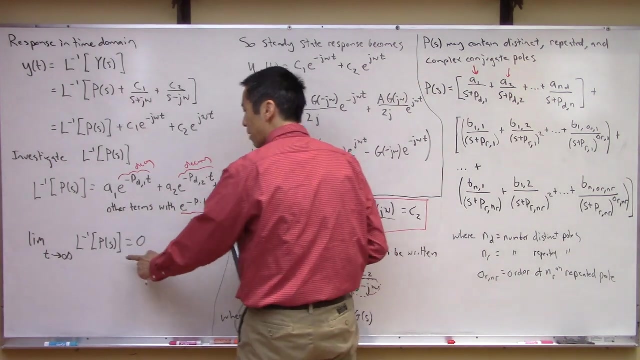 growing term, meaning also all these repeated parts, right, any of these repeats, i don't care how repeated they are, this thing will also decay, right? so aha, this is fascinating. every single term in this inverse laplace transform of p of s, it's going to decay. it might take a while to do it, but it will decay. so, in other words, i can think about. 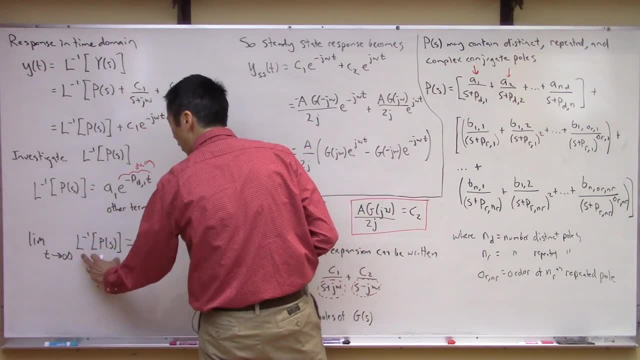 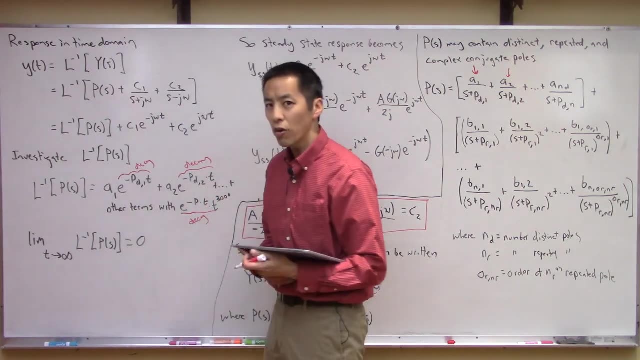 this and say, okay, the limit, as time goes to infinity, of the inverse laplace transform of p of s, that's just going to be zero, right? so if what i care about now is, instead of looking at the actual response y of t for all time, what about the actual response y of t for all time? what about the? 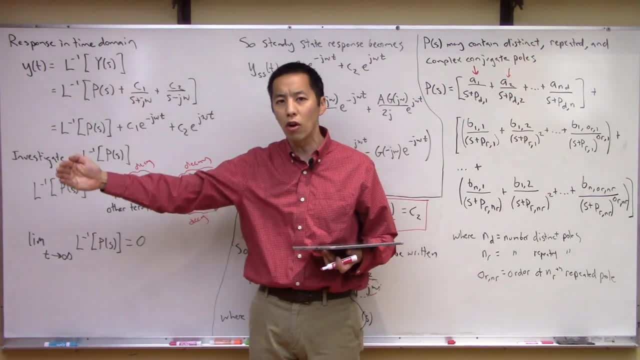 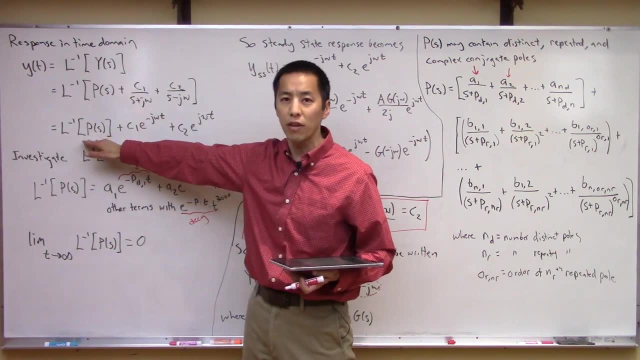 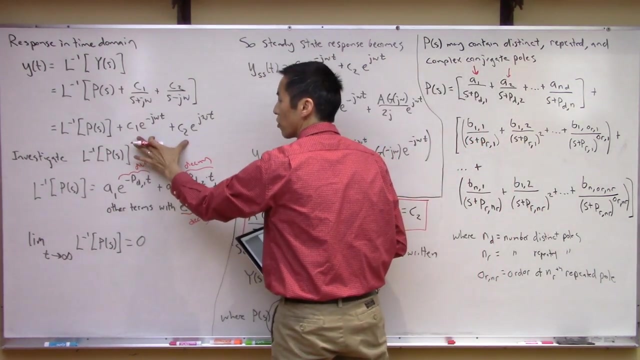 nope. what about tance? right? so when i only look at the steady state response when t becomes large, right, when t becomes large, i can use this fact to basically knock out the ugly bits of this equation, right? so, in other words, the steady state response, it's just these two terms, right? 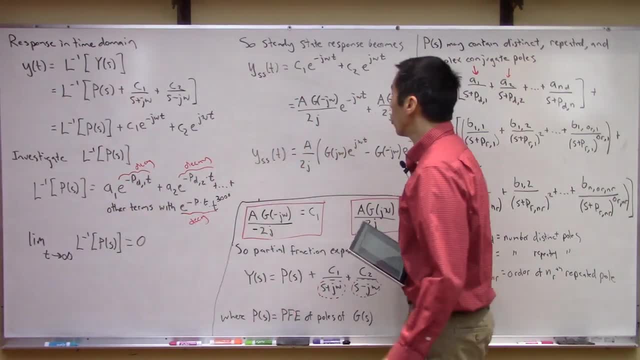 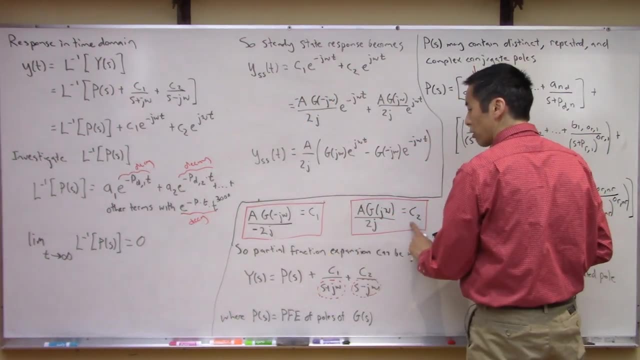 because the that other junk is gone. so we only end up with this right, and we know what c1 and c2 are. we just solved for them earlier, so just plug it in for c1 and c2 for the rest of those. that's what we've got right here, okay, And now I'll just simplify that a little and we end up. 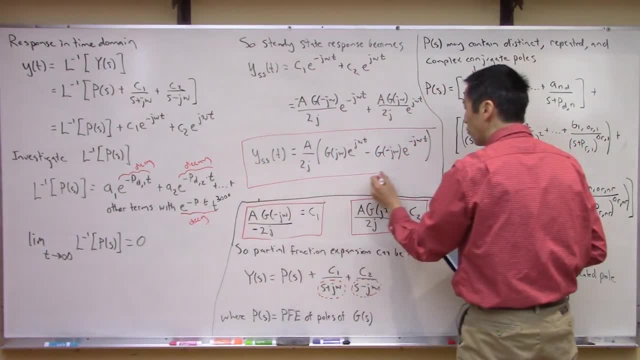 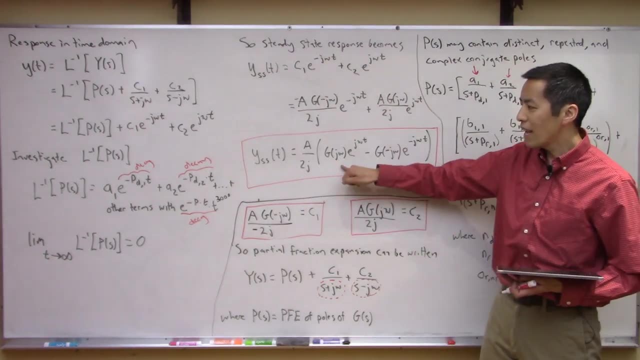 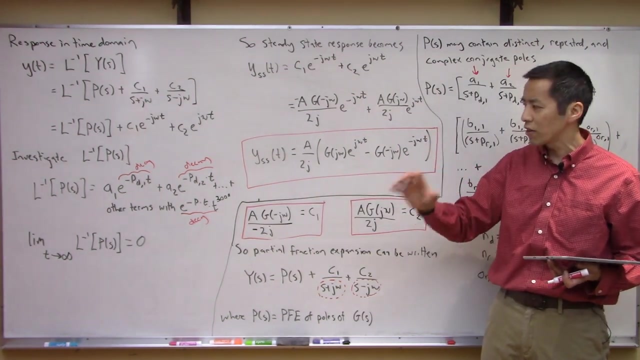 with this. This is beautiful, elegant, but maybe not the easiest thing to interpret right now. right, What this is saying is? this is the steady state response of any linear, strictly stable system in response to a sine wave of the form A, sine, omega, t, right. The only problem is: 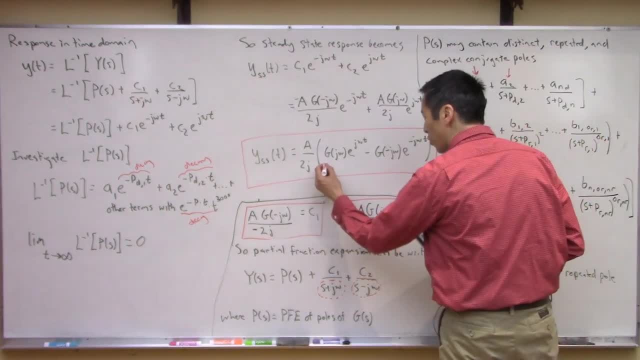 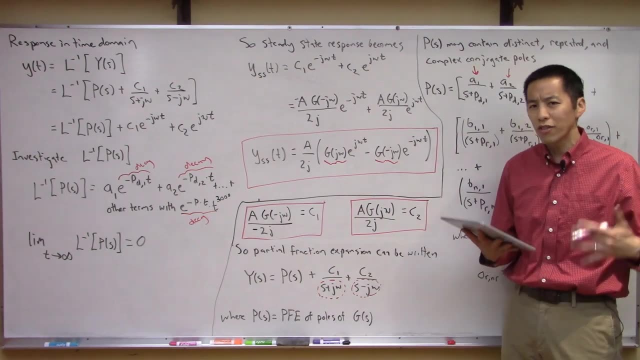 if you look right, we've got to understand what is this term here- G of j omega- and what is this term G of negative j omega. There's two terms in here which, as you can probably imagine, have something, actually a lot, to do with what the original plant model was. So that's what we. 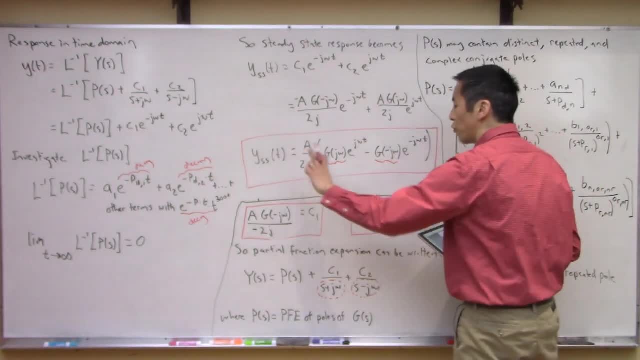 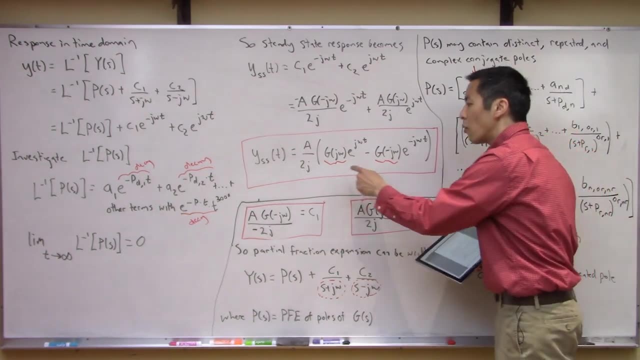 need to do now. We did all this work to get to this beautiful equation, but I don't know. this doesn't look like. I don't think I could plot this right now or have a good understanding of what this is doing. right, We need to examine these two terms, So. 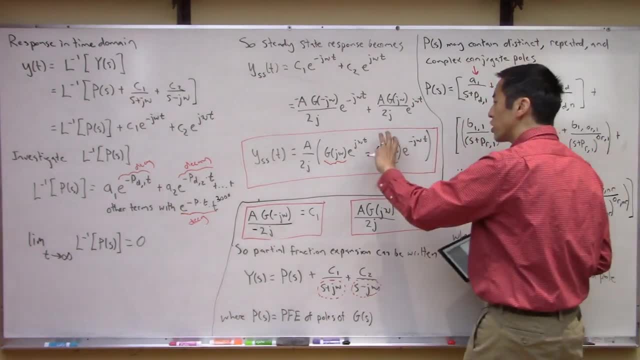 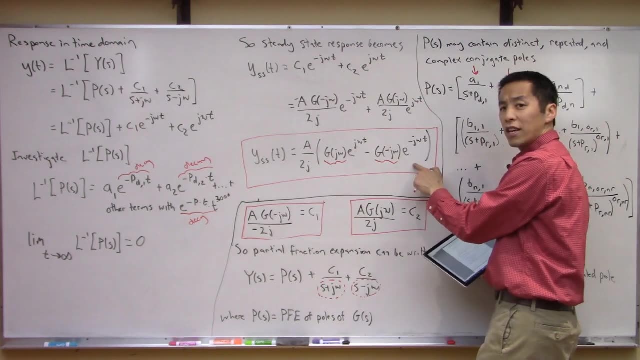 now I think we can safely erase the entire board. We will just save this, move that over to the corner or something like that, because this is the thing we want to work out and get an understanding of what is the steady state response of this system. What is this trying to tell us? All right, 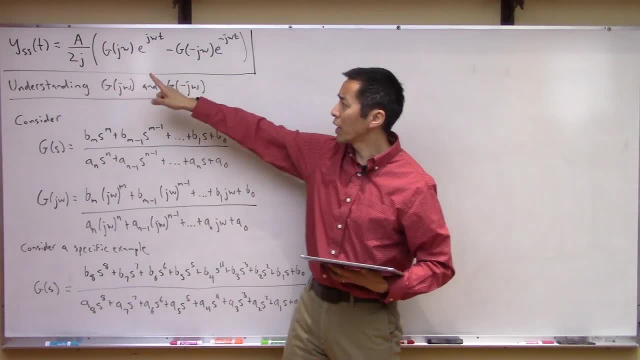 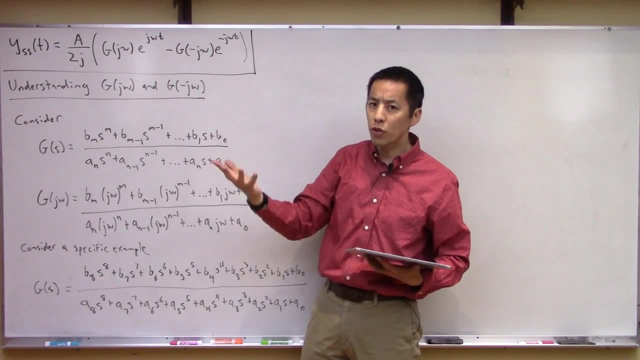 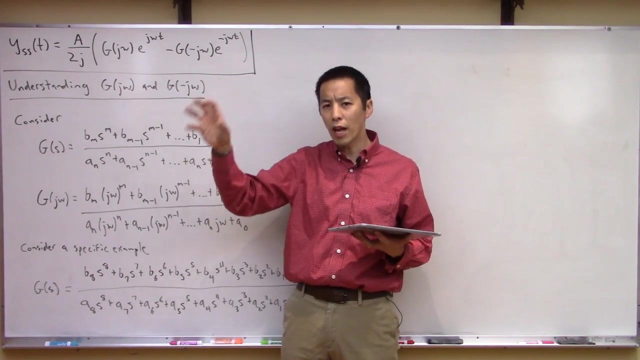 so I've saved our critical equation and now what we again want to do is understand this term: G of j omega and G of negative j omega. okay, So to do that, let's go ahead and consider our transfer equation. So, instead of having it written, as you know, S plus Z1, S plus Z2, all the way up to S. 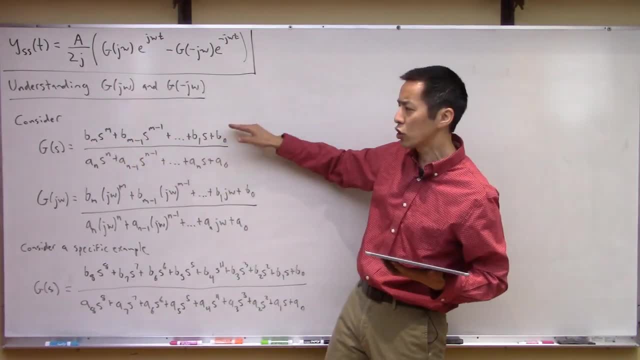 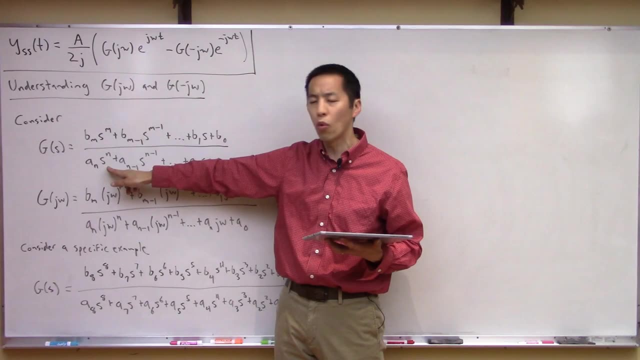 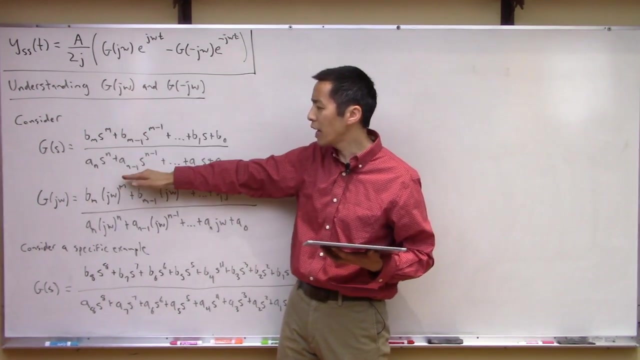 plus Zm. let's just expand it all and in the numerator we'll just have a nth order polynomial in S, and same thing. we'll expand the denominator poles out to an nth order polynomial in S, right, Okay? so all we're talking about with this term- G of j, omega- is you take G of S. 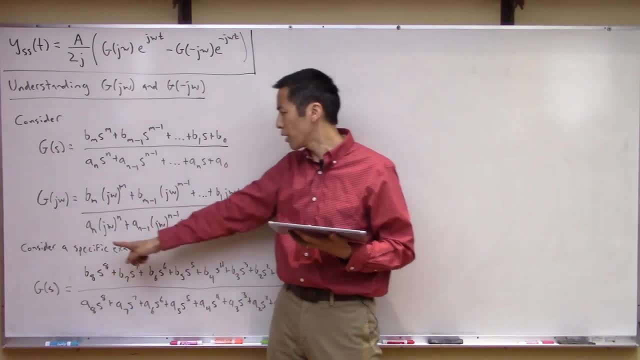 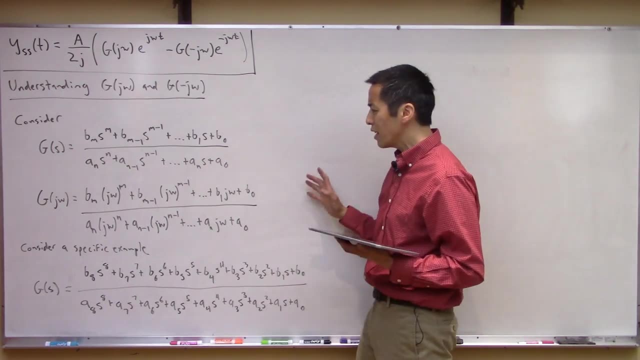 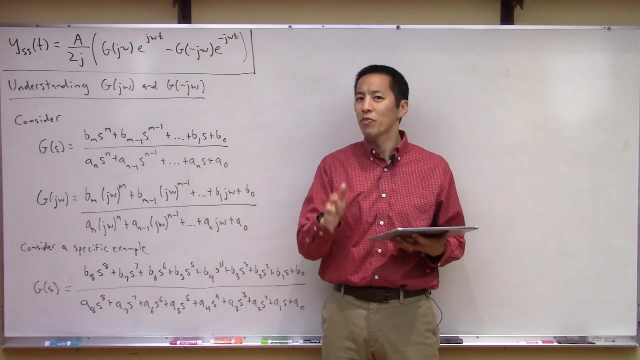 and everywhere you see an S, you plug in j omega, right. So j omega goes in everywhere, right, Okay, so now to gain a little bit of insight, I think the easiest thing to do is let's actually look at a specific example. Now, I am going to freely admit right now that the next 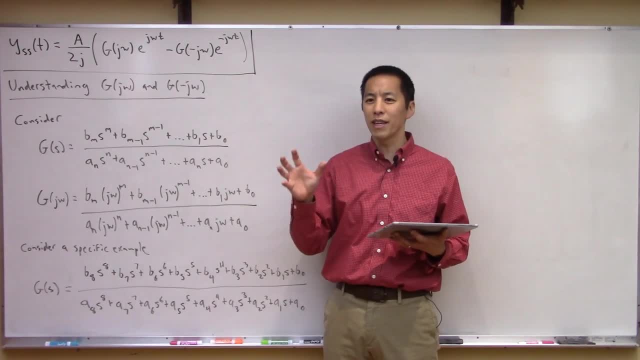 several minutes of this discussion might seem a little bit too much of the nitty-gritty and in the weeds. So if you want to skip all of this derivation and just get to the results, feel free to jump ahead to the end of this section of the video. I just want to go ahead and put it all. 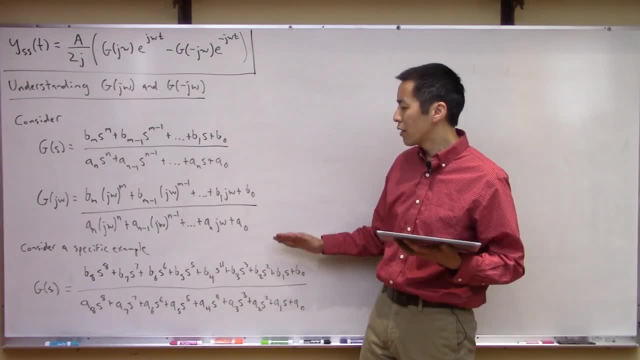 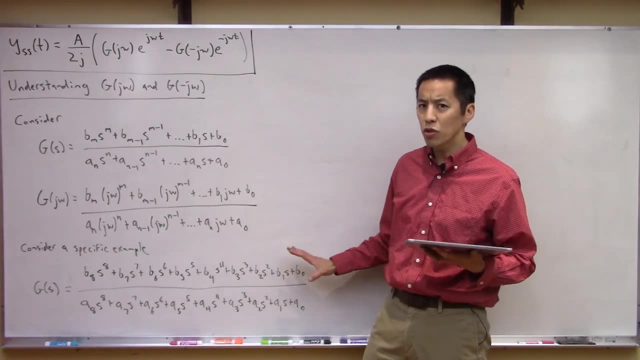 together for the sake of completeness. So what I want to do now is let's go and look at a nitty-gritty example to gain some insight into how this term behaves. So, again, let's introduce it here on the board and actually, you know, what might even be better is let's actually jump over to. 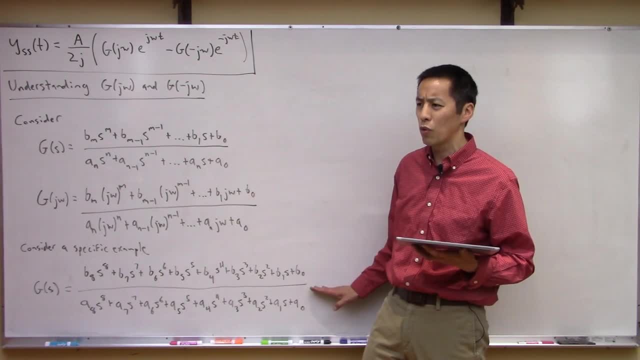 Mathematica, because there's a lot of notation and I don't actually want to write it all here on the board, since I've already written it down in Mathematica. So tell you what, like I said, now might be a good time to either take a nap and zone out for a couple of minutes. 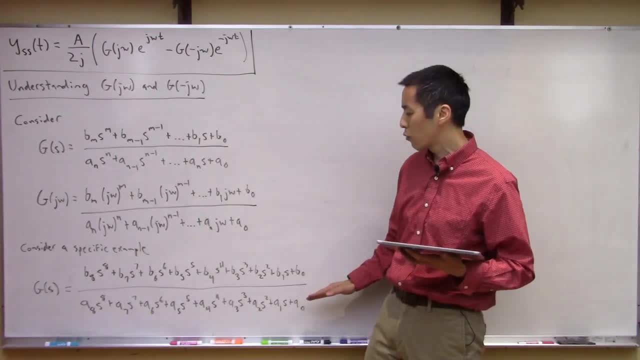 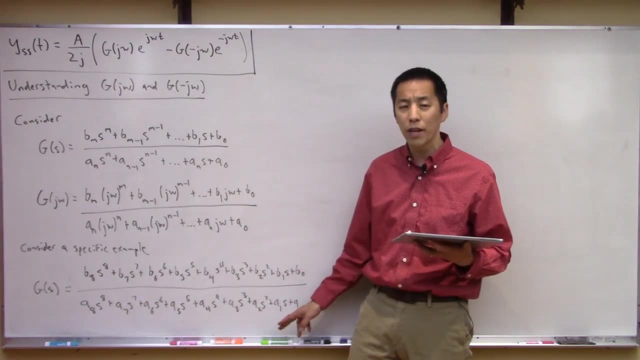 or, if you're interested, let's go over to Mathematica and work out this example of: let's consider an eighth-order polynomial in the numerator and an eighth-order polynomial in the denominator and let's just see what happens if we just work this through a couple more steps. 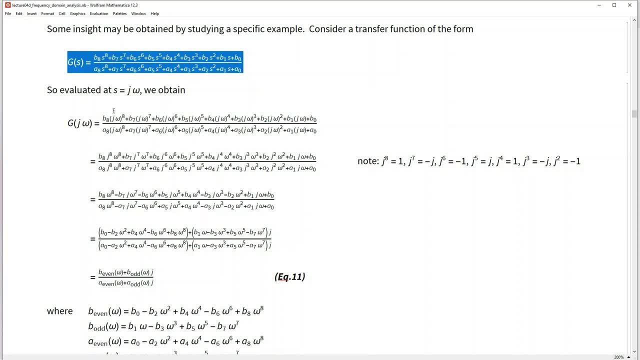 All right, so here we are in Mathematica, and again here's the example I want to look at, this eighth-order polynomial. So what we're going to do here, and you can kind of see why I didn't want to write this all on the board. there's a lot of kind of repetitive calculations. 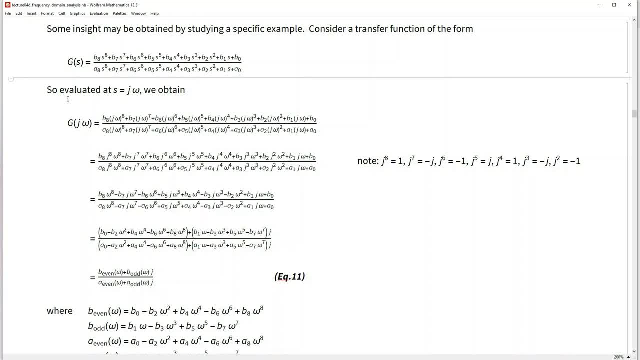 again. I just want to put it up here. feel free to pause the video if I go too fast and if you really care about it, but I really think this is probably one of these things where maybe one percent of the people actually want to actually see it. but I want to put it out here for 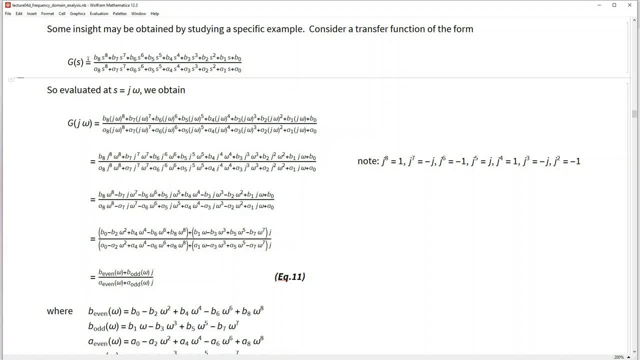 the sake of completeness. So, again, all we're going to do here is we want to understand what does this term look like when you evaluate it at s equals j omega. okay, So that's basically take the transfer function everywhere you see s sticking j omega, right, So you basically get. 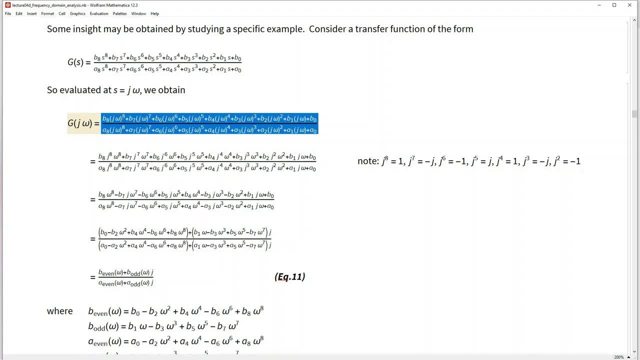 this, right Now, you can distribute these powers, these exponents, through to both the j and the omega term. that's what you get down here, right? And now we can make the interesting observation that, well, okay, what is j squared? j squared is just negative one, right? What's j? 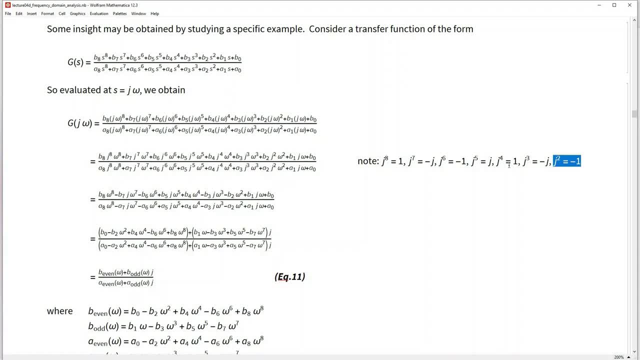 cubed. Well, that's just negative j j to the fourth is then just one, so, etc, etc. right, You can see how there's a pattern going on with j's raised to successive exponents. right, You get this pattern of basically negative, negative j, one j, negative, one negative j, right, And 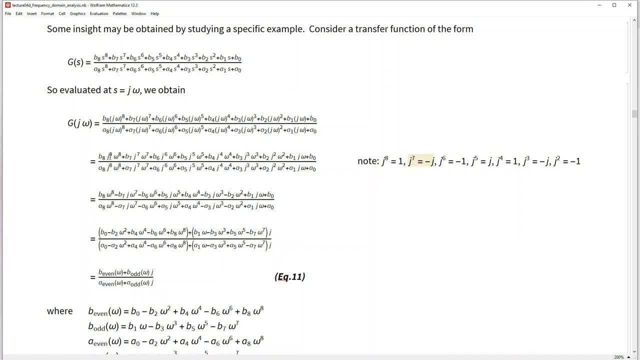 etc, etc. it repeats over and over, right? So basically I can replace all of these j's to exponents or these imaginary numbers to exponents with smaller, lower order terms, right? So you would get something like this: 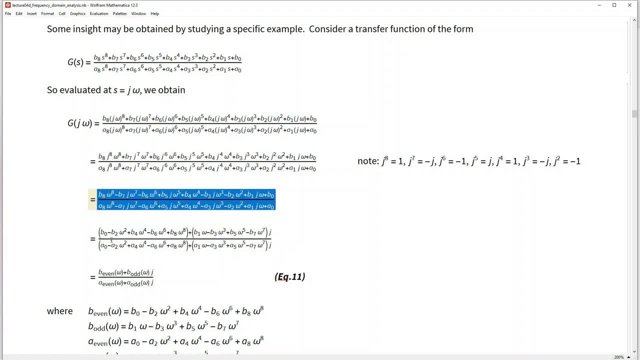 okay, Now what I'm going to do is let's go ahead and collect all of these so-called even coefficients, or even powers of omega. right, So this is omega to the zero, omega squared, omega fourth, omega six, omega eight, etc. right, So here's all of the even powers of omega. 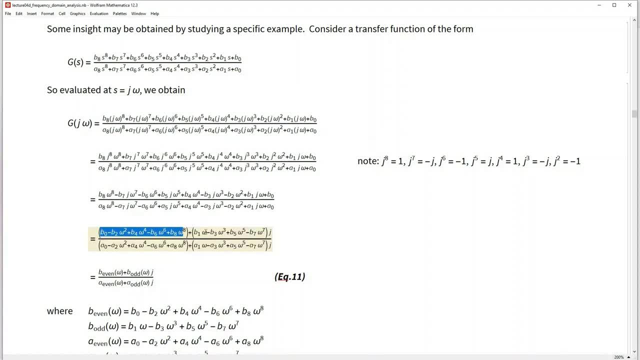 whoops, sorry, The numerator same thing. let's collect all of the odd powers of omega here and you notice what's interesting is all of these odd powers, those are the ones that are that have an associated imaginary term associated with them, right? So all these odd ones are where there? 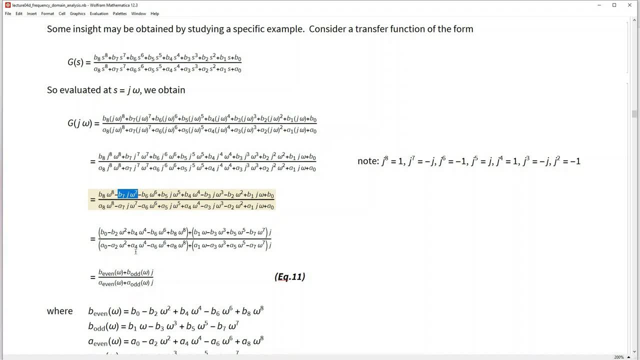 still are imaginary terms, right, So you can do that for the numerator and the denominator. So, at the end of the day, what we end up with is: let's call this entire polynomial, just be even. and let's call this entire polynomial here. 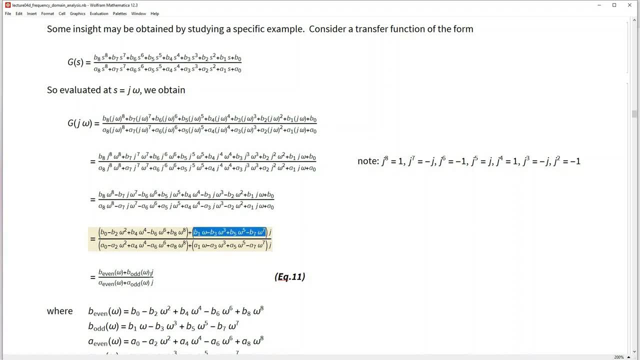 be odd. and all these are both functions of omega, right? So all I've done here is, if you see, it's just basically writing this again. it's just a complex number. we're just collecting terms and shuffling them as even, as either even or odd terms. So again, 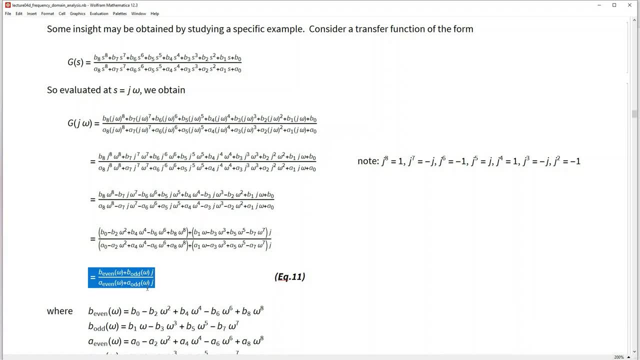 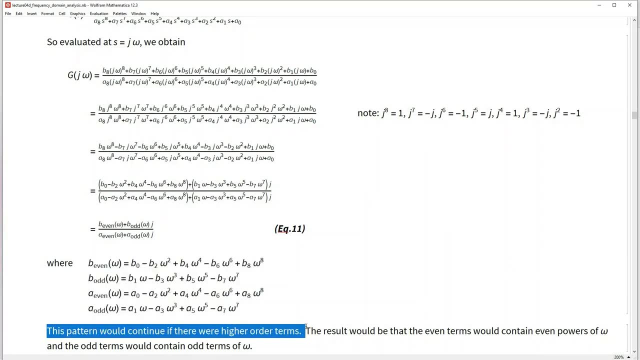 this is just algebra, right? So we get to this term with just plain old algebra, and this is what each one of these even and odd terms are. and we notice that this pattern would continue, no matter how many orders you know, if it's eight, sixteen, sixteen, sixteen, sixteen, sixteen. 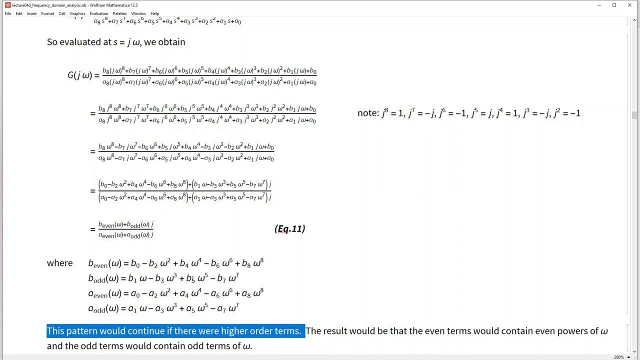 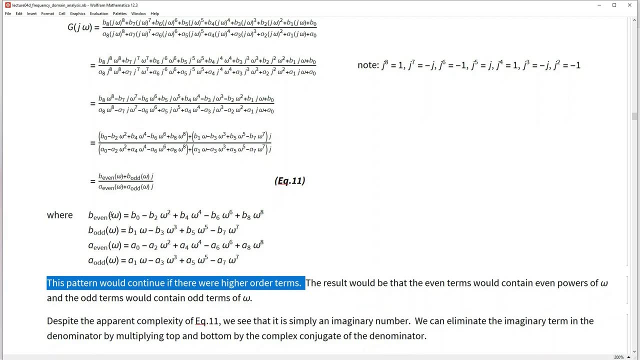 a hundredth order, you would just see more terms collected in the even or odd side, right. So that's what we end up with Now, despite this apparent complexity- right, we see that really it's just an imaginary number, right? You look at the top and you see: oh, 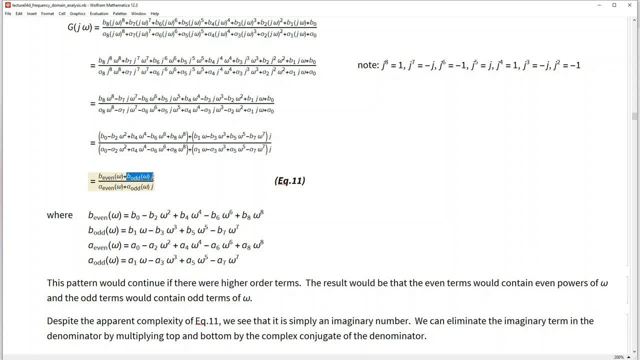 there's a real component here in the numerator and there's an imaginary component in the numerator. Same thing: there's a real component in the denominator and a real component in the denominator. So again, this is nothing more than an imaginary number, right? So if you look at the top and you see, oh, there's a real component in the. 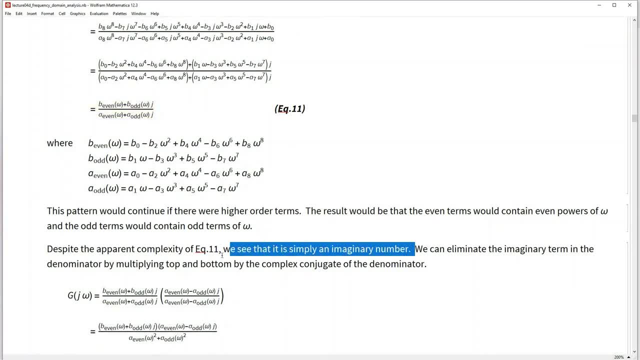 denominator. So if I want to eliminate the imaginary term in the denominator, we do that by just multiplying the top and bottom by the complex conjugate of the denominator right. So the complex conjugate of this denominator, it's just the real part minus the imaginary part right, which is this: 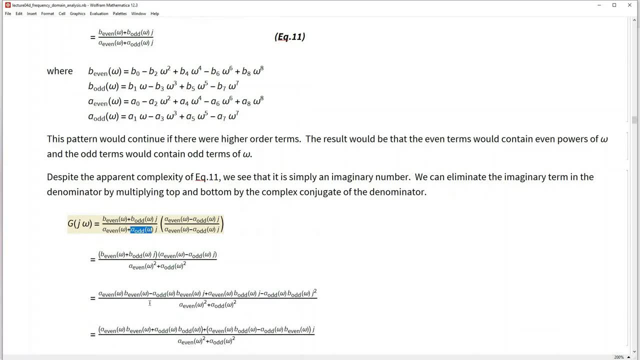 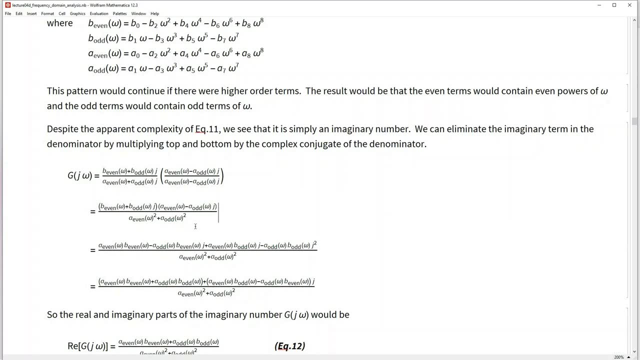 odd term, okay. So again, nothing fancy, it's just more algebra. So again, this is. I'm just going to scroll through this quickly. Feel free to pause the video. If you want to double check my algebra, feel free to go about that. but you see that it's just doing multiplication. 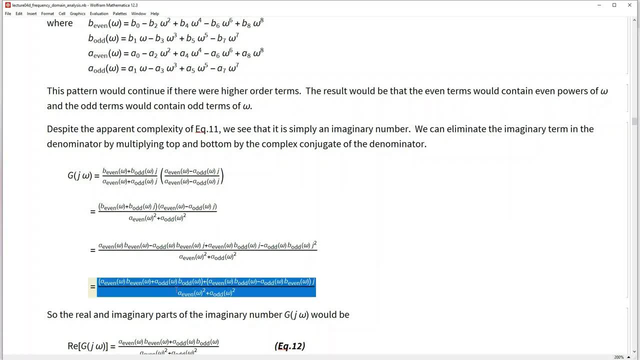 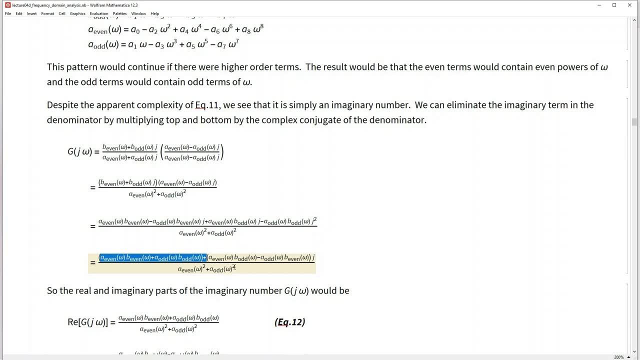 multiplication and we end up with this thing, right? So at the end of the day, you look at this thing and again you see that this term divided by this is basically the real part of this imaginary number g of j, omega, right. And then this part, oops, sorry, let me see if I can actually. 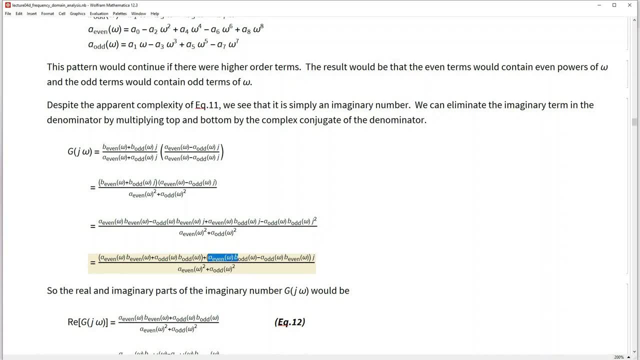 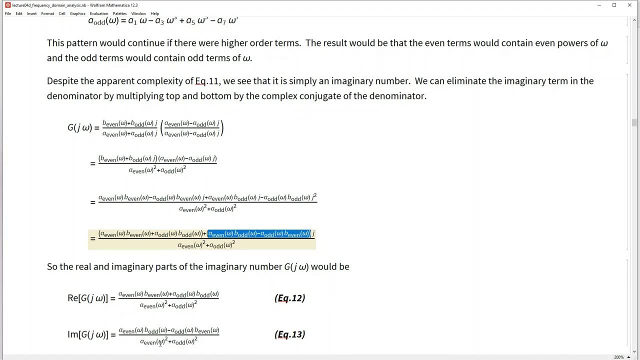 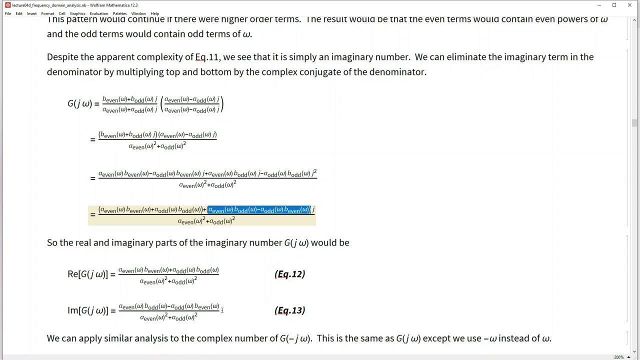 highlight this, I might have to use my keyboard because it's hard to get with the mouse. but this entire thing, right, the coefficient of j divided by the denominator, that's the imaginary part of this imaginary number g of j, omega, right? Okay, so that's great, We end up. 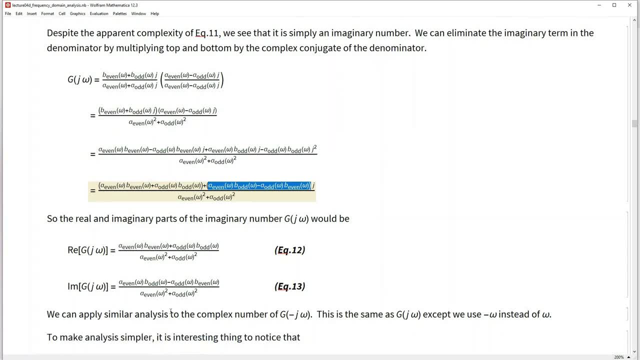 with this result. okay. So now let's do a very similar analysis, but instead of evaluating it at s equals j omega, let's evaluate it at s equals negative j omega. So again, it's the exact same thing. You can go through all of this analysis and basically just do the algebra, The thing that 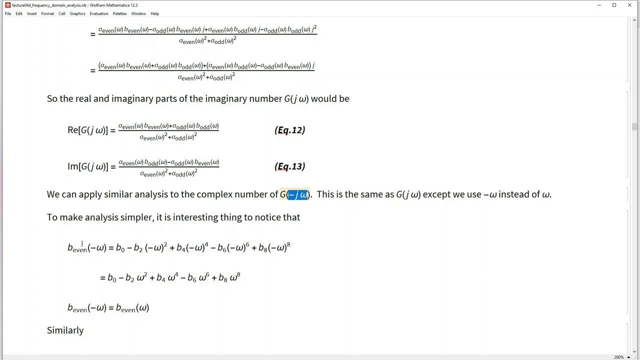 I noticed that. remember that even and odd term we had here B, even of negative omega. again, if you run through the math it has this property and again, this is sort of the definition of kind of an even function. I apologize, that's actually a bad naming collision here of even Tell you what. 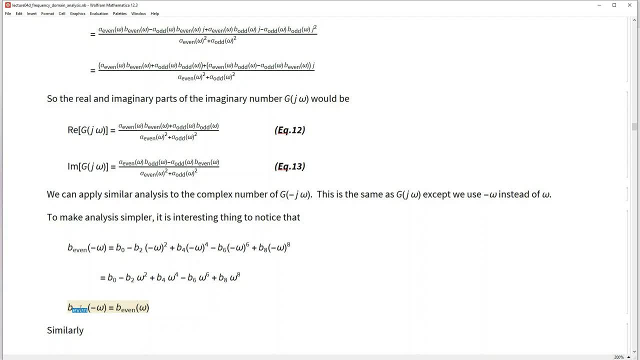 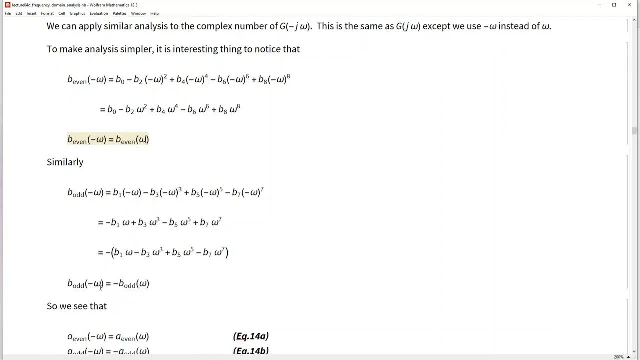 ignore the fact that I said that All we see is that b the even terms, if you stick in negative omega, it's the same thing as b of omega, whereas the odd term, if you stick in b odd, it's the same. 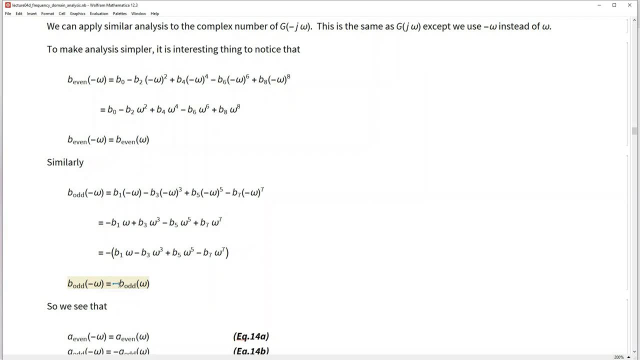 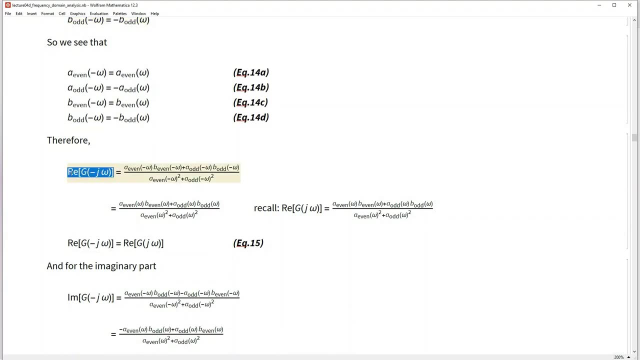 thing. So if you do that, what you would end up with is this here: if you follow the exact same process, this real part of g of j omega is going to be this: okay, And now, if you compare that with what we saw was the real part of g of j omega, you actually see that these are the exact 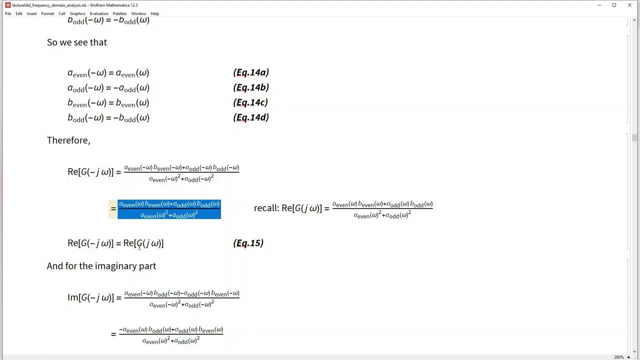 same terms. right, They are the same. So, in other words, at the end of the day, the real part of g of j omega is equal to the real part of g of positive j omega. So this is one of the key things that we 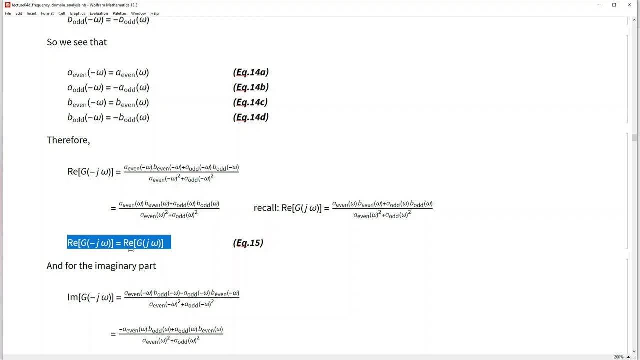 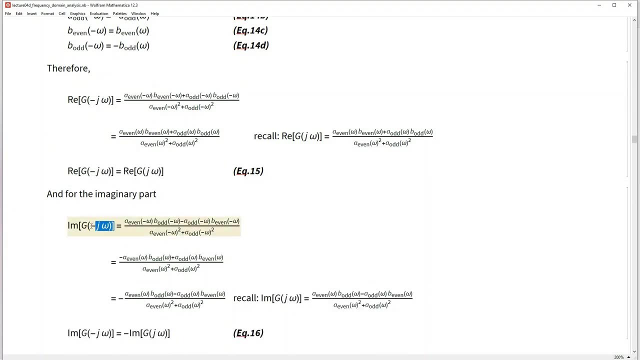 wanted to get out of all of that kind of boring algebra. that, I admit, is a little bit well, we rushed through it a little bit. right Now you do the exact same analysis for the imaginary part of g, of negative j, omega, and you end up with this term okay. And again, if you compare this: 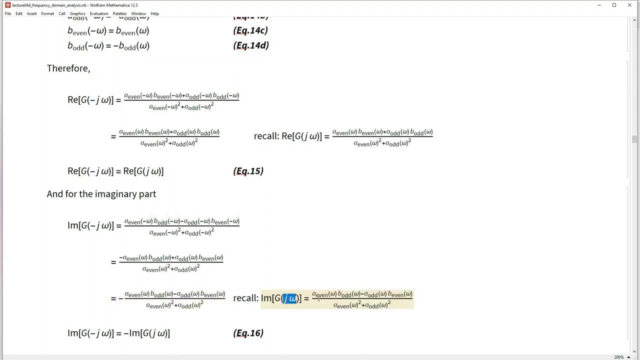 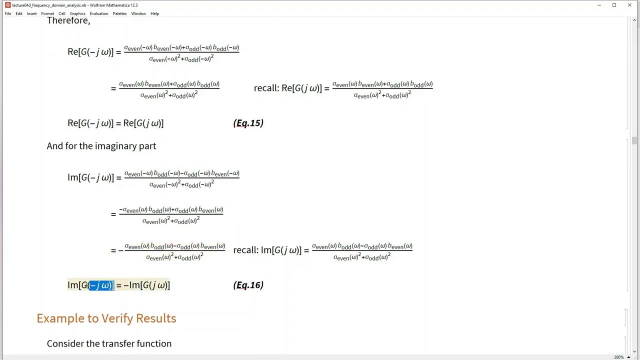 with what we got earlier for the imaginary part of g of positive j omega. you see the two things are identical. So if you compare this with what we got earlier for the imaginary part of g of negative j omega, you see the two things are identical except for this minus sign. So we end up with this. We end up with the imaginary part of g of negative j omega- is actually negative times, the imaginary part of g of j omega. So this and this- I don't know if I can highlight two. no, I can't highlight two things at the same time. but what I've labeled here is equation 15, and equation 16 is the result of all of this algebra and manipulation of the complex number. All right, so we've got that result. and while we've got Mathematica up, let's 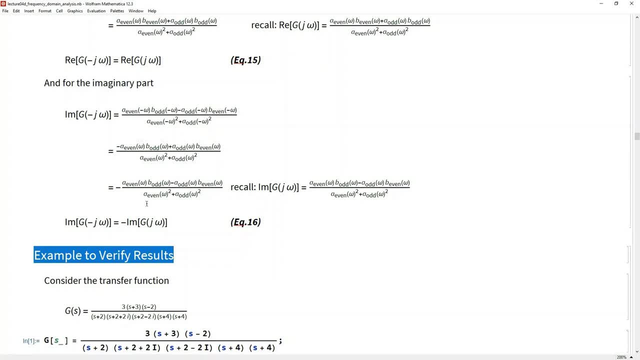 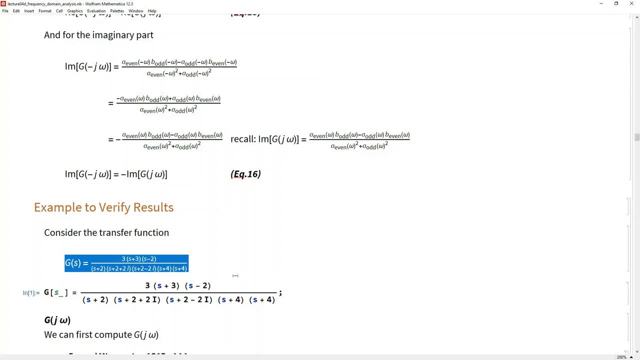 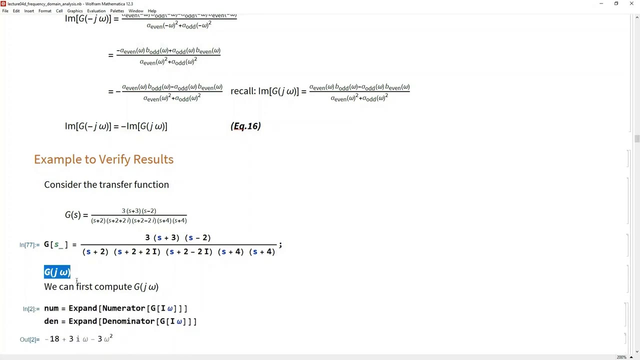 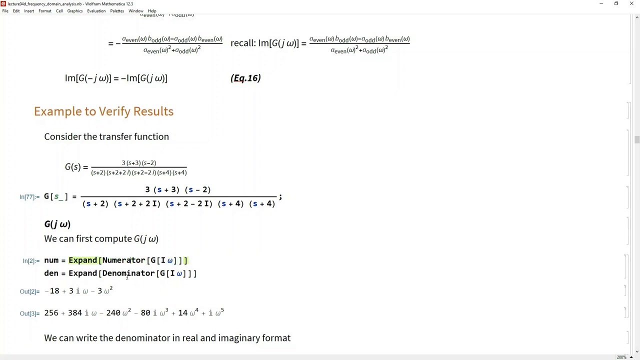 just go through an actual numerical example just to make sure that equation 15 and 16 check out. So let's try a concrete instantiation of some linear transfer function that looks like this, right? So let's go ahead and get this into Mathematica as g of s. okay, Now let's go ahead and compute g of j omega. So again, all that means is anywhere you see an s plug in j omega. So I'm just going to go ahead, do that. here. I'm going to split it up into a numerator and denominator, like such right. So here's what the numerator looks like. here's what the denominator looks like. 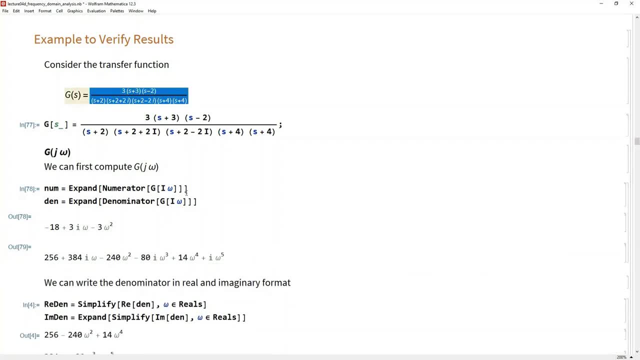 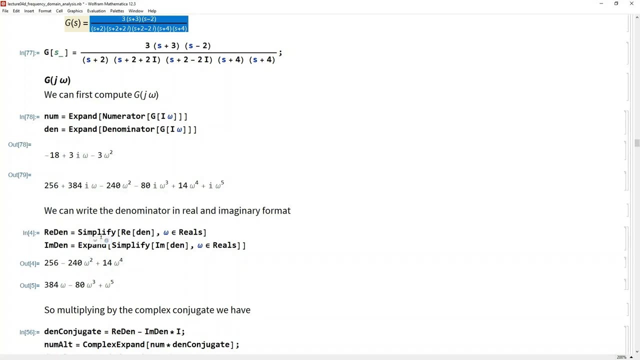 if you took this expression and everywhere you saw s substitute in the imaginary number times Omega. okay, now all I'm gonna do is I am going to try to do a couple of manipulations here to get this as just a real part plus a imaginary part, right? so I'm just gonna do a little bit of manipulation here and 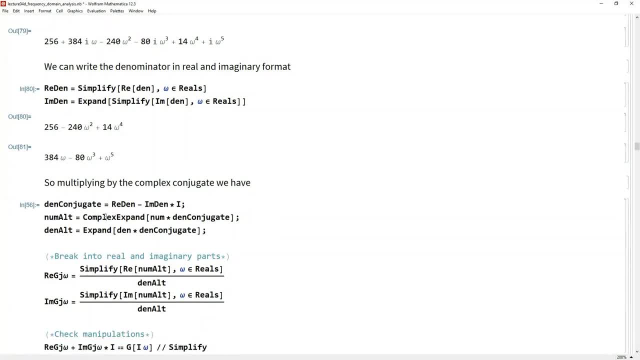 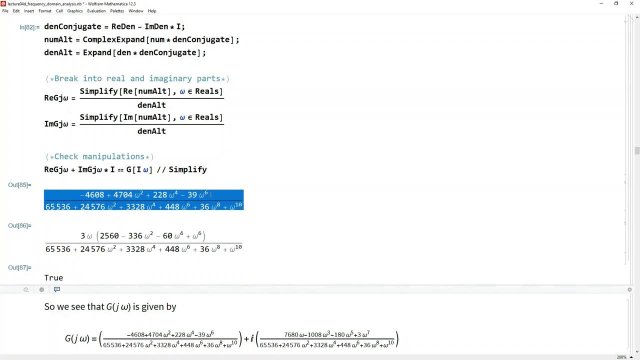 I'm gonna multiply the numerator, the denominator, by the complex conjugate to basically do a little bit more manipulation and okay, so we end up with this expression here. this is the real part of that imaginary number. here's the complex part of that imaginary number. and again, I'm just checking to make sure. 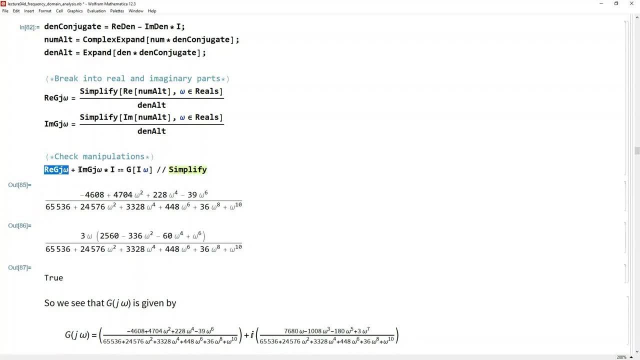 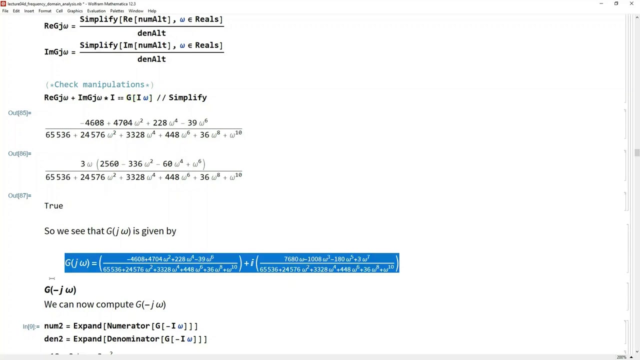 that I did my calculation correctly and that my real part plus the imaginary part times the imaginary number is the same thing as the original transfer function times J Omega or I Omega, however you want to think about it right. okay, so basically we see that, okay, G of G Omega looks like this. it's some ugly. 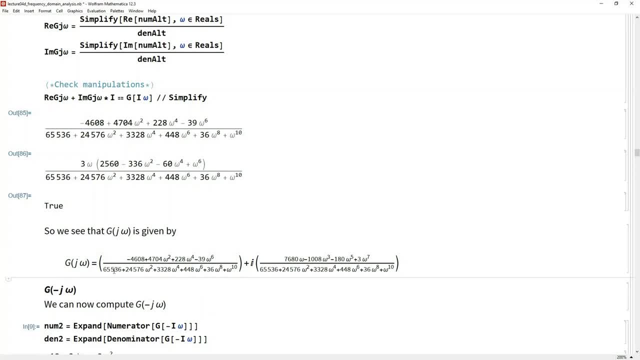 ugly, ugly expression, right, but at the end of the day, it is nothing more than a complex number where the real part is a function of Omega and the imaginary part is a function of Omega, right. okay, let's do the exact same thing with, now, G of minus J, Omega, right. so again, all I'm gonna do, I'm gonna run through the exact. 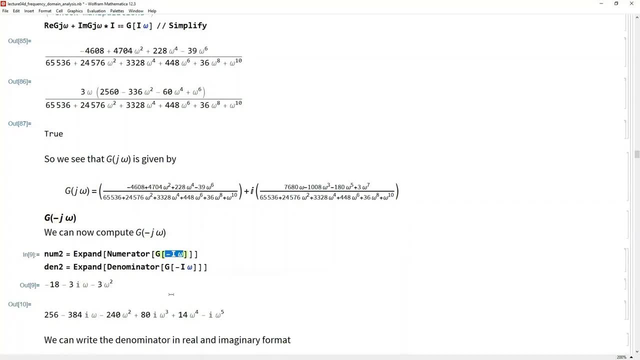 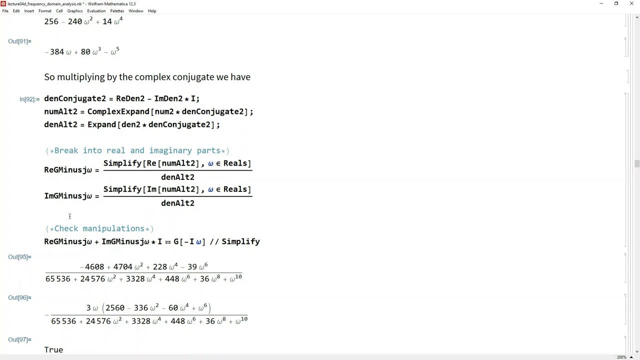 same operations, except everywhere I see an s, I'm gonna replace it with negative J, Omega, right? so let's go do that, let's do that, let's go ahead and go do this to basically get it into a form that looks like this: so this is what G of negative. 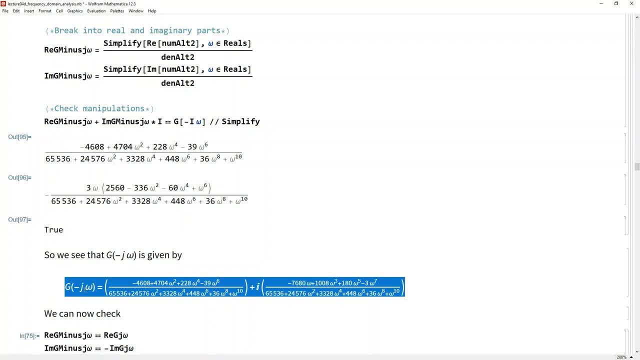 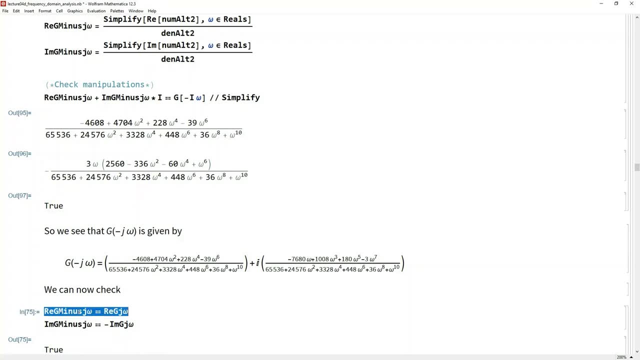 J Omega is right, and now I'm going to go ahead and check. make sure that equation 15 and 16 are true, meaning that the real part of g of negative j omega is the same thing as the real part of g of j omega and the imaginary part of g of minus j omega is negative imaginary part of g of j omega. 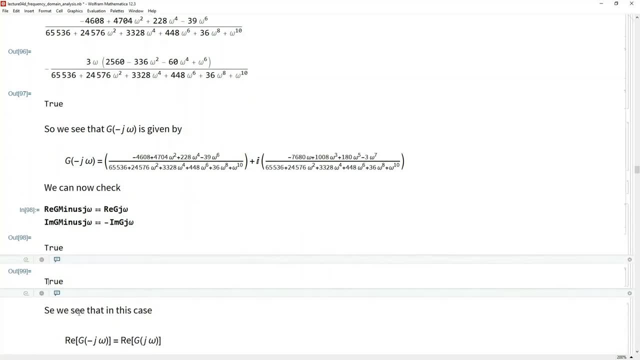 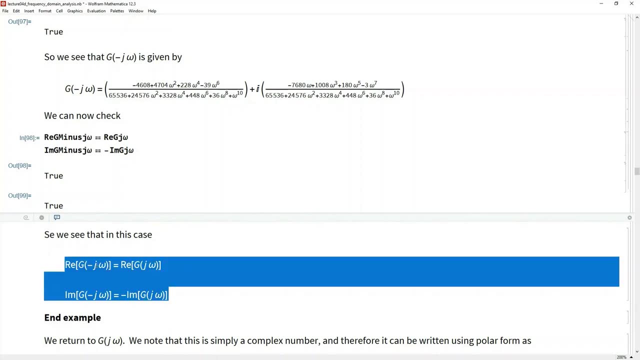 right there. so that's, and there we go. checks out, true and true. so again, in this one instance it worked out and again you can make the argument that this is going to work for any argument. so basically, here are equation 15 and 16. again, this is what we want to take to the bank and take it. 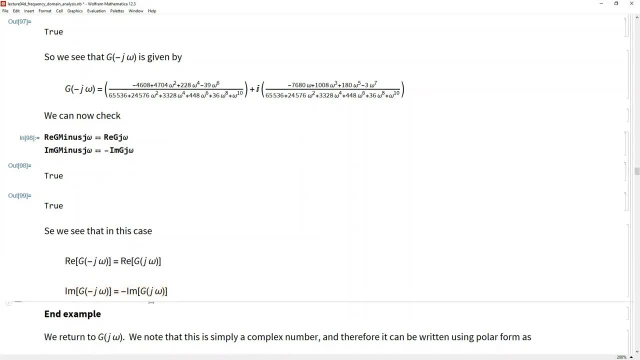 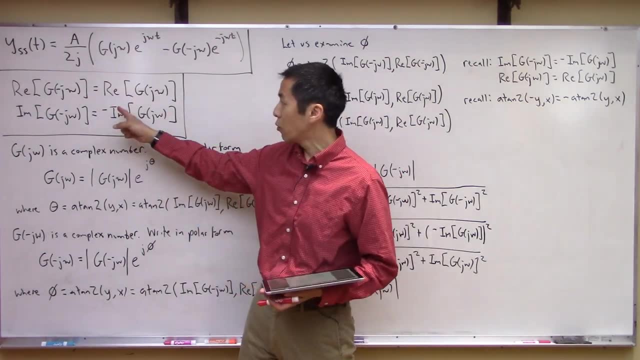 back to the blackboard and we will go ahead and use this now to better understand the frequency response of this linear system. all right, so thanks for sticking with me through that to basically we ended up with this right. this was what we went through all that algebra for, to just figure out. 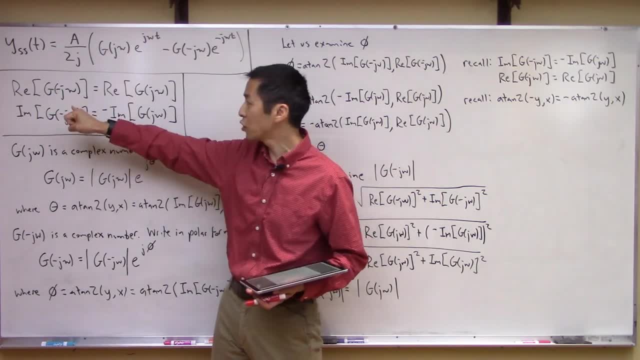 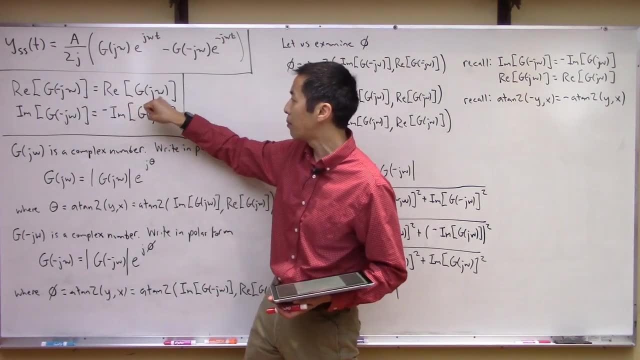 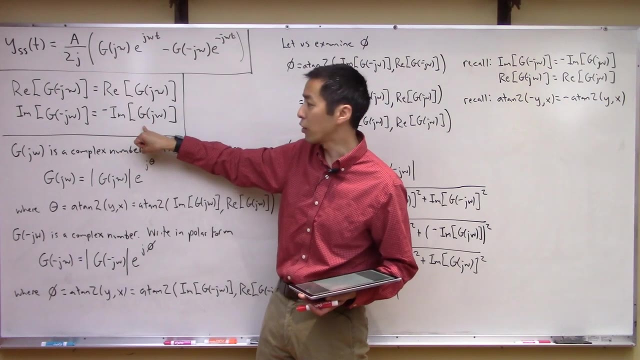 that for this linear transfer function. it has a nice feature that the real part of the negative, or g of negative j omega is the same thing as real part of g of positive j omega, and the imaginary part of g of negative j omega is negative, the imaginary part of g of j omega. okay, so again i 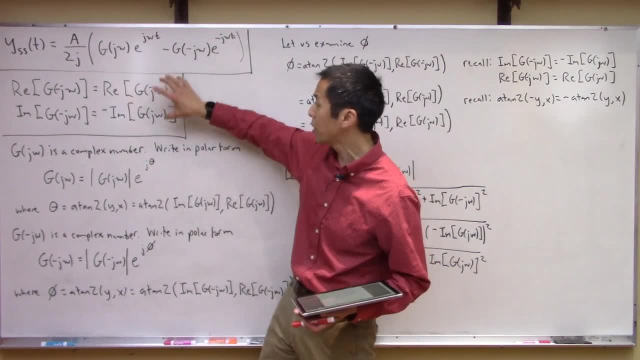 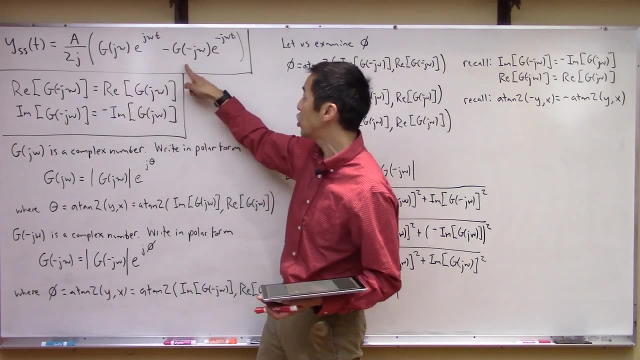 put this underneath, underneath our other important equation, right, because we now want to see: how does this help us? right? remember, we're gunning for this thing g of j omega and g of negative j omega. we want to have some better understanding of it. this was the first step, okay, so now let's go and 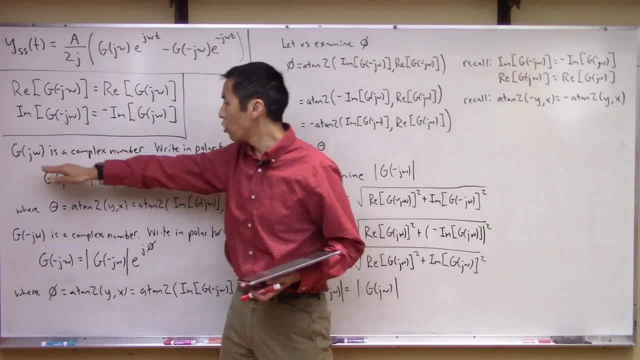 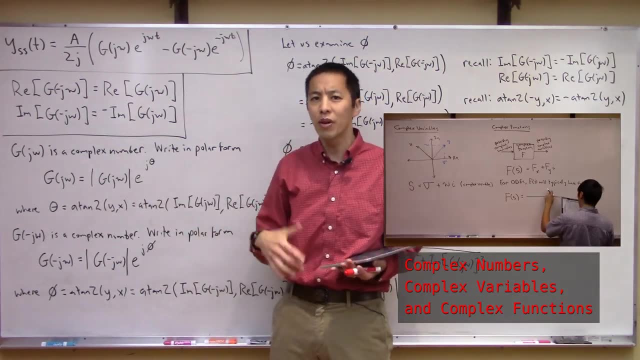 directly attack this term here: g of j, omega, right? so, as we've seen, g of j, omega it's nothing more than just a complex number, right? so tell you what, if it's just a complex number, instead of writing it in um, car you know rectangular cartesian form, where we look at the real part in the imaginary? 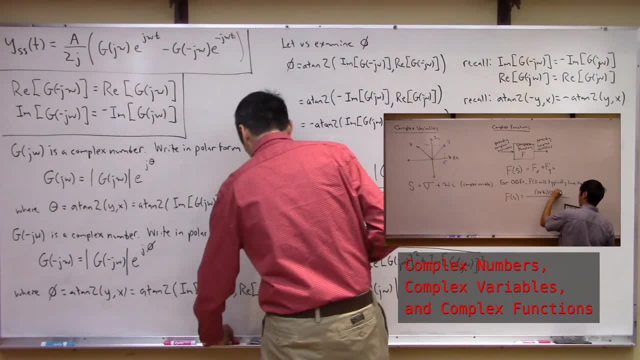 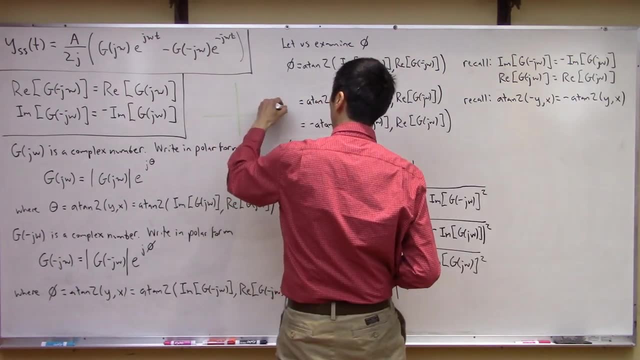 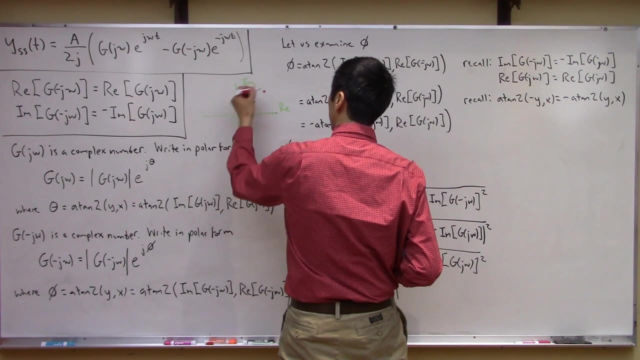 part. why don't we write this thing in polar form, right? so remember, just to refresh your memory, maybe i'll just draw a quick picture, right? the idea was, you know, if you have a real and imaginary right and you've got some vector out here like such right, um, and it has a real part and it has an imaginary part of this complex. 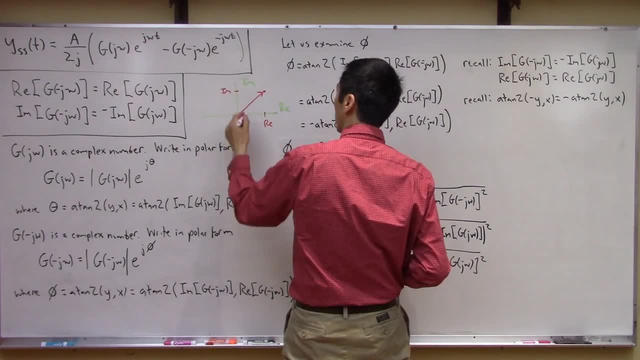 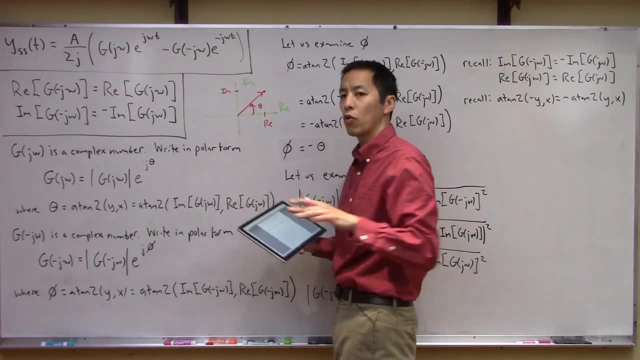 number, right? you can think about this as a vector, like such, where this vector has a magnitude and it has an angle- let's call it theta- associated with it, right? so this is the, the, the, you know, quote unquote polar form of the complex number. and again, we've got a dedicated video on complex numbers. if 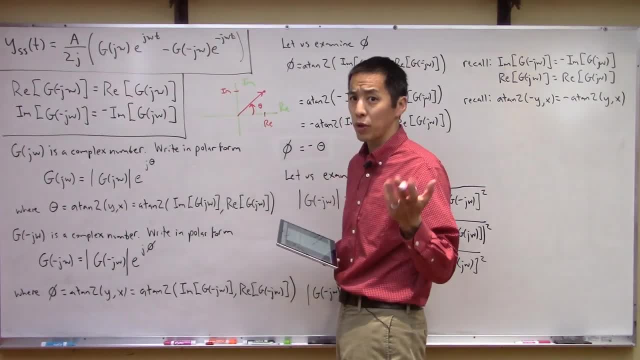 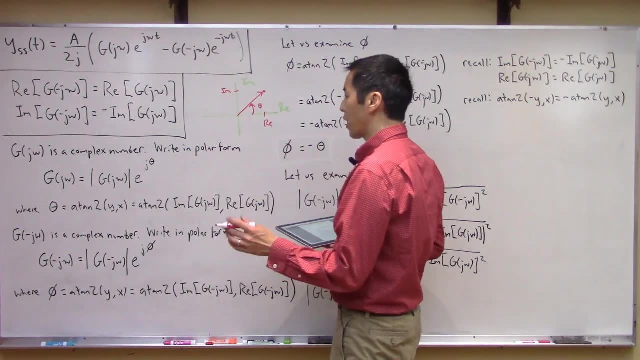 you want to refresh your memory on this um and some other properties that actually we're gonna we're gonna leverage later, so i would recommend checking out this complex number video if you haven't already seen this. so, um, assuming we're all okay with that, we can write. 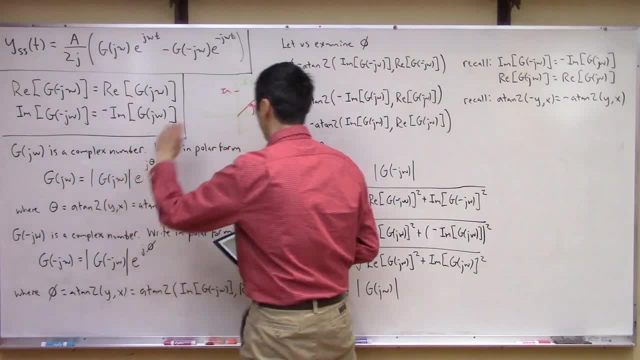 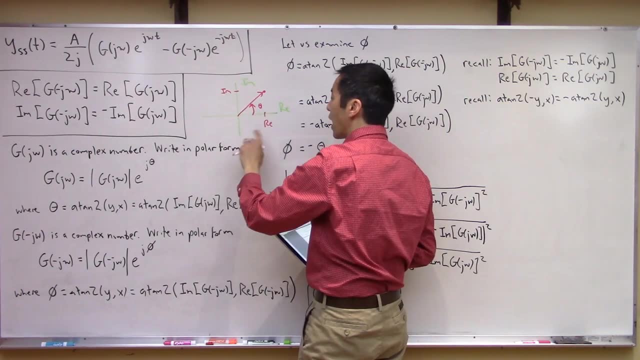 this thing as again it's just the magnitude of the complex number. right it's this length times e to the j theta, where theta is this angle associated with the, the vector right, and again this angle, you can see it's just given by basically the four quadrant inverse tangent. 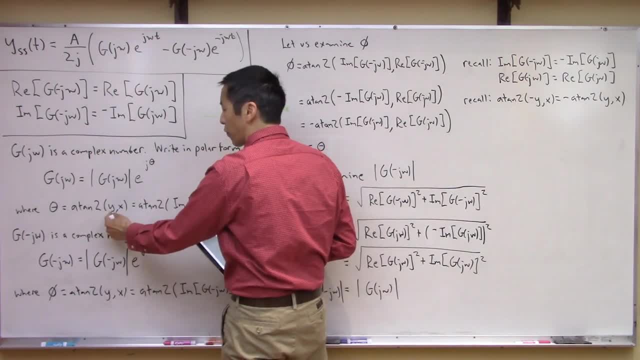 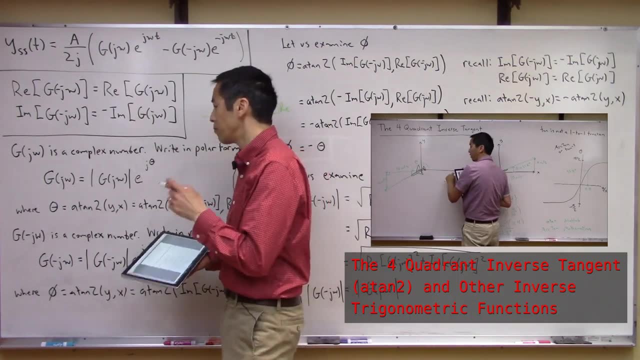 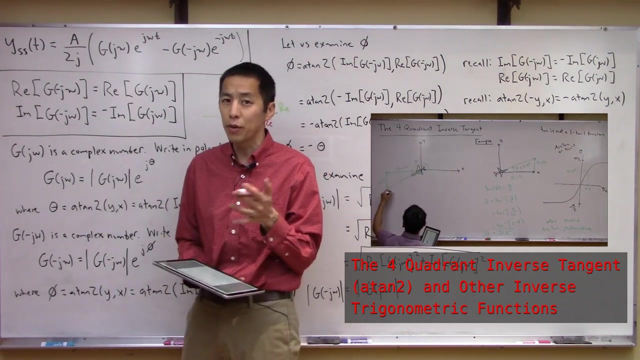 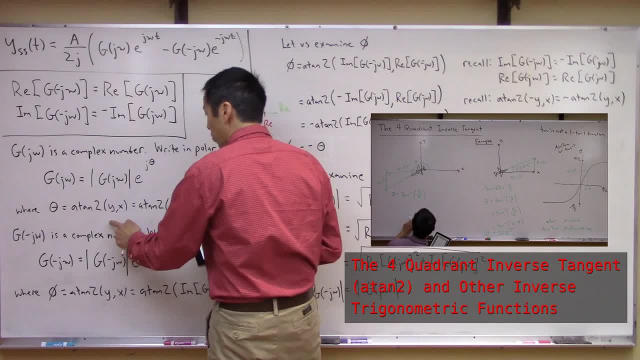 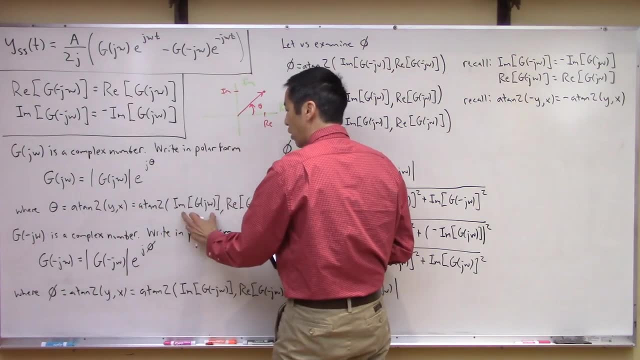 a tan 2 and the sort of the four quadrant inverse tangent. so if a tan 2 is not familiar to you, check out this video over here. um, but again i'm going to use sort of the matlab notation of it to note that yeah, we're looking at the y component, then the x component, right, so again this angle, theta. 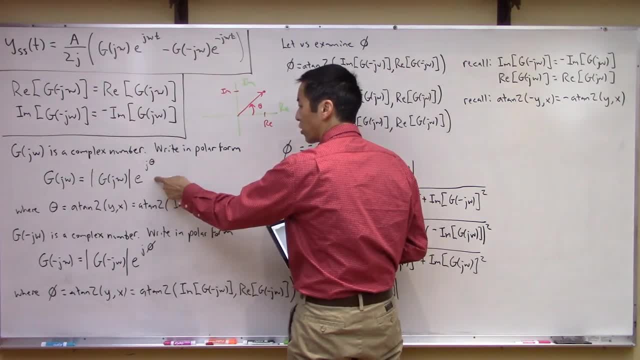 then it's just a tan 2 of: well, the y component is the imaginary component and the x component is the real component. right? so it's just this, right? so here you go. this is another way to write g of j, omega. okay, we can do the exact same thing we saw for g of negative j. 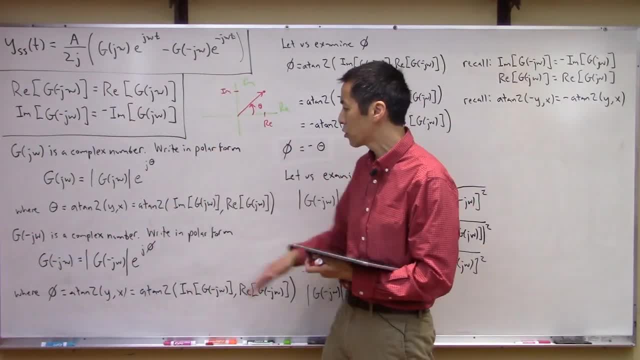 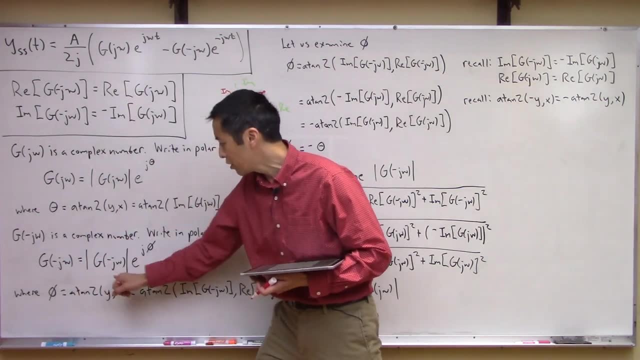 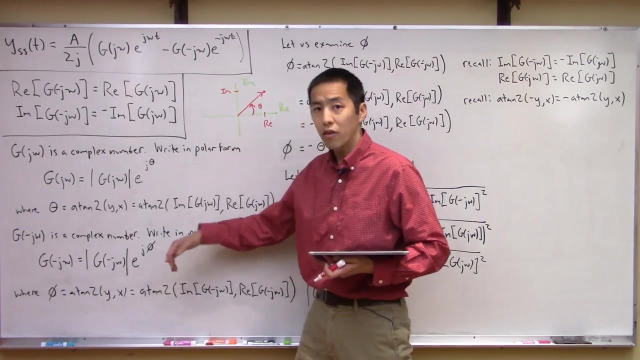 omega. again, at the end of the day, that was just another complex number, so same thing. write it in polar form, right? so this complex number g of negative j omega, well, it's just the magnitude of g of negative j omega times e to the j phi, right? so in this case, phi, the same thing, right? 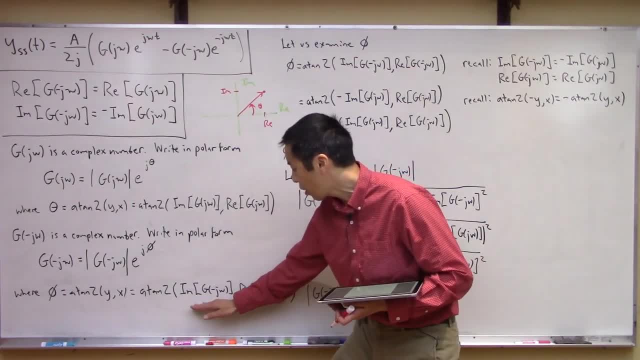 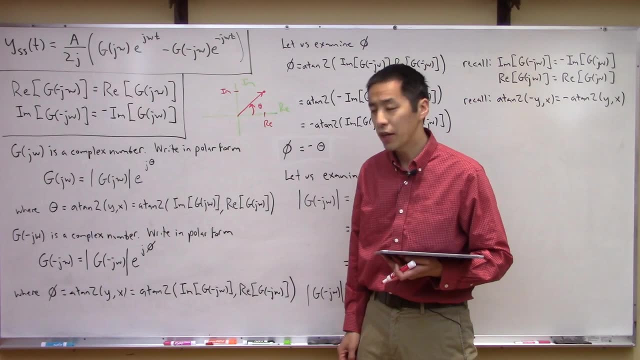 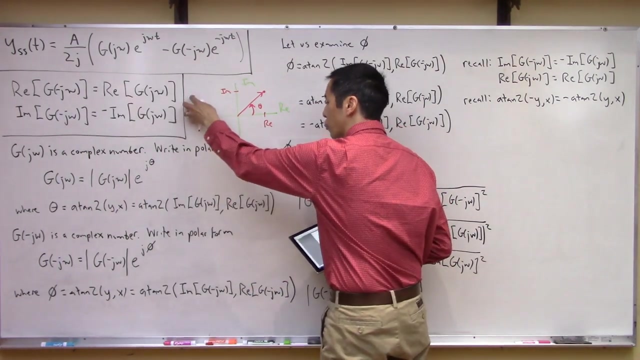 it's just you take the a tan 2 of the imaginary part of g of negative j omega and there would real part of g of negative j omega. right, That gives you this angle, phi. okay, Now here's where the kind of interesting part comes in and where we can now tie the previous result into what we're. 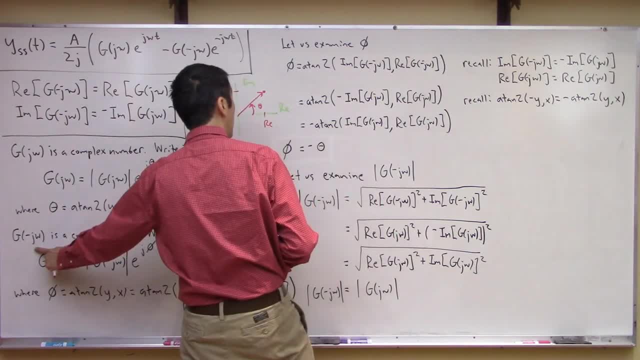 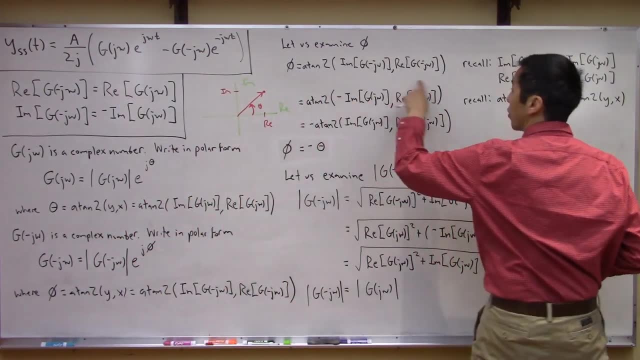 looking at. right now, Let's go ahead and examine this g of negative j term. okay, Let's start with how? about the angle associated with it? That's what we call phi, right? So I just rewrote it right here, right? Phi is just nothing more than a tan 2 of the imaginary part of g of negative j. 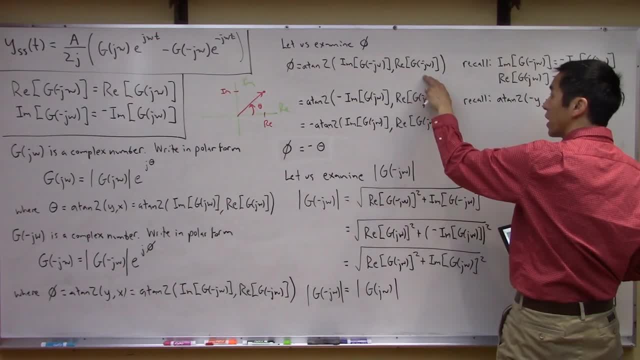 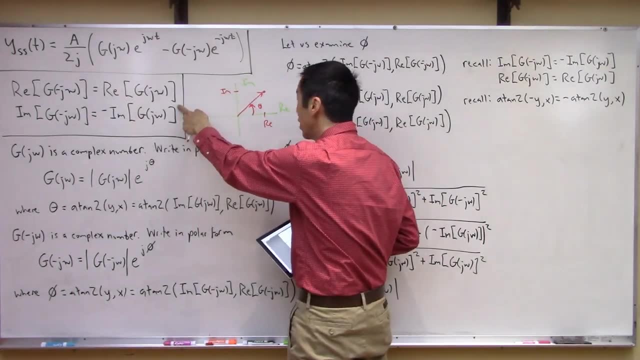 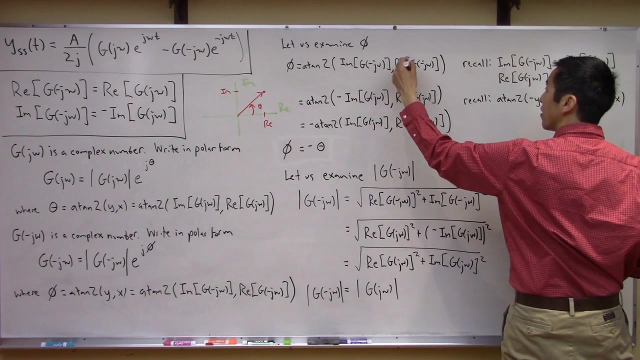 omega and the real part of g of negative j, omega. okay, Now, here is where I want to use this property that we spent time deriving, okay, So what we now know is that, well, this part, right, this thing, the here real part, here, this is the same thing as the real part of g of 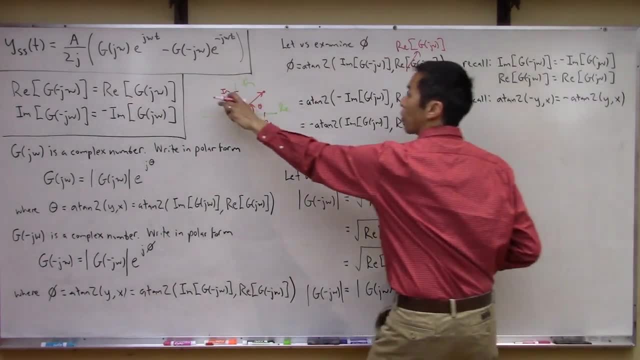 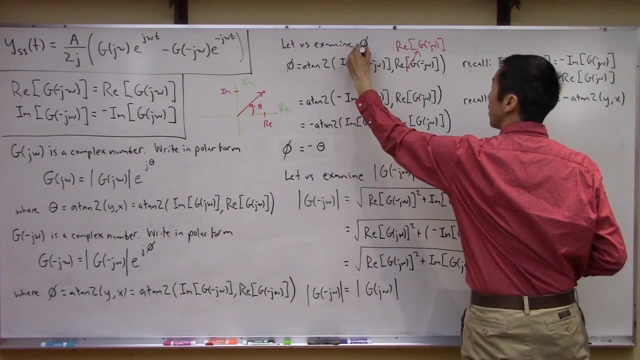 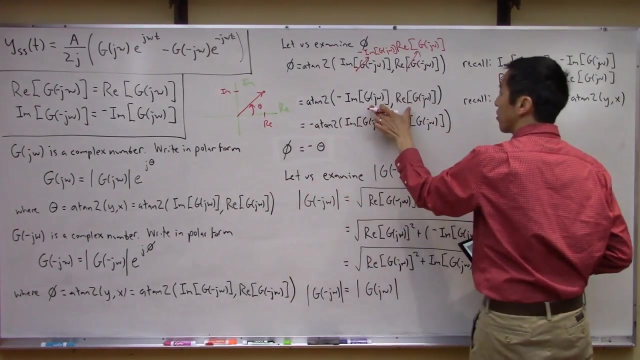 positive j, omega, right, That's exactly what we wrote right here, right? So that's that, This term, right here. this is the same thing as negative imaginary part of g of positive j omega, right? That's what we've got down here, So I'm just going to make that substitution in like such: right Now you. 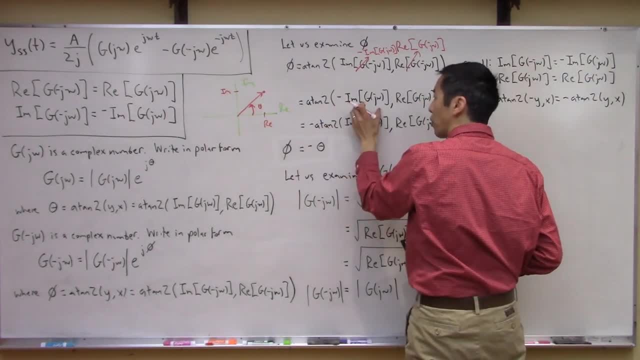 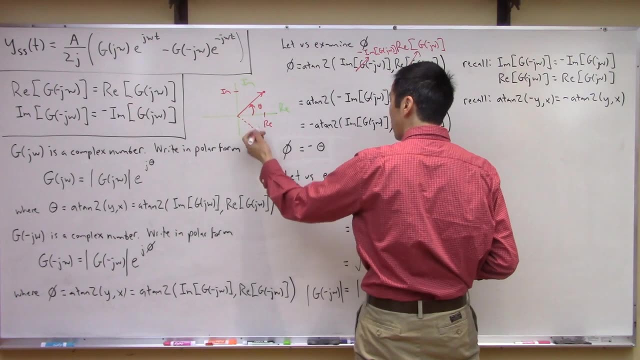 remember the way a tan 2 works right? This is the y component, So the negative y component. you're basically doing this right. You've got something like this, okay, So this is basically the property: that if you have the a tan 2 of a negative y x, it's the same thing as the negative. 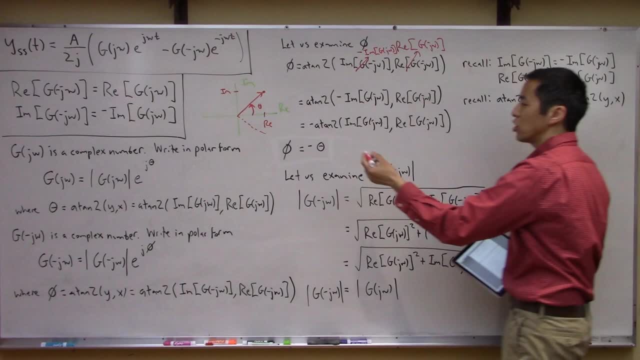 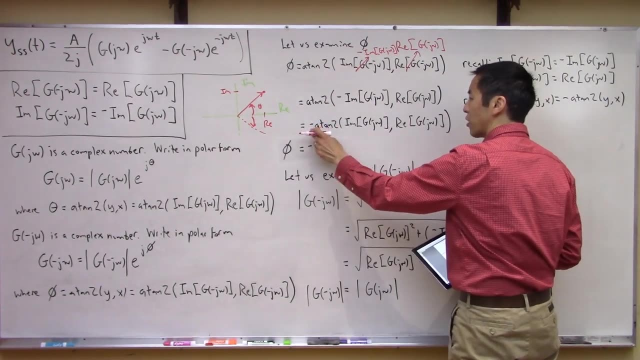 a tan 2 of a negative y x. So this is the same thing as the negative, a tan 2 of a negative y x. Right, Because it's basically just getting you a reflection like that over that angle, So you can clearly see that that comes. the negative sign comes out here, This part inside the negative. 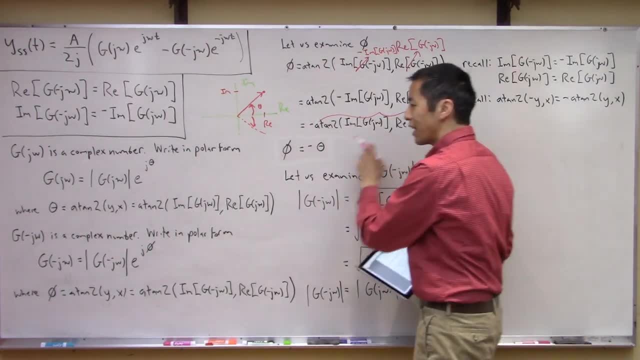 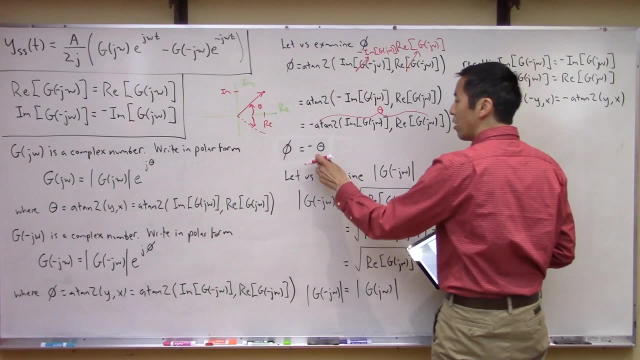 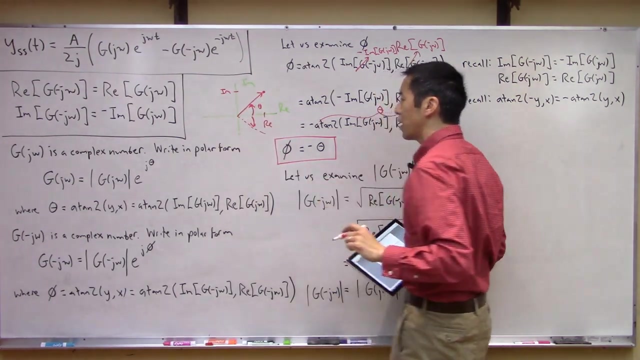 sign this thing right here. that is this right. This is theta right. This whole thing is theta. So we end up with this result here: that phi is nothing more than negative theta right. So it is indeed reflected over the. 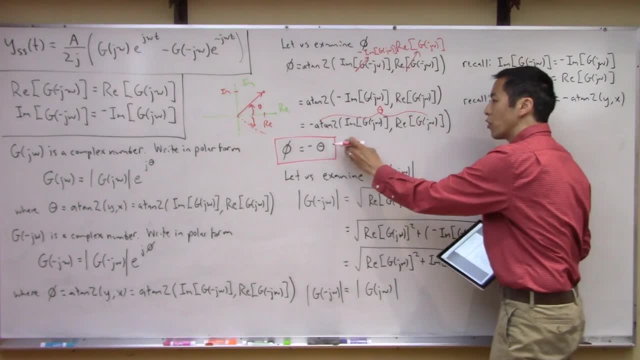 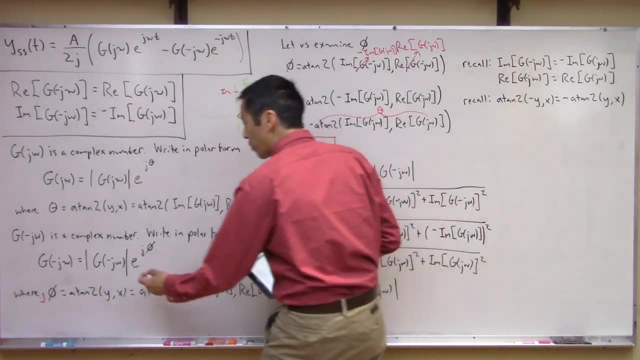 the real axis or the x axis, right? So here's one critical step, right. So now we understand what this thing is doing, this phi, right, Let's put a check mark there. The next thing that we might want to look at now is: how about this term, right? What is the magnitude of g, of negative j, omega? 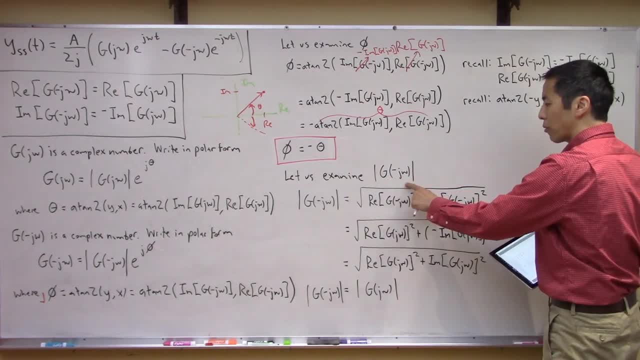 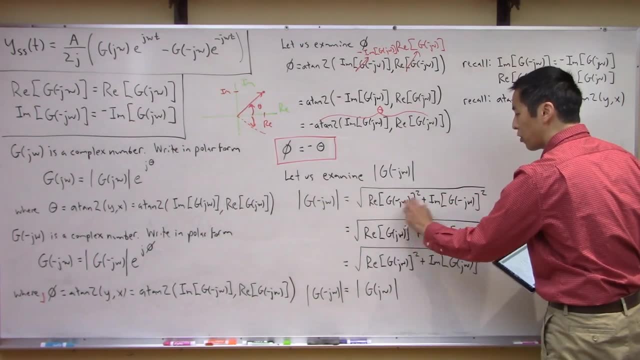 right. So again we can go ahead and examine that term. And again, this is just a complex number: g of negative j, omega. It's a complex number, So the magnitude it's just. you take the real part of it squared plus the imaginary part squared, you take the square root of the. 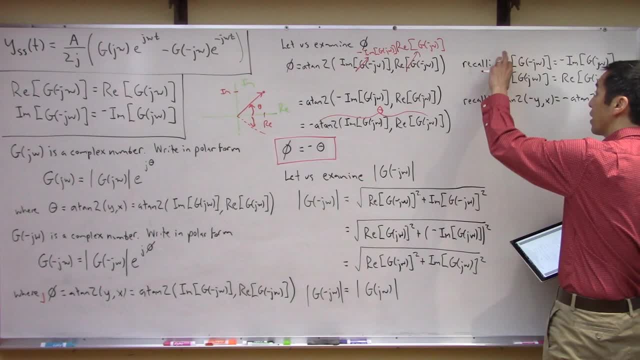 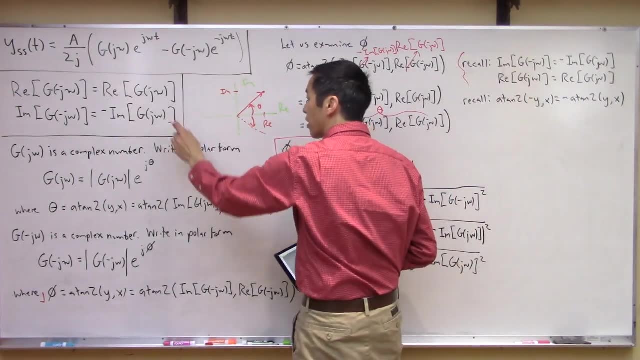 right. Okay, Now again, let's go ahead and play this exact same trick we did earlier here and substitute in these relationships: okay, Because I really don't, really I don't want the negative j omega. I want to write everything in terms of g of positive j omega, right. 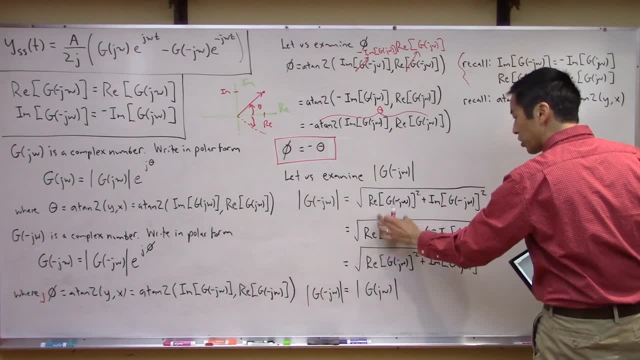 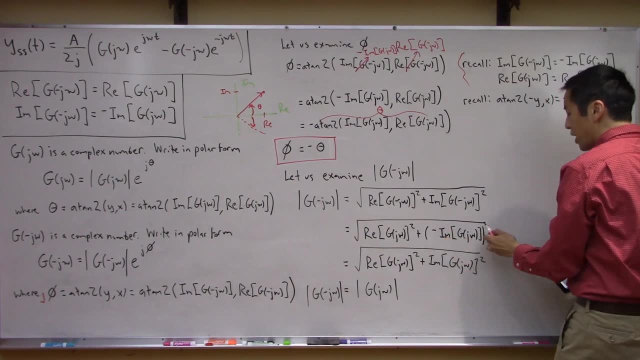 So again, the real part is unchanged, right, That's what we wrote up here. And then the imaginary part. you just pop in a negative sign here, okay, Which, again, by the time you square it, that doesn't matter, right. 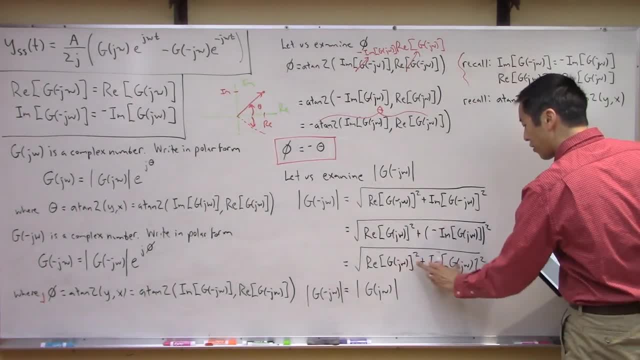 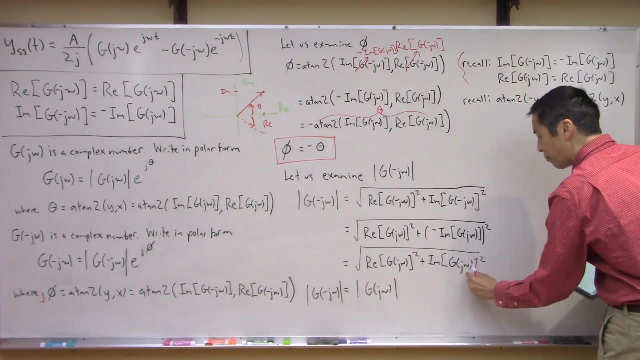 It's negative one squared is going to go away. So you end up with this. And if you stare at this long enough, this is just the real part of g of positive j- omega squared, plus the imaginary part of g of positive j- omega- squared, square rooted. So this right-hand side, it's nothing more than. 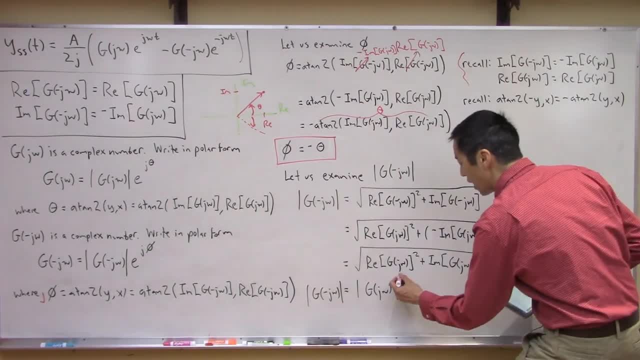 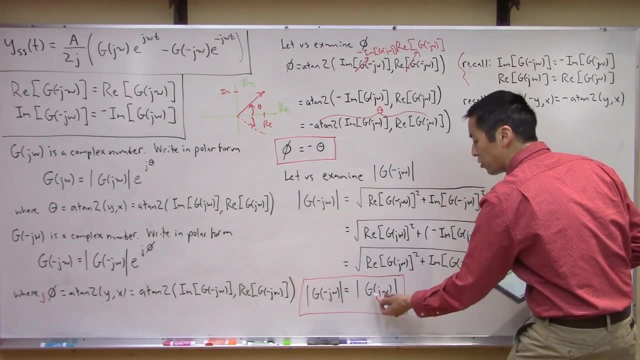 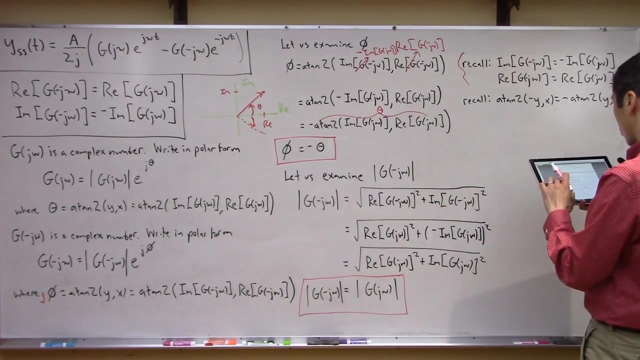 the magnitude of g of positive j omega. So again, we end up with this result here: that the magnitude of g of negative j omega is the same thing as the magnitude of g of positive j omega. right, So that is great. We end up with those two terms. So, really, at the end of the day, what we can do is 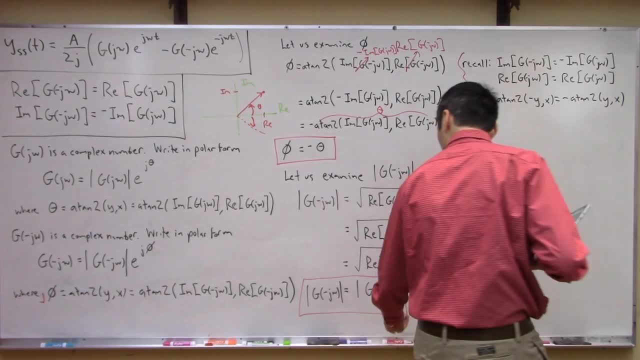 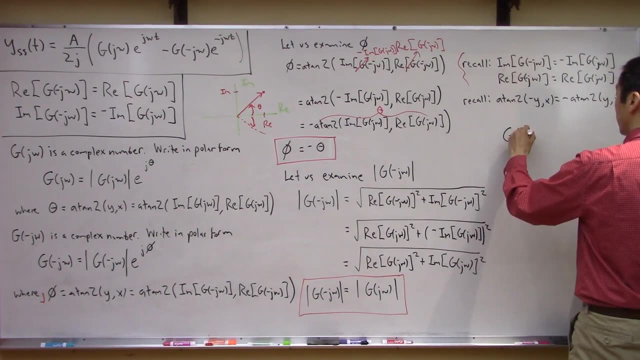 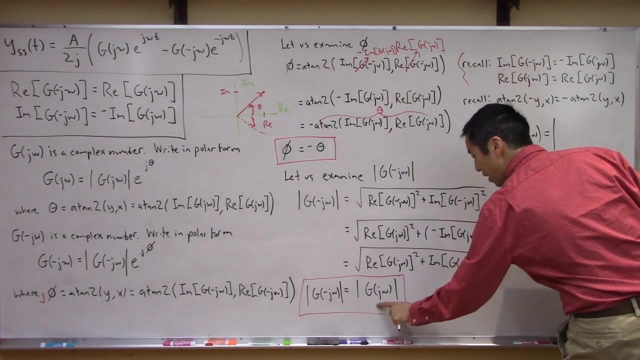 let's rewrite this right. So we have, let me pick a color, black, which is the same thing we have over there. So we said: g of negative j omega- right, It's the magnitude which is this, but that's the same thing as magnitude of g of positive j omega right. Times e to the j. 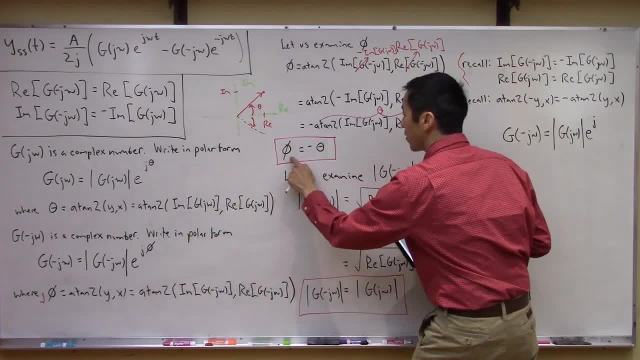 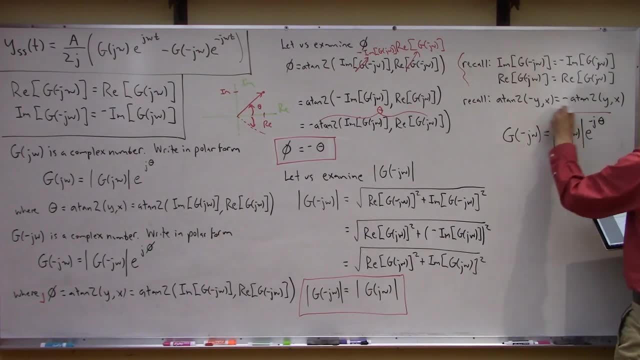 e to the j phi, but phi is the same thing as negative theta, So I can just write negative theta like that, right, And this is kind of one of the things that we're gunning for here. okay, So this is awesome, because now what we can think about doing is: let's substitute this expression. 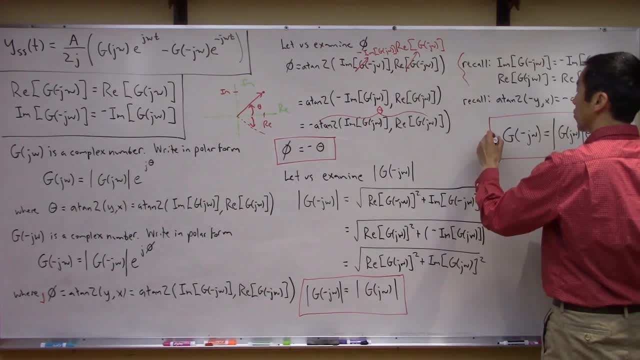 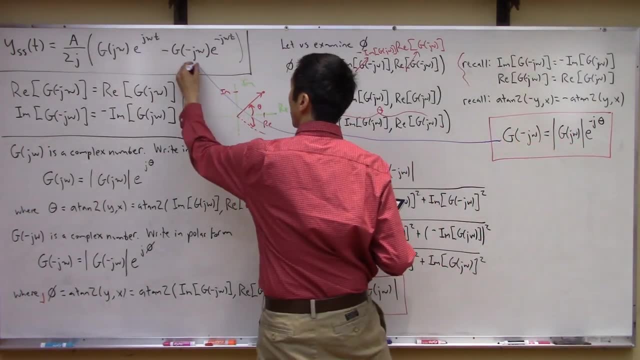 in to where is it? It is all the way over. I should let me. let me pick another color so we can see this. Okay, let's substitute this guy in to here, right, Because that is g of negative j omega. 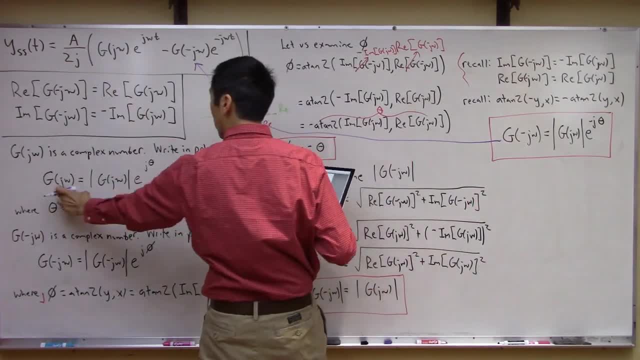 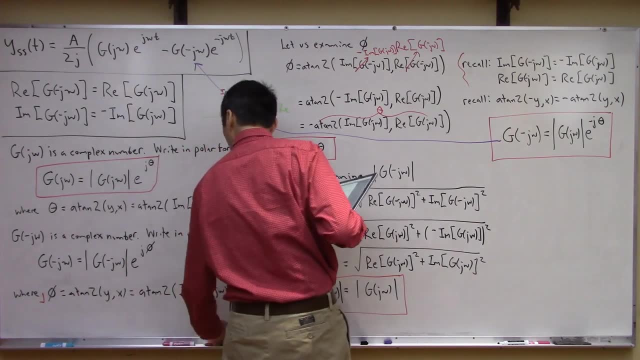 We have it right here. okay, How about g of positive j omega? It's, it's right here. Let me, let me box this guy up here. right? This is the polar form of it. right, Got the polar form here. 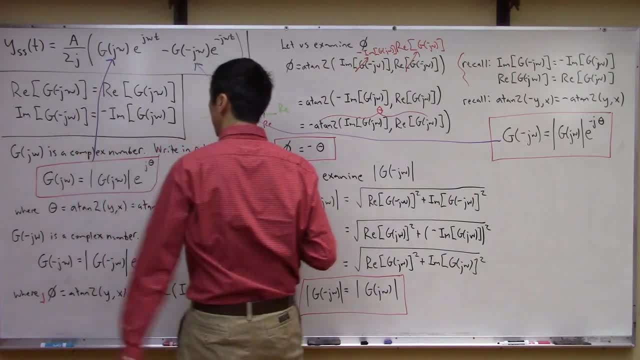 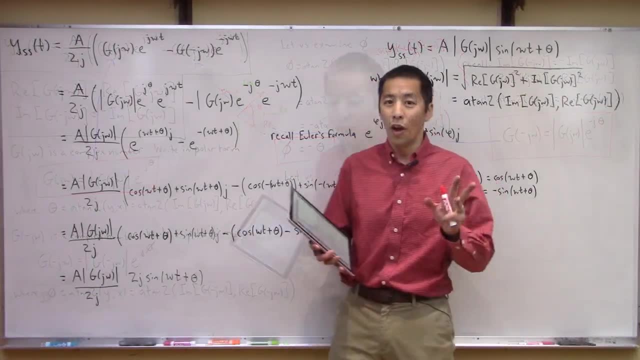 plug that in to that, okay, And let's see what we get. So give me a second to erase the board and let's make that substitution, Okay. so now this is where it's getting really exciting, and we're really cooking with gas Cause, remember. 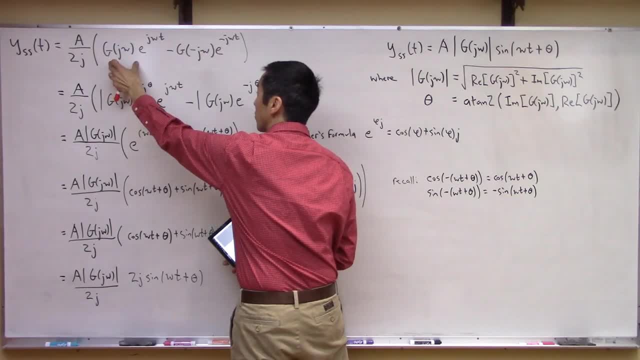 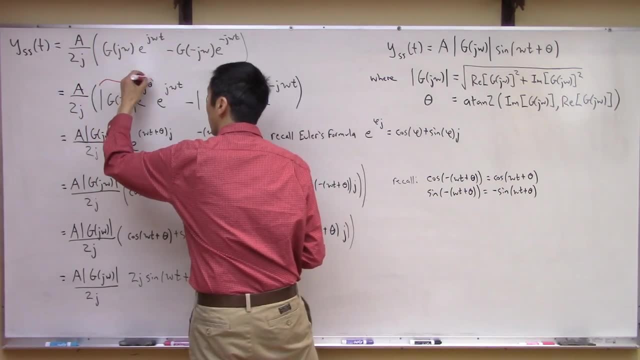 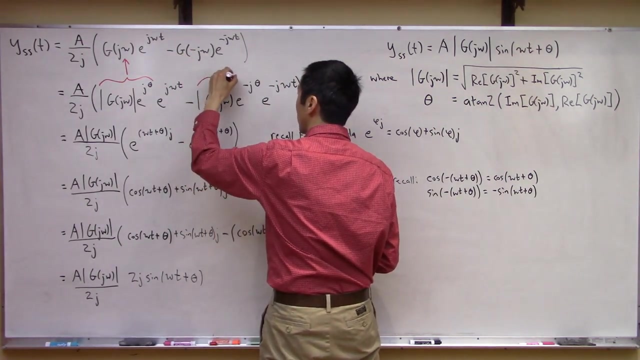 here was our steady state expression. Now again, let's just make this substitution So g of j omega. let's just go ahead and write it as a polar form like this: right, So that's that term there. And then, same thing, this g of negative j omega. we actually were able to write. 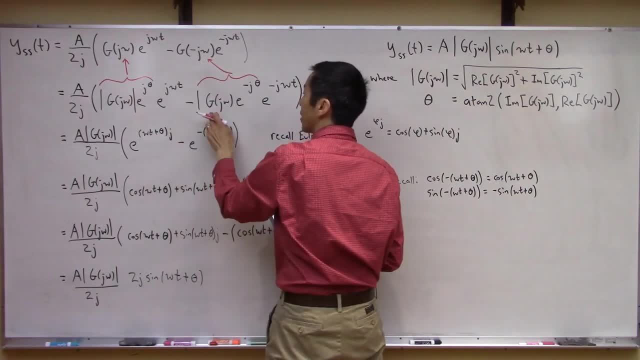 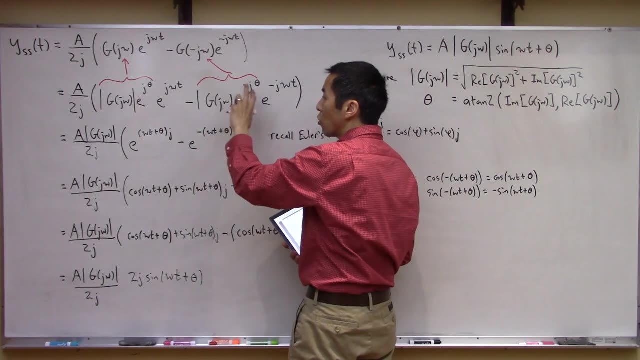 that as a polar form related to g of positive j, omega. As we just saw, we just had to make a negative sign here on the associated end, So let's just go ahead and write that as a polar form angle, right, okay? so that's what we got. so now let's make a couple of simplifications. um, first, 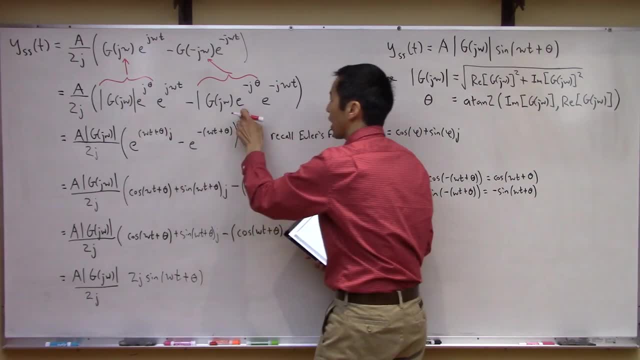 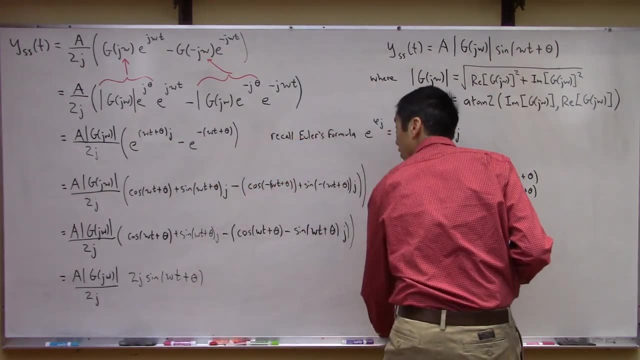 thing that we can easily see is: you got exponent times, an exponent, exponent, times, exponent. let's just go ahead and combine them and pull out the j on each side. whoops, and i actually look like i just forgot there should be a j right here. there we go. okay, that's all we're going to do. 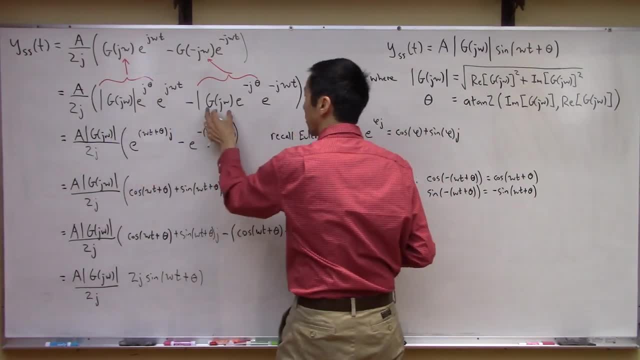 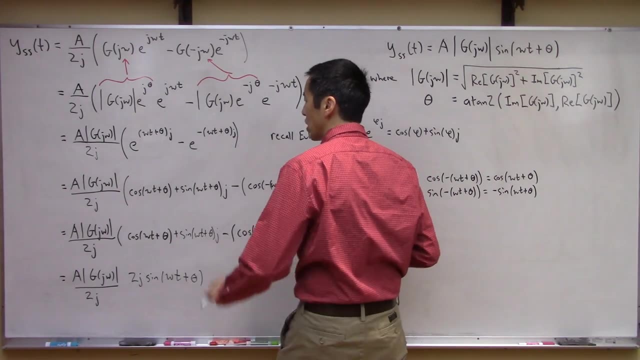 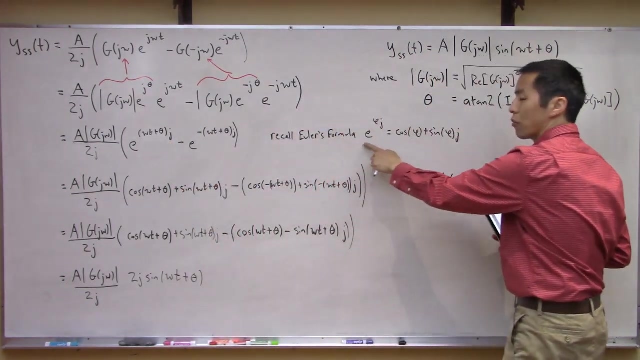 um, and also notice here that there is a magnitude g of j omega, magnitude g of j omega. so let's pull that out here, okay. so here we go. this is, uh, one simplification. now you stare at this. this exponent, right, it's e to the something i right. do you remember euler's formula? right, where it basically: 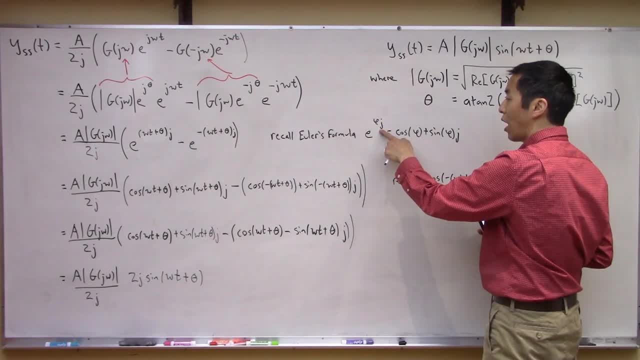 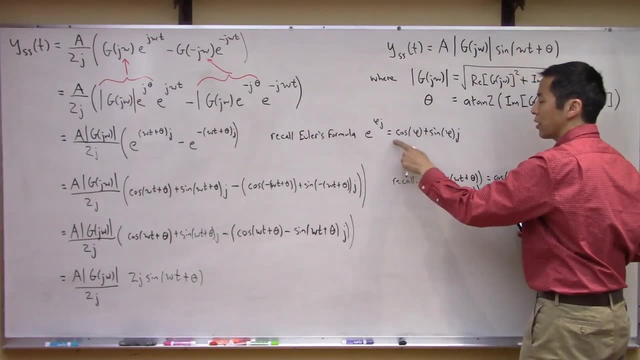 said, euler's formula was e to the anything, uh, i or j. you can write that in terms of cosines and sines like this: right, okay, so let's just make that substitution again. make the note that e to the- in this case i'm going to say e to the phi- j- is just cosine of phi plus sine phi times. 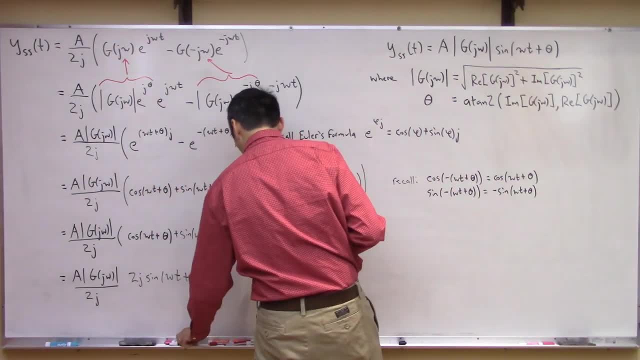 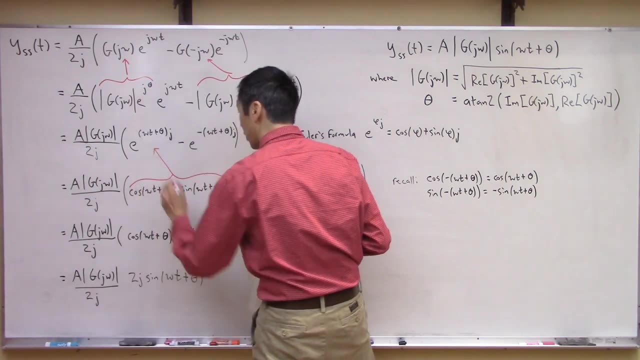 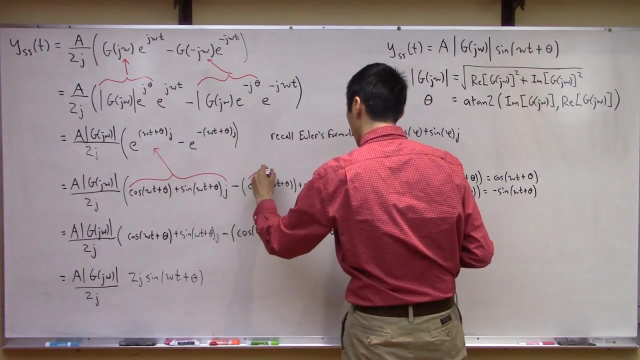 j right. so this thing right here again. maybe we'll go ahead and note this this term right here. that is nothing more than euler's formula for that guy, right, and then same thing. i got a minus sign. i'm just going to euler formulate formula, this exponent. so that's this thing inside this. 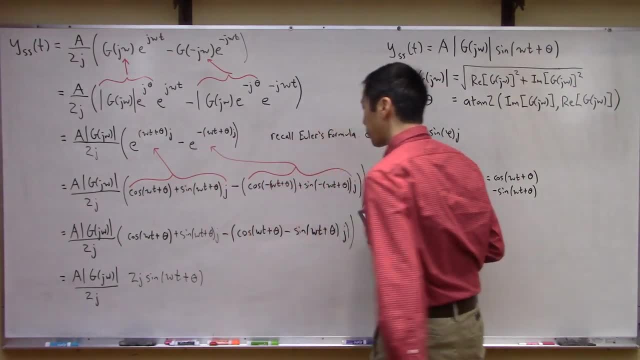 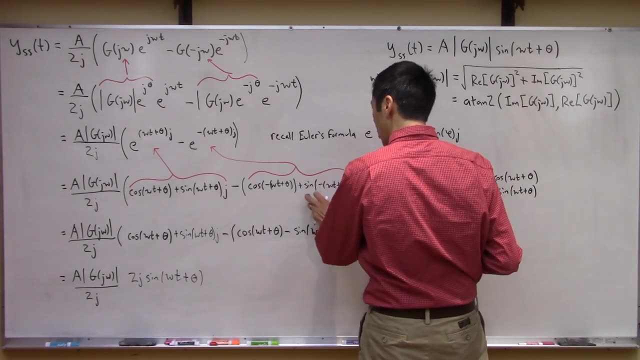 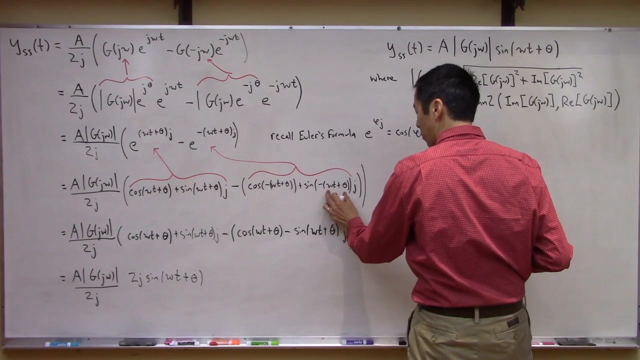 set of parentheses. is this term there right? okay, great, so now we just got to be a little bit careful. um, let's take a look at these two terms here. these, this cosine and sine right. so this is basically cosine of a negative something right, and sine of a negative something. 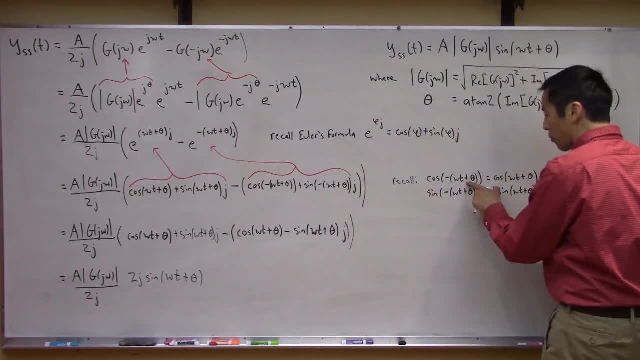 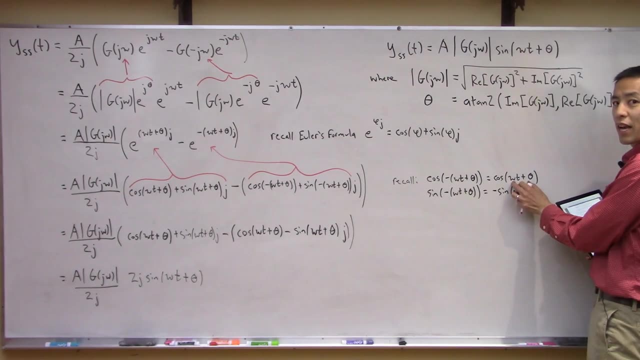 here, right, let's just look at the cosine and sine. everyone you remember, right, cosine is an even function. so if you have cosine of negative something, it's the same thing as cosine of that thing, right? the negative sign doesn't matter because it's an even function. similarly, sine. 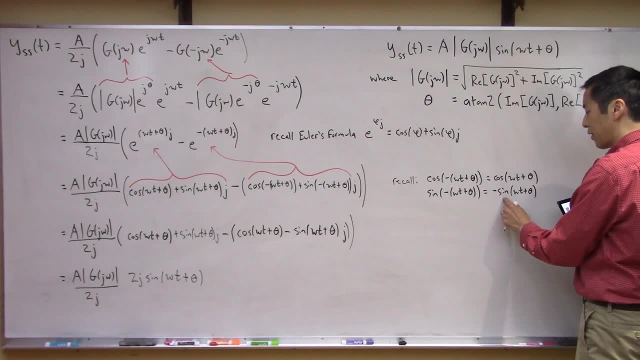 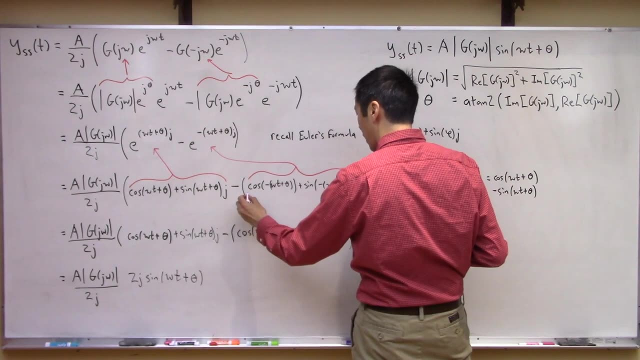 is odd where sine of a negative something, it's just negative sine of that something, right? so let's just go ahead and make that replacement here. so that's all i'm doing here is: um, i'm going to use the fact that cosine is even to basically get down to here, right, just going to. 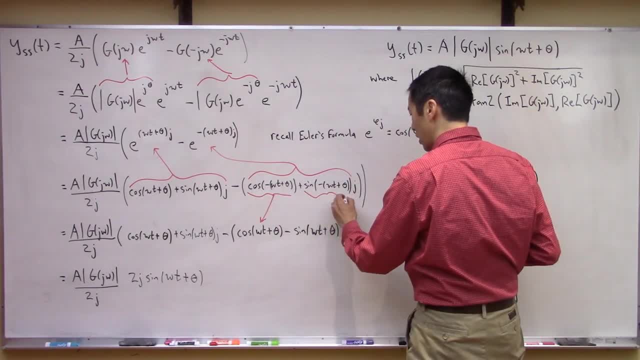 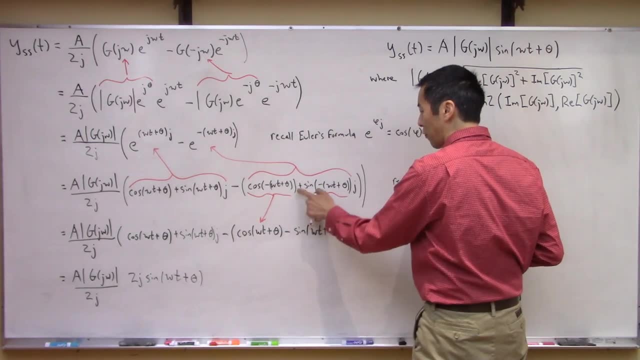 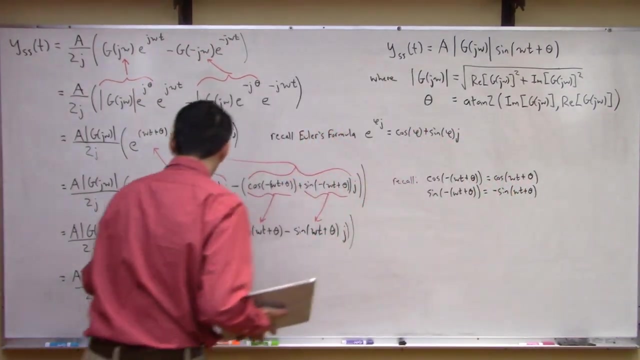 knock out that negative sign- and i'm going to use the fact that sine is odd to basically get to here- but switch the sign, the the s-i-g-n in front of the sine s-i-n function, right, that's all i'm doing, okay, now? now we're really cooking because, man, if you look at this, i got a positive cosine omega. 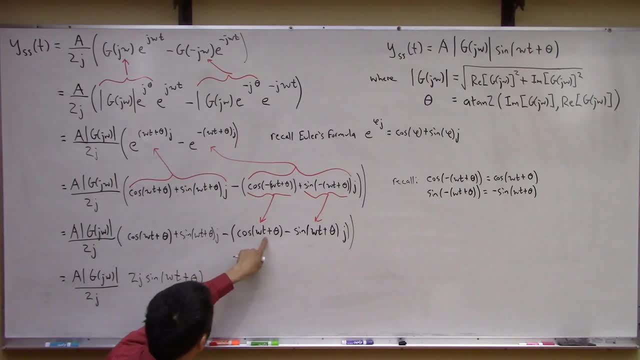 t plus theta and a negative sine omega t plus this. so this will cancel with this term here. and then i got a positive sine omega t plus theta minus a negative sine omega t plus theta. and sorry, j's right. so this is really. this is two sine: omega t plus theta. j right, that's this thing, right. so this combined. 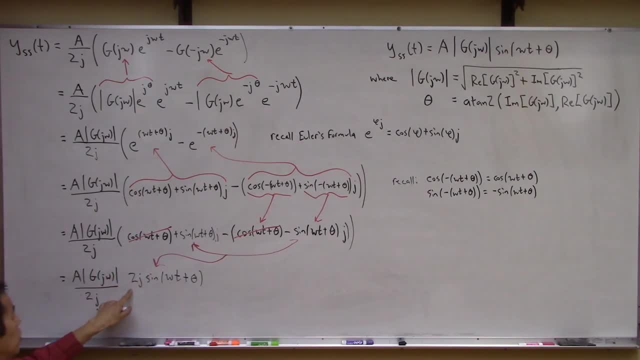 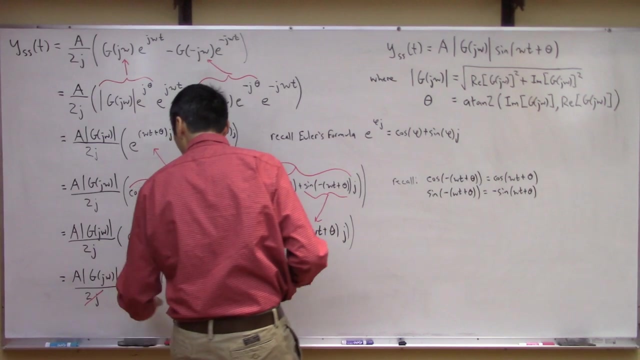 with this will get you this right: two j sine omega t plus theta right and man. this is really exciting because man look at this and again i always get excited by this because look at this, like the imaginary terms all cancel out at the end of the day, if we did all of our math and our algebra and our manipulations and simplifications properly. 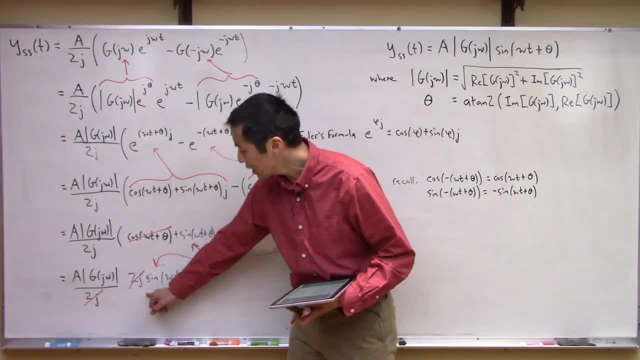 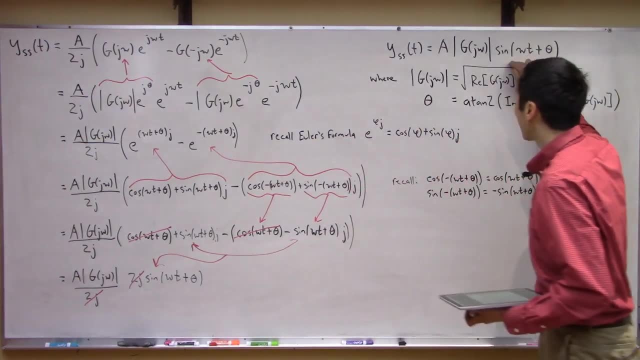 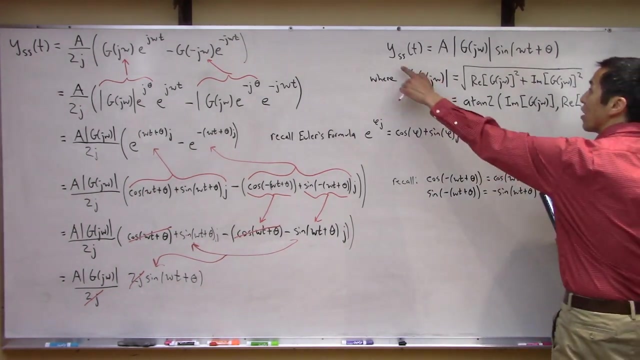 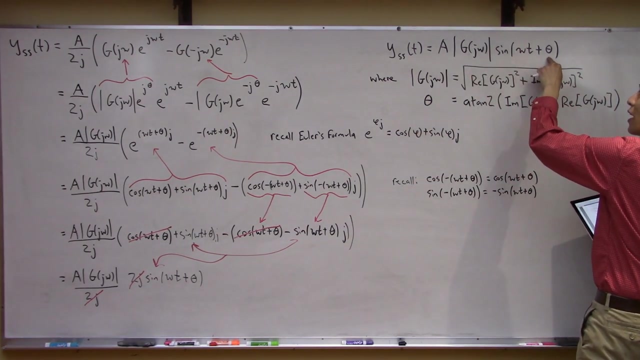 look at this. the imaginary stuff went away. so suddenly this entire expression for y steady state crushes down to this right um, and this makes good physical sense of what this is. this says why steady state, it's just what it's: a times magnitude of g of j omega, times sine omega, t plus theta, where this thing, this magnitude of g of j omega, right, it's nothing more than, again, g of j omega. it's a complex number. so it's magnitude, it's just the real part squared plus the imaginary part, squared, square, rooted right. and this thing here, this theta, it's just a tan. 2. 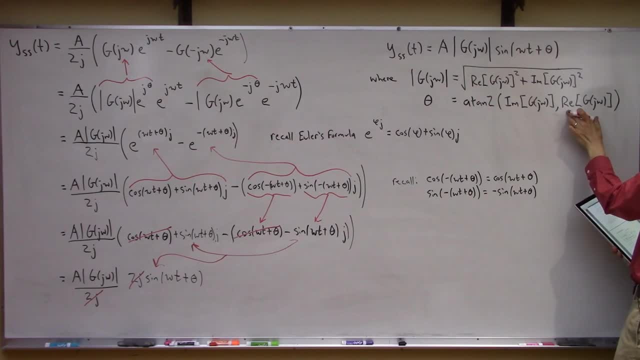 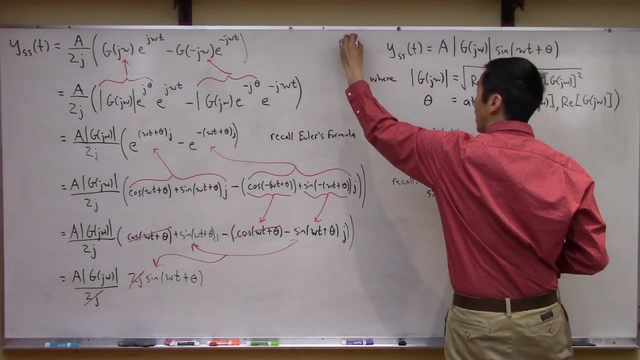 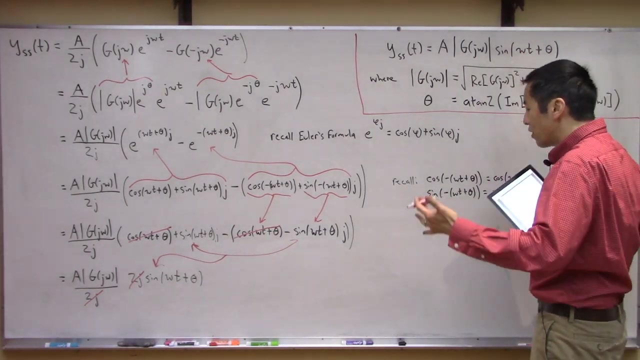 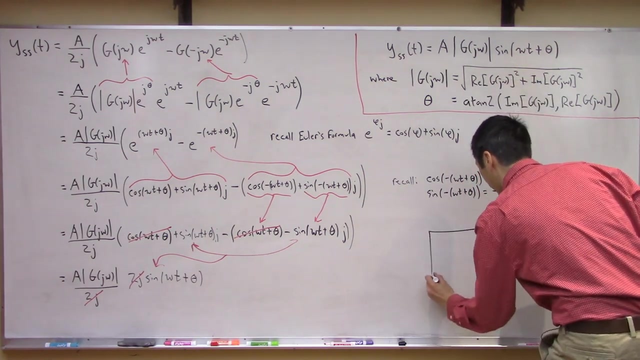 of that imaginary number. right, you give it the y component and the real component, you get the angle associated with that vector. that's what this is right. so, again, this is amazing and and just it's so elegant that it came down to this for this linear system. um, because let's take a step back and ask ourselves what's physically going on here, what, how did we get here? right, it's been a couple of minutes since we set the stage for this, so it might behoove us to kind of come back and ask what. 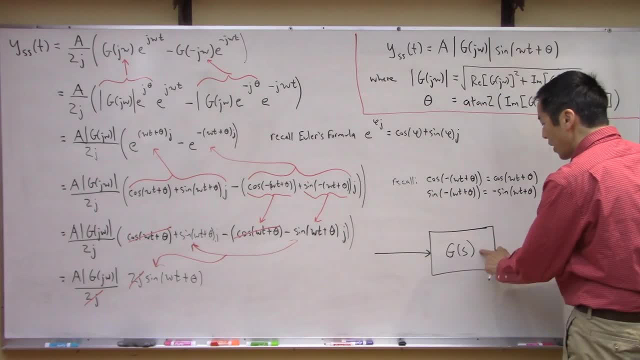 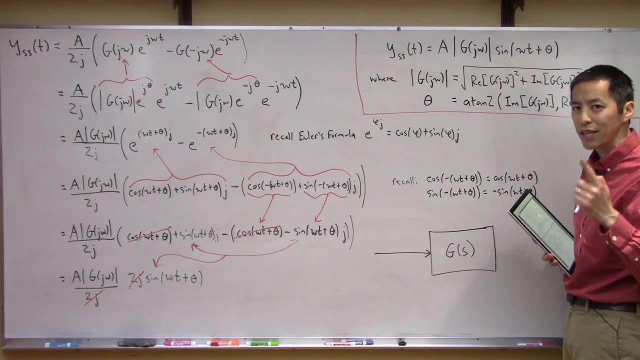 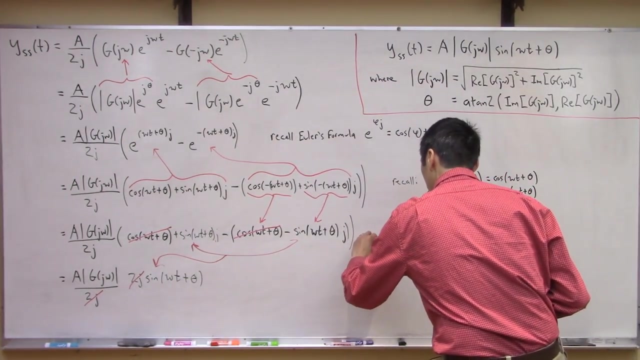 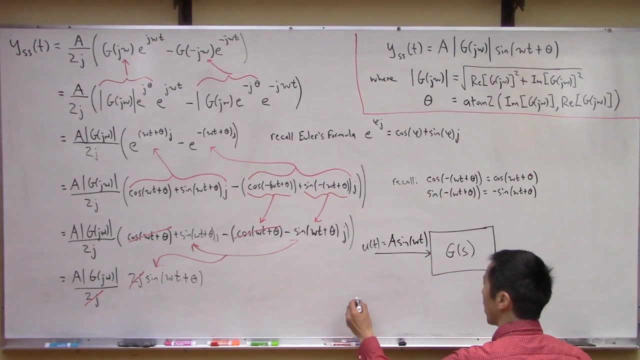 were we doing with this frequency domain analysis stuff? right, we said we had a linear transfer function g of s. and again, remember, this is an arbitrary g of s right. as long as it is strictly stable, this could be basically anything right. and what we did is we said the input to this was a sine wave of the form, a sine omega t right. so what you did here is we basically put in a sine wave to this thing. 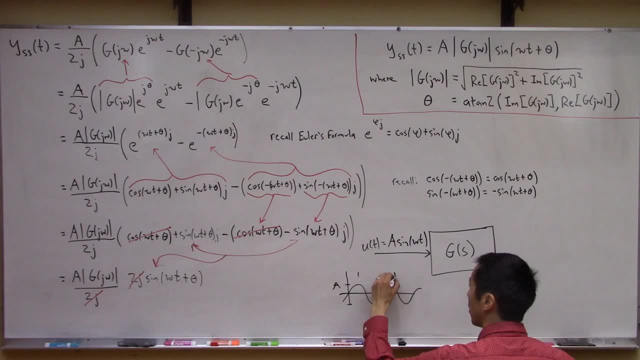 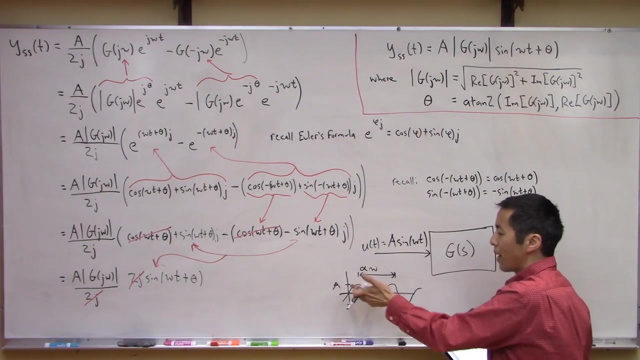 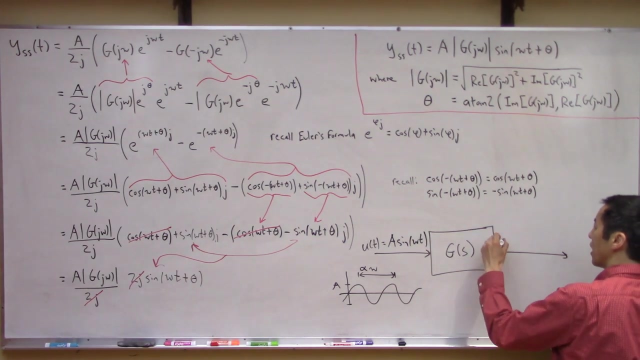 with an amplitude of a and some angular frequency omega, right? well, okay, i don't know if i should draw. this is technically the period of the sine wave, but you get what i'm saying. maybe i'll write it like this: it's proportional to the- uh, the frequency, right? um, you put in a sine wave of magnitude a angular frequency omega into this thing, right, and what we have now is we are interested in actually the steady state response of this thing. 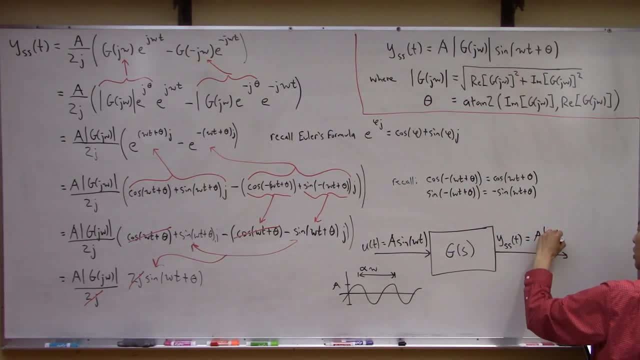 that thing up there, right, it's a times magnitude of g of j, omega, uh, sine omega t plus theta, right? so let's think about what does this actually tell us now, right this, if you look at this steady state response. so, again, what we've got now is, if i look at y of t versus t, again, i am not going to care about what happens in this sort of 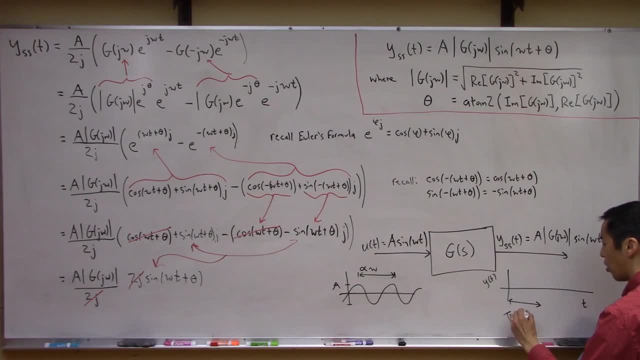 transient period, right. so here's transient. we know there's going to be a lot of stuff going on, but if i let all those transients die away and i let t become large, eventually the steady state response is going to look like this. and look at this: what is this? this is a sine wave of the exact same angular frequency as the input sine wave. the only difference is that it is phase shifted by the amount theta. and let's look at the amplitude. what's the amplitude of this output? the amplitude it's, i mean you. 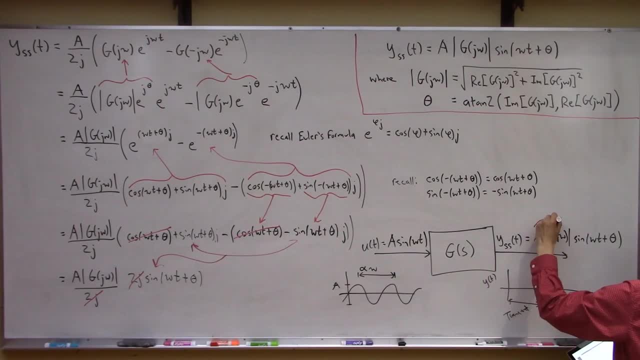 can see it right here, in the term right, this composite term. right here is the output amplitude, right, so the output of this guy, it's, it's, it's. you know, maybe i'm gonna, oh, sorry, sorry, hold on, i do not want to draw the, uh, the, the transient part, i want to draw it out here. you know, eventually it's going to look something like this: right, where the amplitude of this is a times magnitude of g, of j, omega, right, and again, the 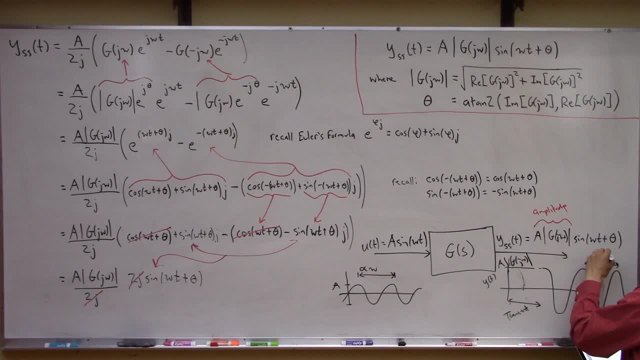 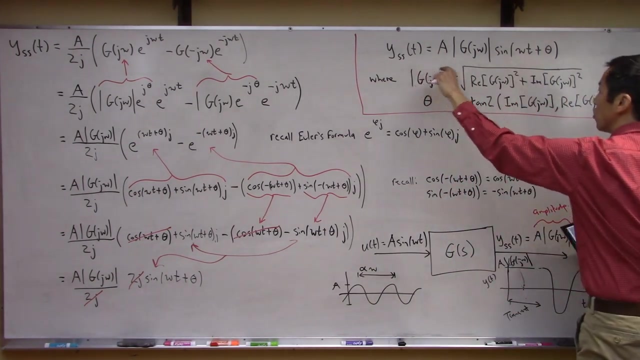 phase, or sorry, the frequency is, you know, something proportional to the omega. so you get out a sine wave which is looking very, very similar to the input sine wave, except that now the amplitude has been magnified by g of j omega. right earlier we had an amplitude a, now you get an amplitude a times g of j omega. so this thing right here, a physical intuition of what this means is, you can think of this as an 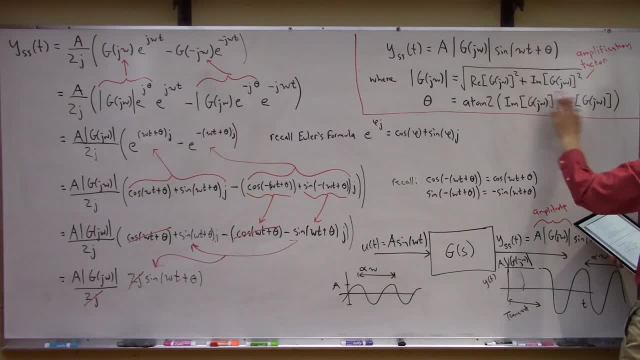 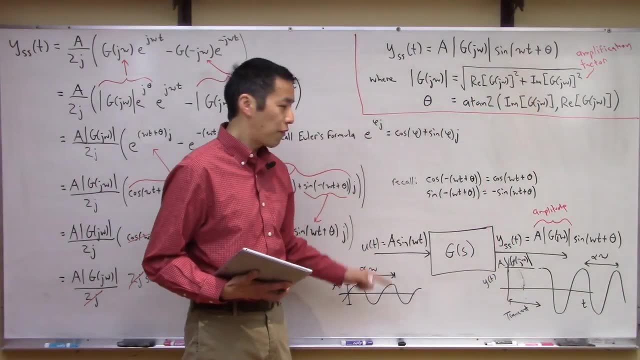 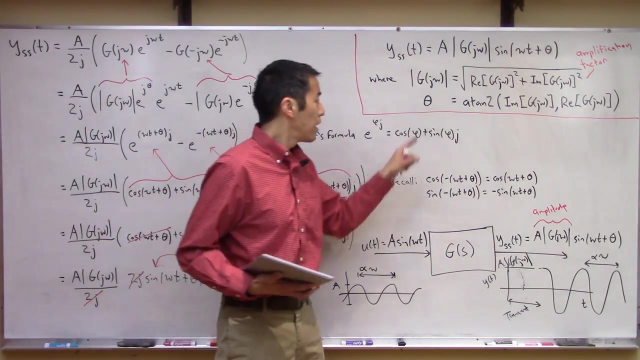 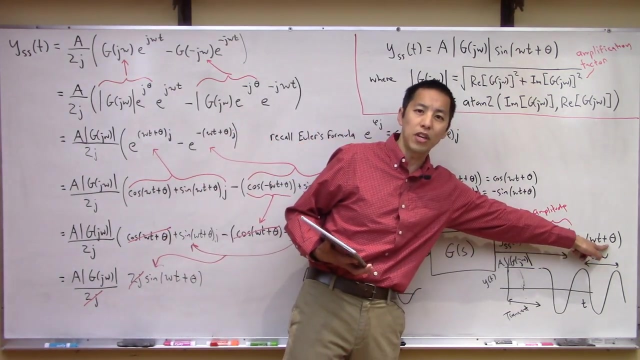 optimization factor, right? so if this thing is bigger than one, you are going to get a bigger sine wave out. then you put in: if that number, if this magnitude of g, of j, omega is less than one, you're gonna get a smaller sine wave, then you put in, right. and now we also understand now what this theta is, right? this theta, it's basically a phase shift, right, you can see. so this theta is a phase shift. 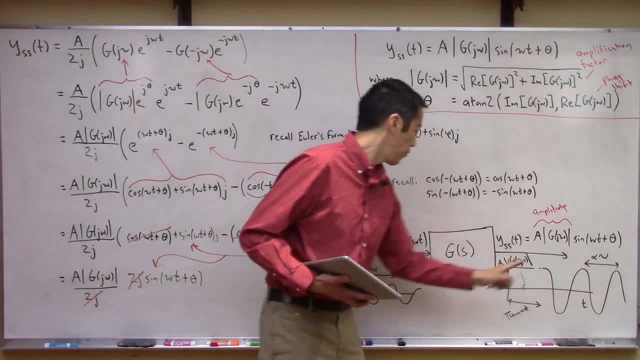 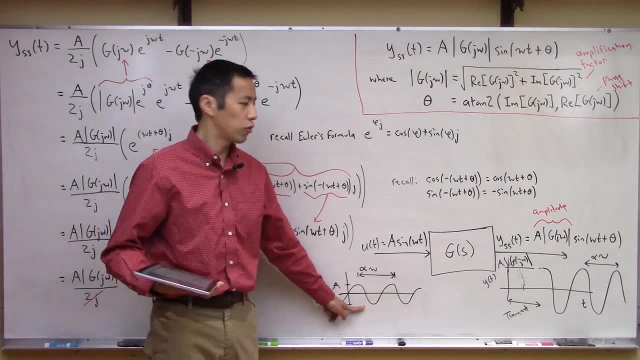 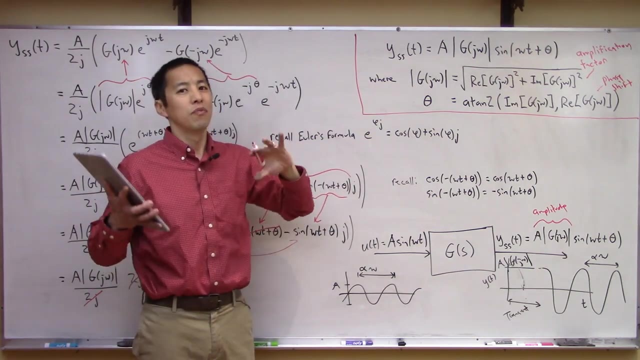 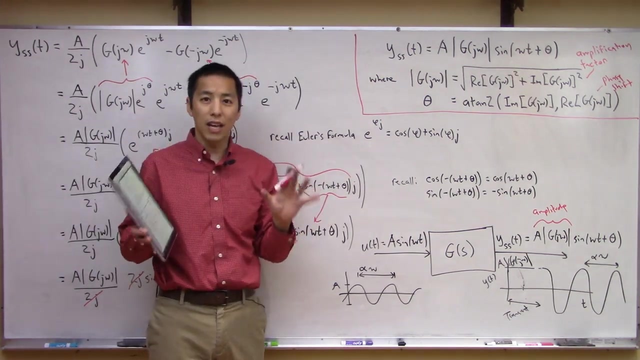 so again, you will get out a sine wave which is phase shifted from the input sine wave or lagging the input sine wave by some amount, right, depending on what this, this imaginary number, is, uh, when you calculate its angle right. so again, this is just so incredibly elegant that, again, if you think about what just happened here is we did a lot of analysis to come up with this result that says: i can predict. 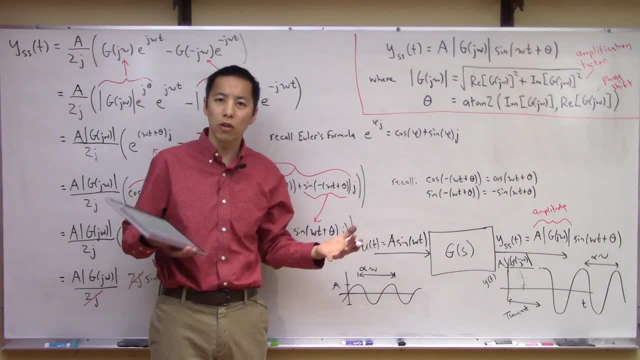 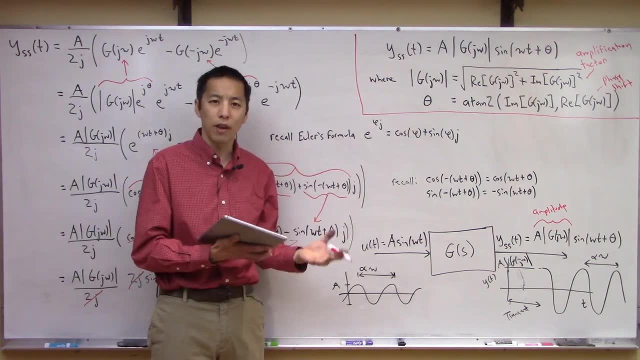 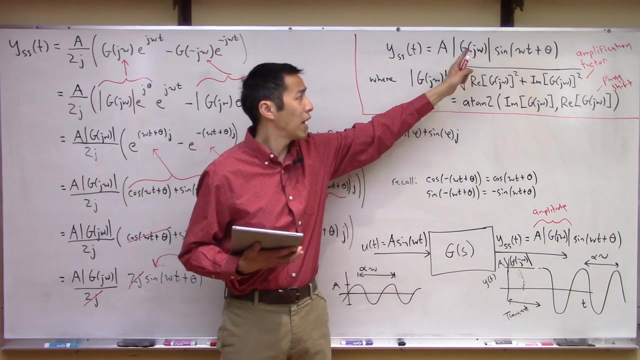 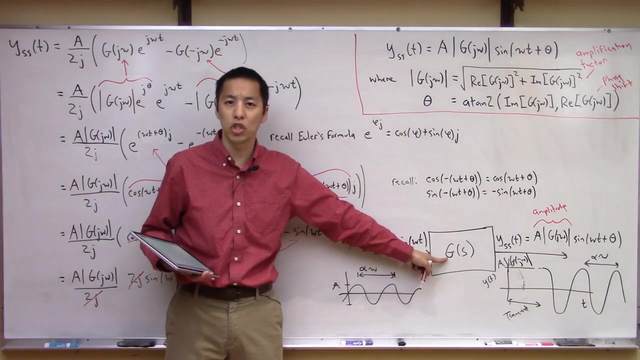 that steady state what the system is going to do in response to a sinusoidal input. right, and what's going to happen is you are guaranteed to get out a sine wave. that is the same angular frequency, but it is amplified or attenuated by g of j omega and it is phase shifted by theta. and again you can calculate all of that. the second someone drops this transfer function g of s in your lab, all you do is you replace s with j omega, and it is phase shifted by theta, and again you can calculate all of that. the second someone drops this transfer function g of s in your lab, all you do is you replace s with j omega, and it is phase shifted by theta, and again you can calculate all of that. the second someone drops this transfer function g of s in your lab, all you do is you replace s with j omega, and it is phase shifted by theta, and again you can calculate all of that. the second someone drops this transfer function g of s in your lab, all you do is you replace s with j omega, and it is phase shifted by theta, and again you can calculate all of that. 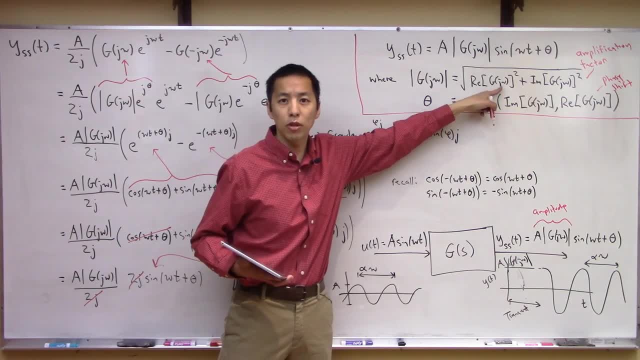 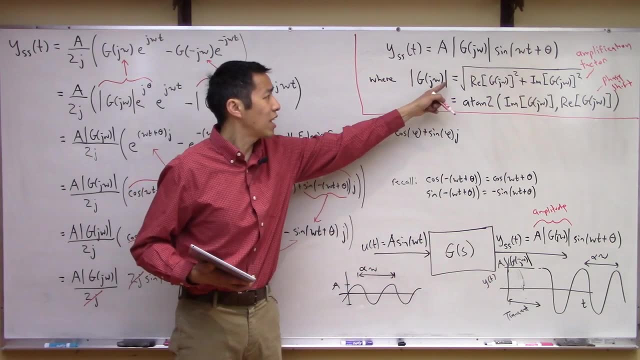 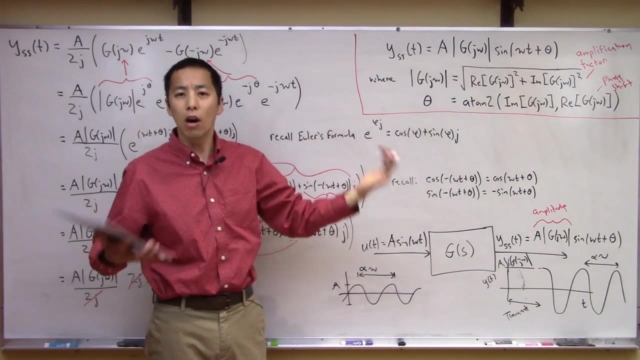 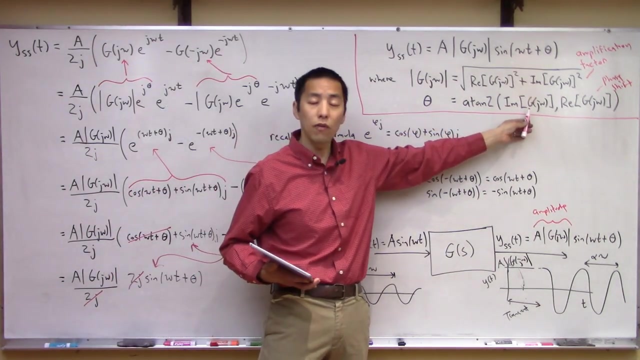 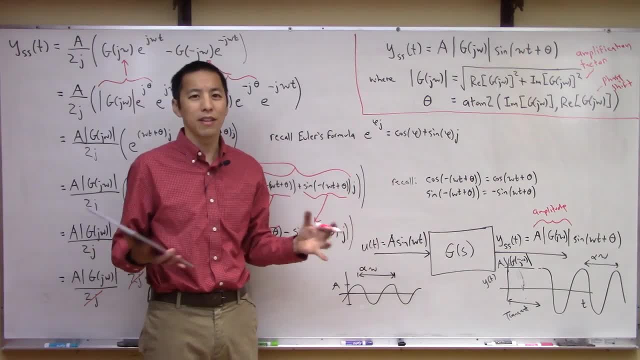 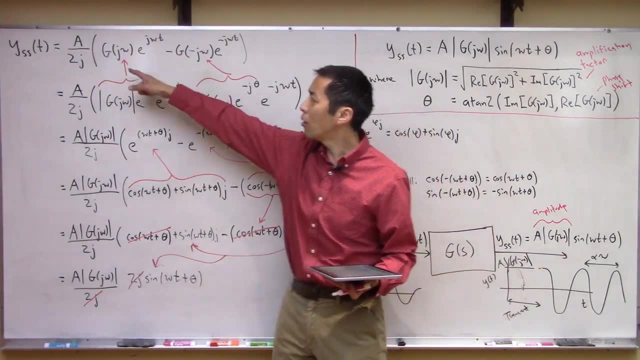 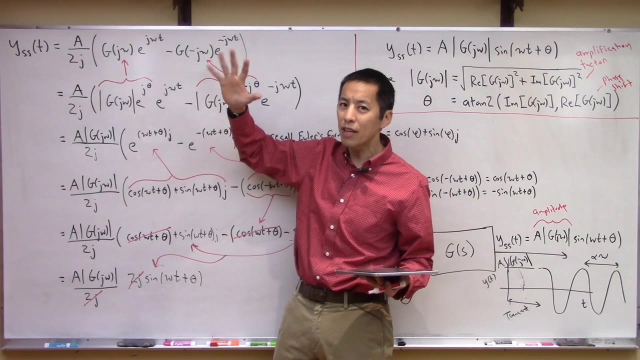 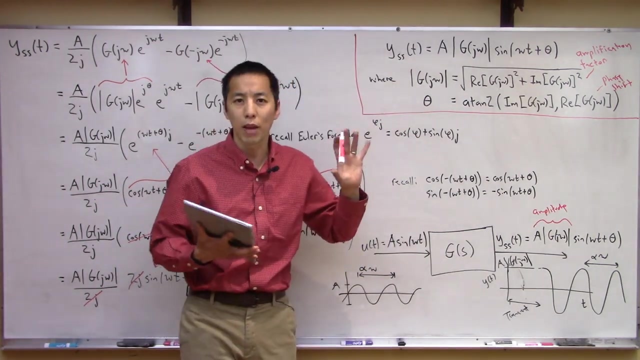 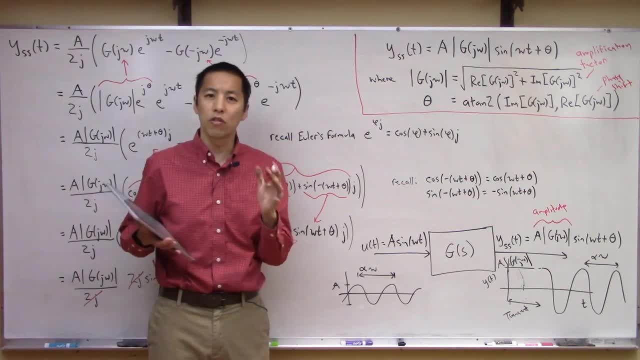 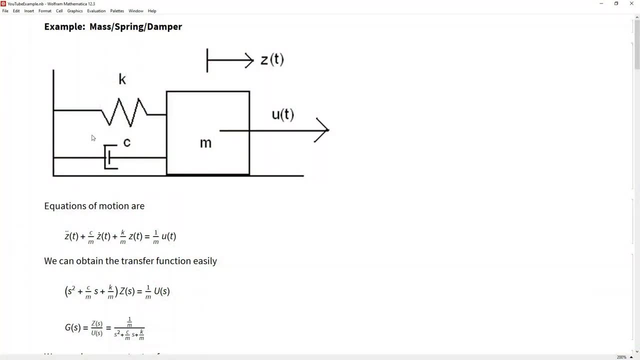 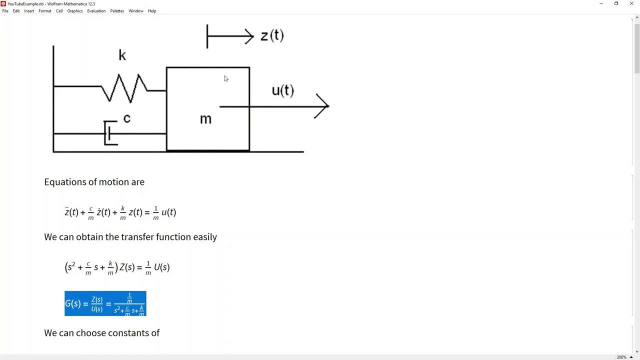 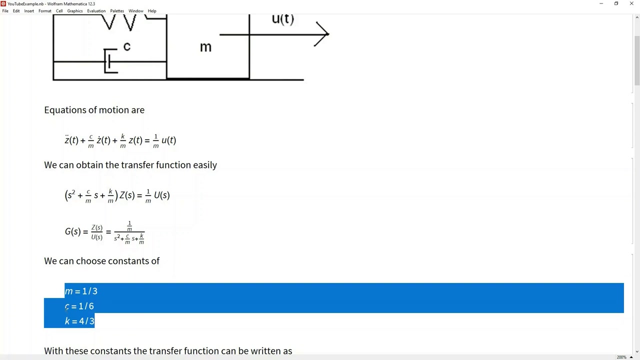 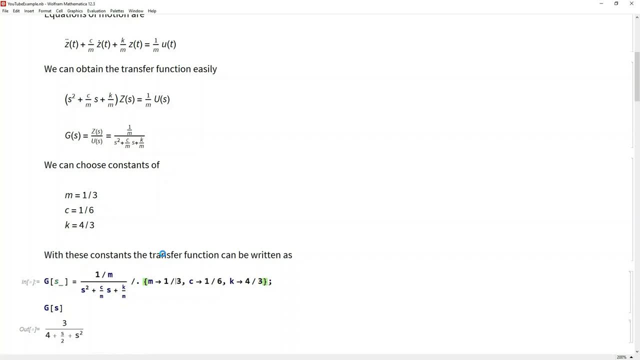 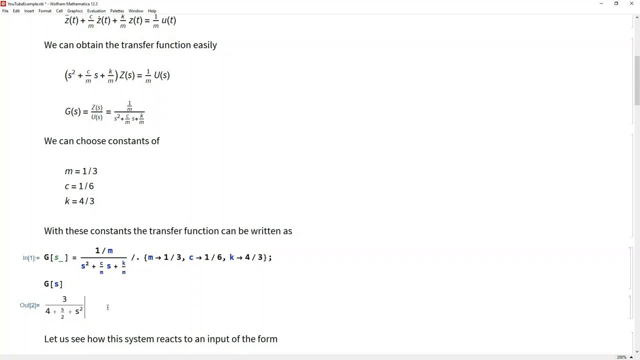 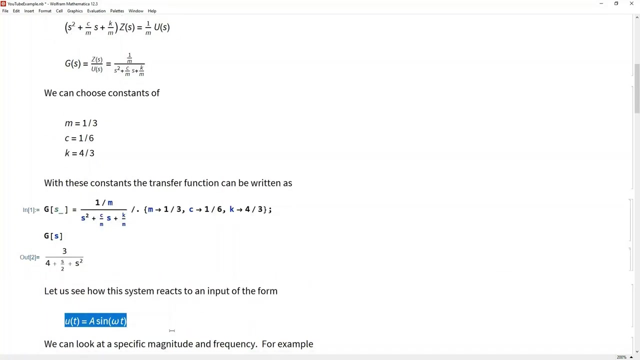 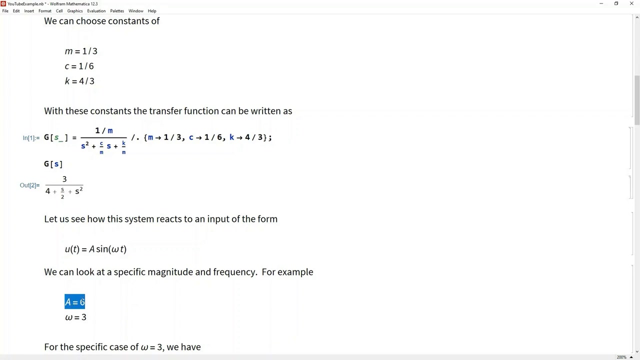 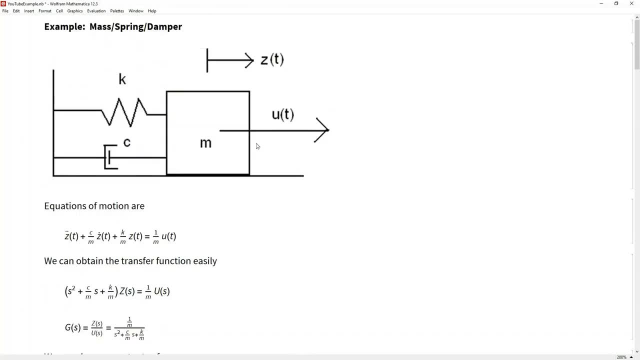 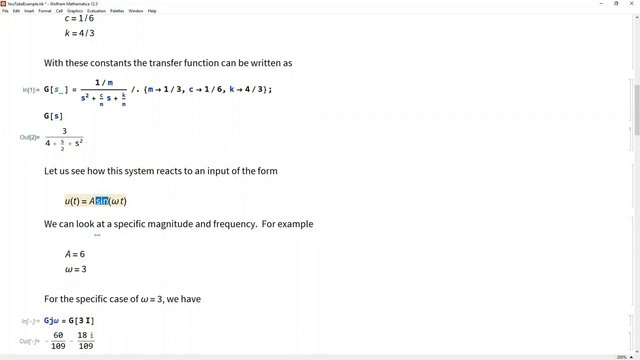 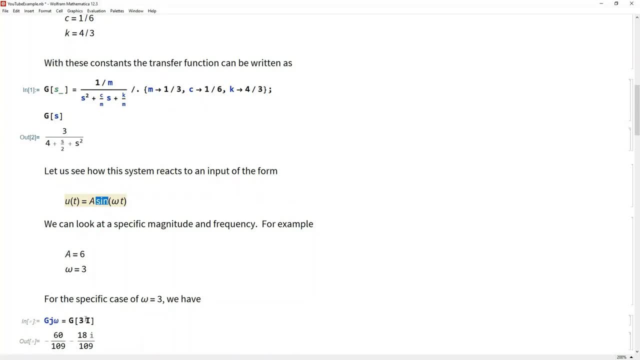 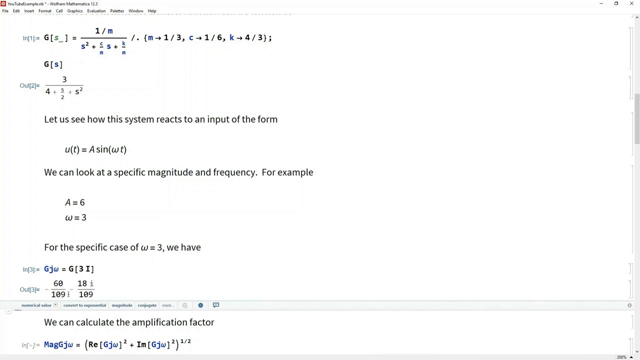 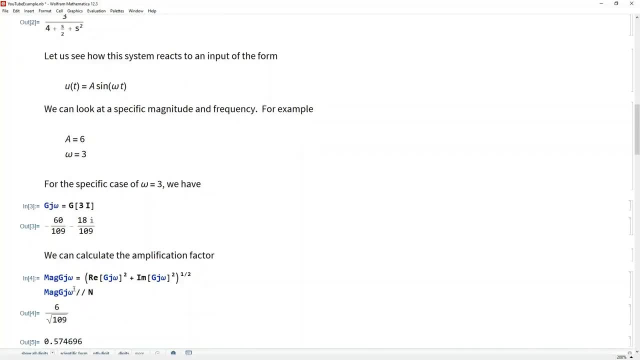 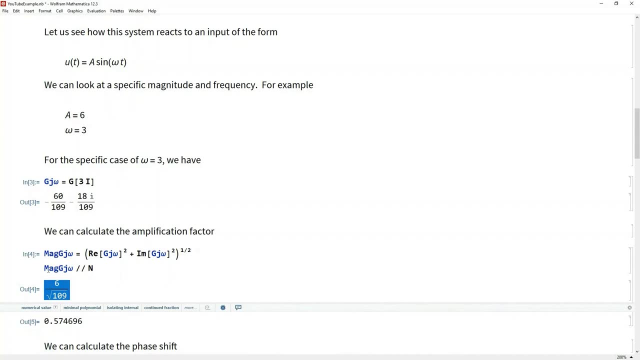 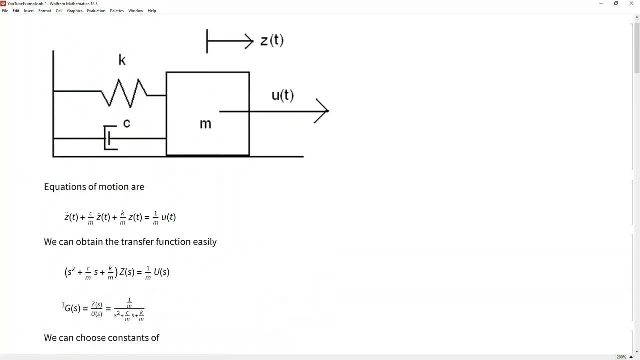 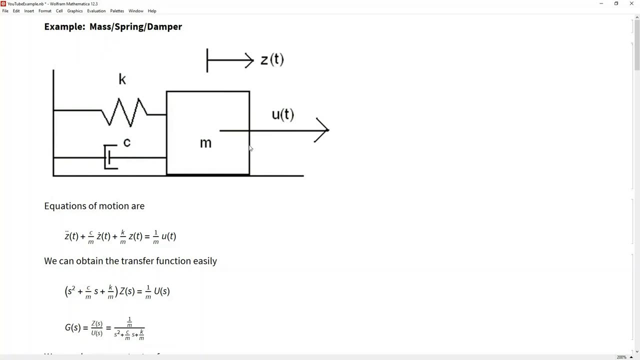 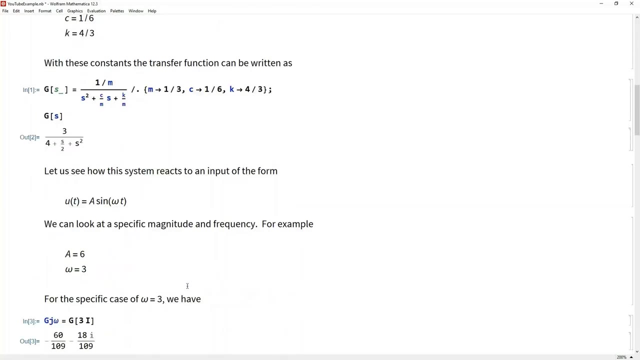 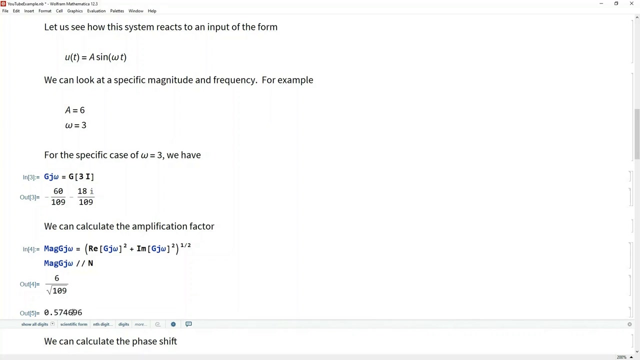 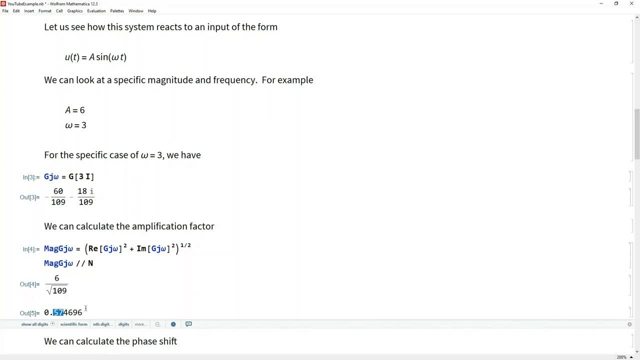 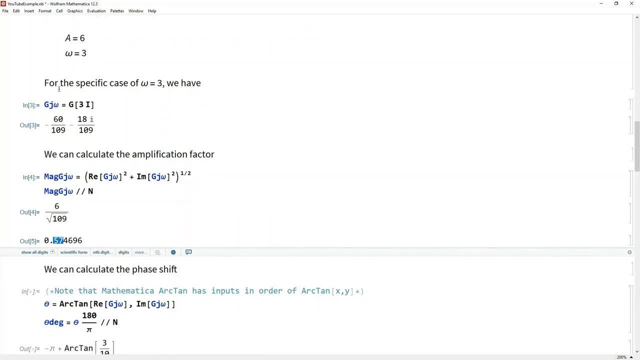 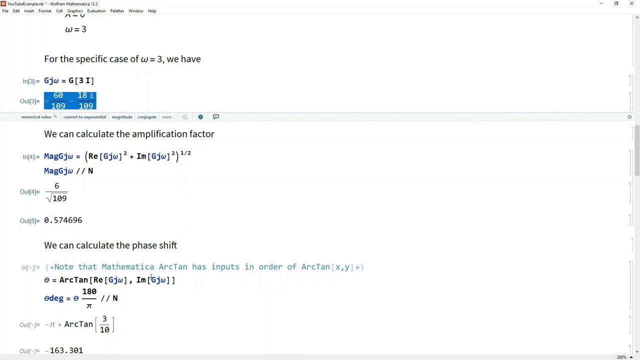 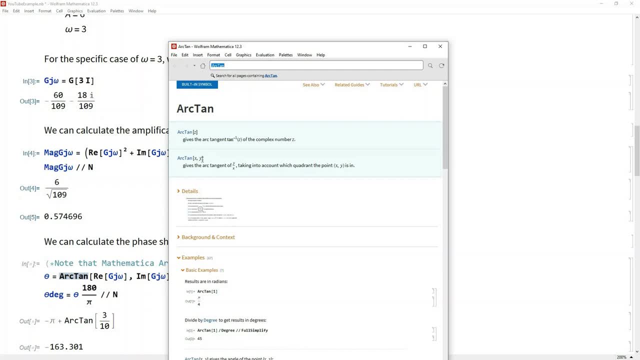 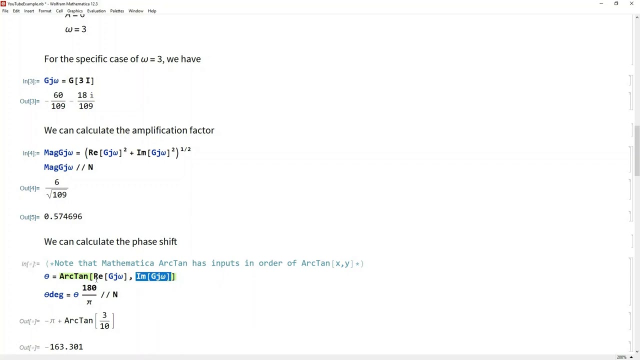 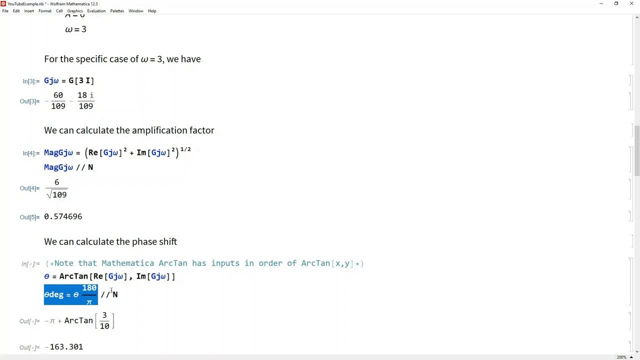 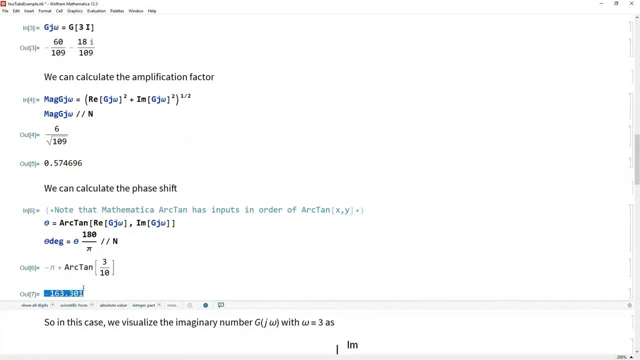 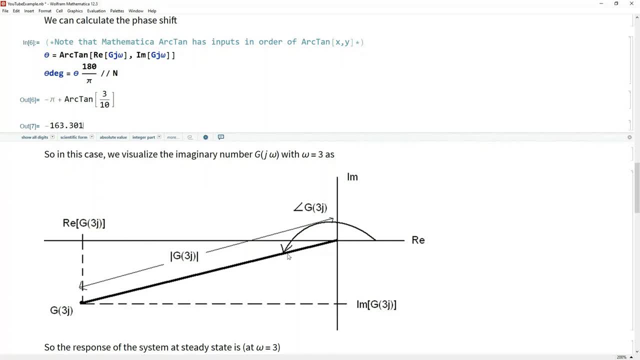 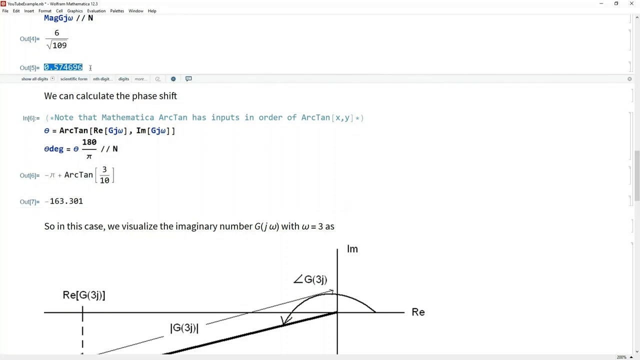 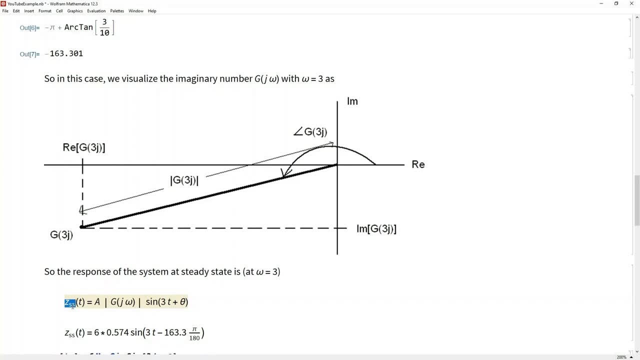 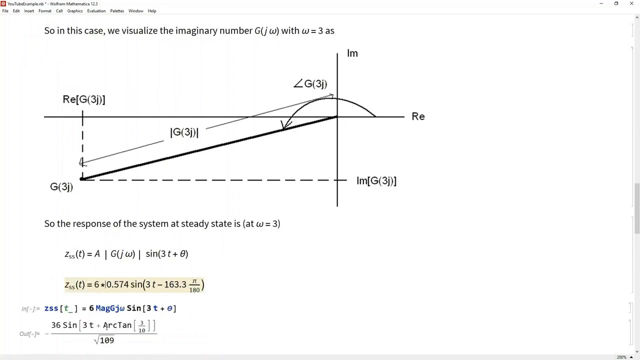 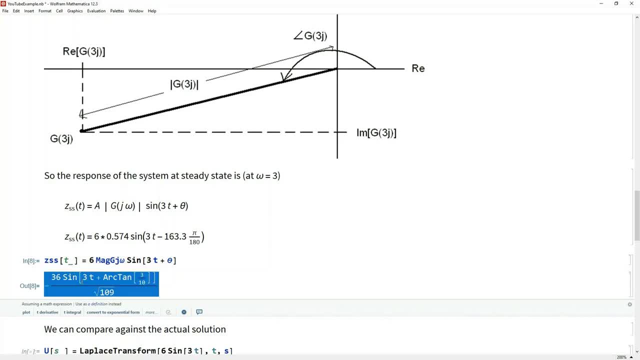 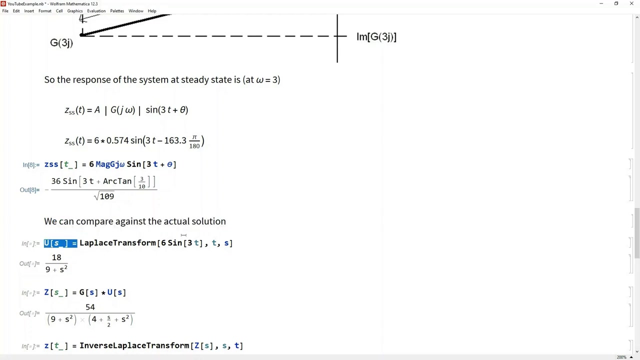 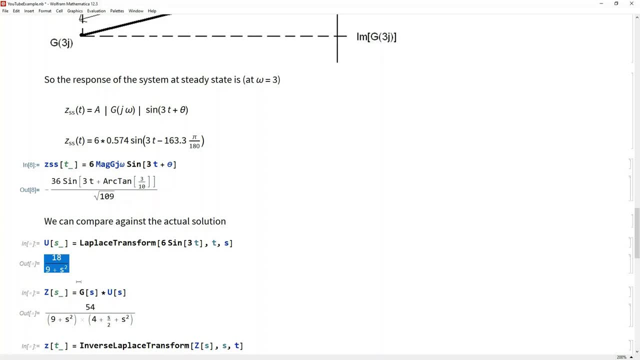 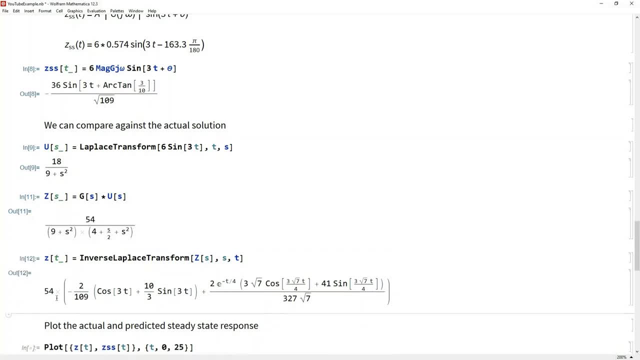 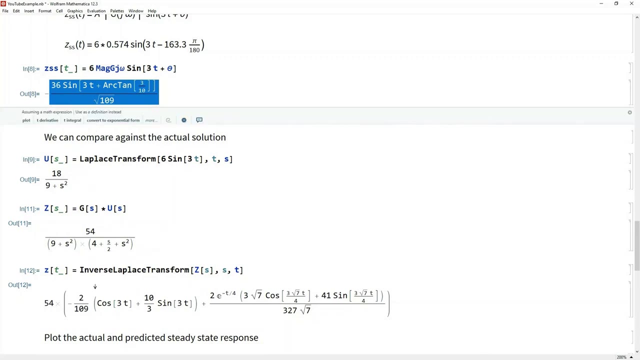 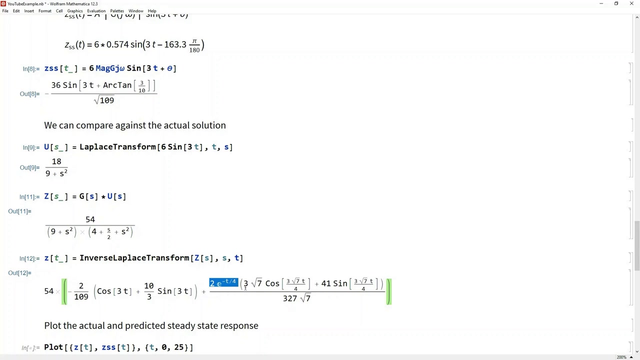 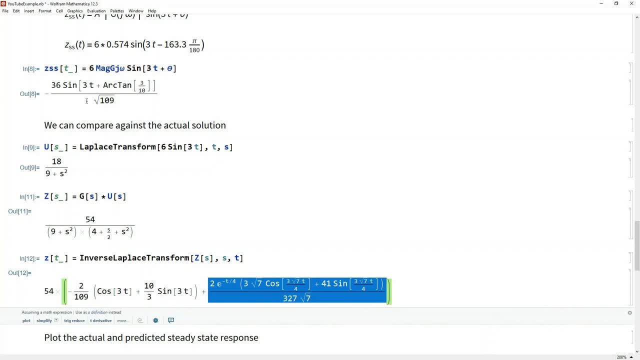 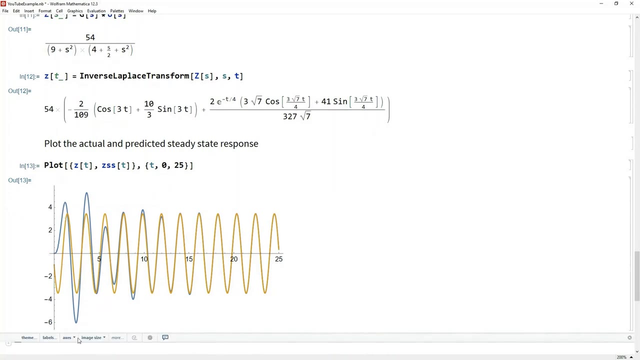 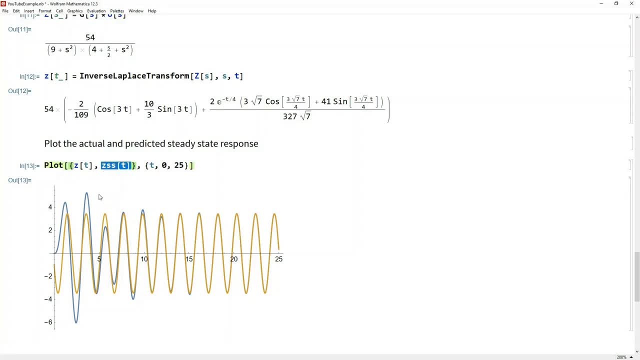 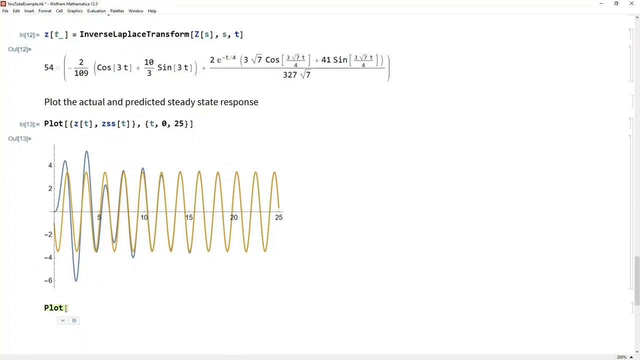 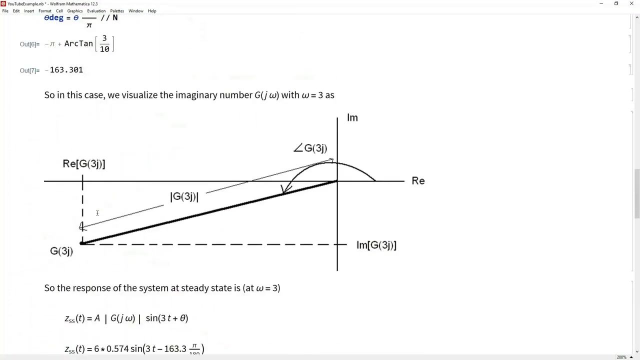 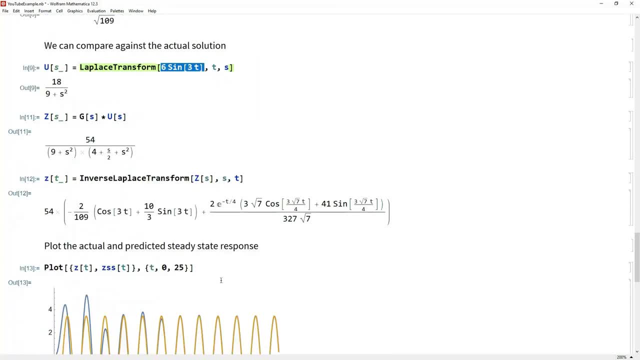 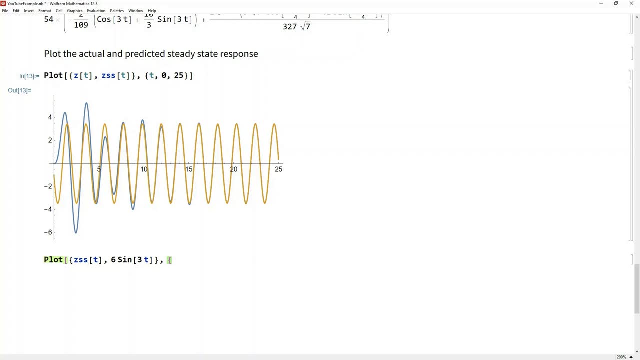 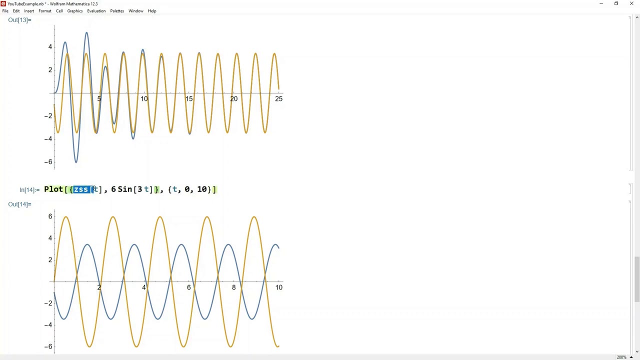 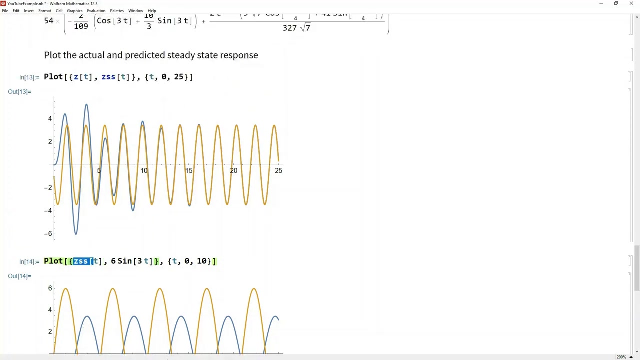 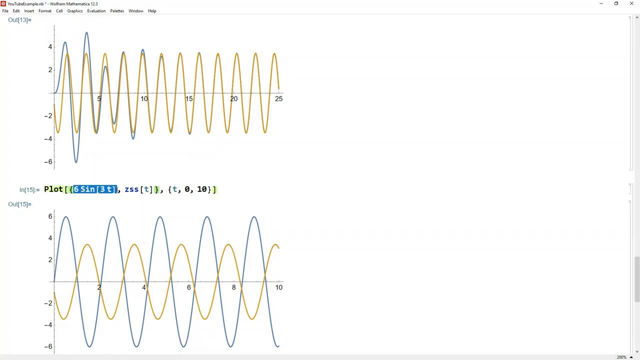 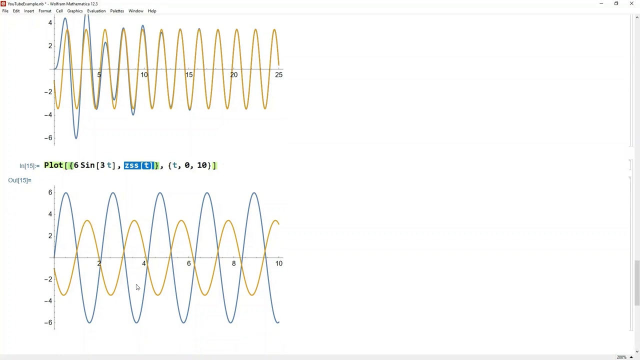 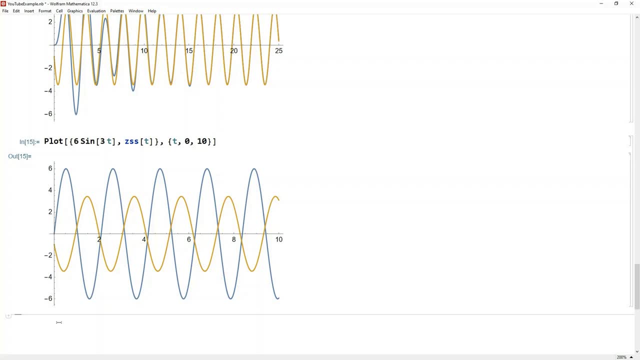 to the frequency response of the system. I just wanted to give a little bit of an introduction today and lay some of the mathematical foundations of this concept. The natural next question that I'm sure people are asking right now is: you know? this example used a very specific angular 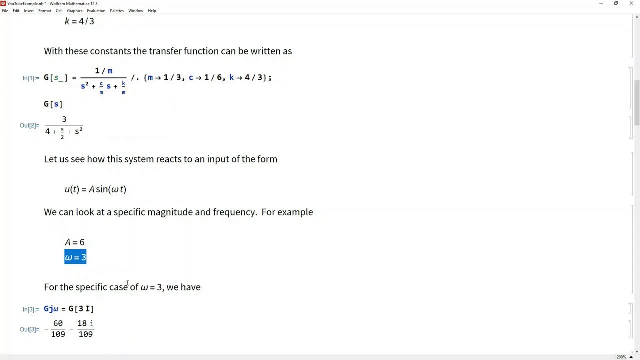 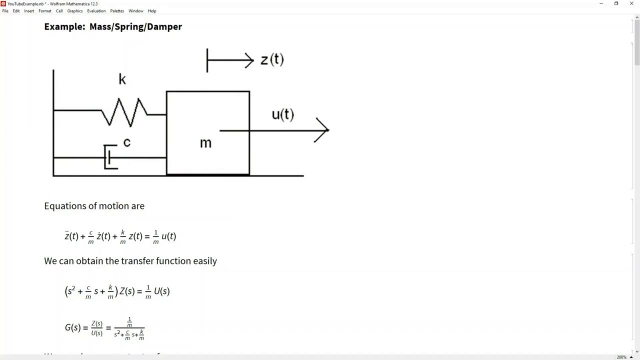 frequency of three. Why did we pick three? Why not five or 30 or 300?? How does this system respond and how does it change if the angular frequency were to change right? That's the logical next step, And in fact that is what we're going to talk about in several of our next videos, And 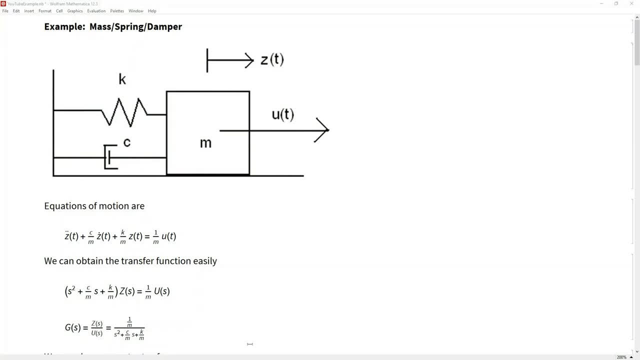 that's going to introduce things like Bode plots, resonant frequencies and a lot of other interesting analysis that we can do on this linear system. All right, so let's take a moment to summarize- And here's the funny thing, right, We've been talking for about an hour and we can summarize.